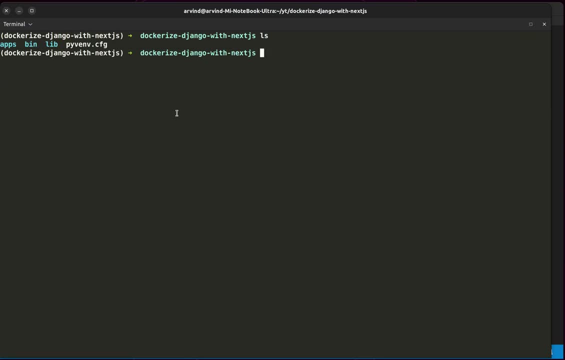 source. So yeah, and now what I'll do is I'll initialize poetry. I'll be using poetry. you can use whatever you want. yeah, so I initialize poetry. so poetry ad. I'll be using Django version. 3.2 comma less than 3.3. yeah, I'll be using the Django version between 3. 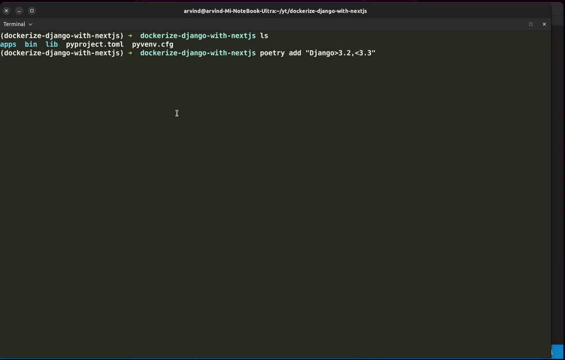 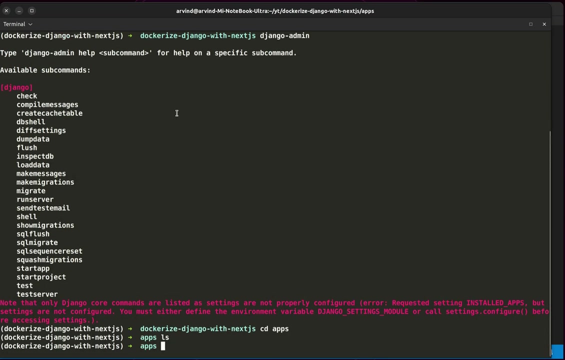 and the 3.2 and 3.3, because the Django version 3.2 is the LTS, so I'll be using that. yeah, so once it's installed I'll have Django dash admin. yeah, so I'll cd into apps and hit LS. there's nothing, so over here I'll create Django admin. 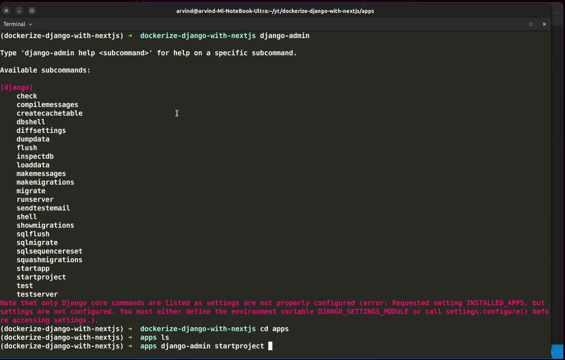 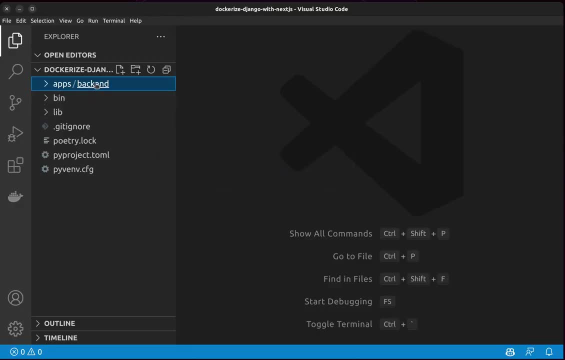 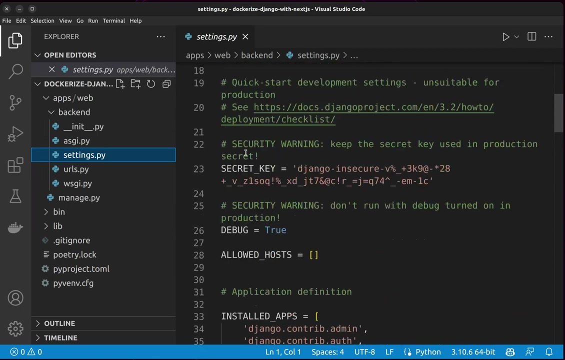 yeah, so I'll cd into apps and hit LS. there's nothing, so over here I'll create start, call it back end. yeah, and now, apps back end. so I'll rename this to web as of now. so, yeah, and now. this will be my Django project. and now. 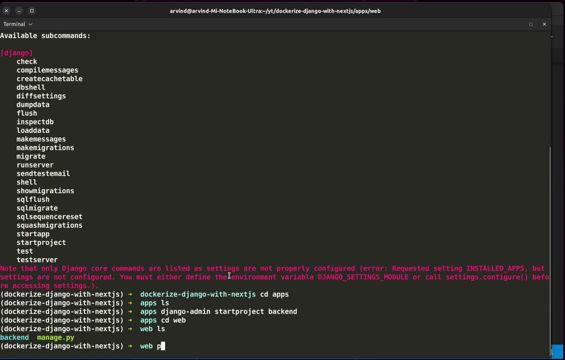 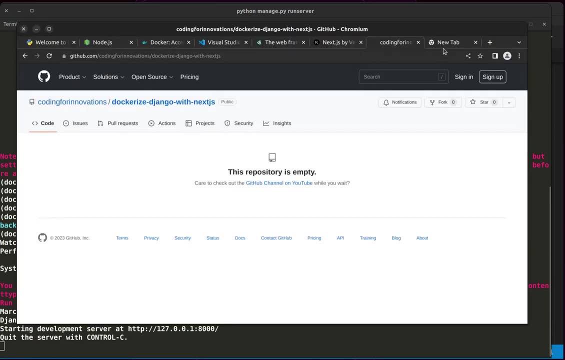 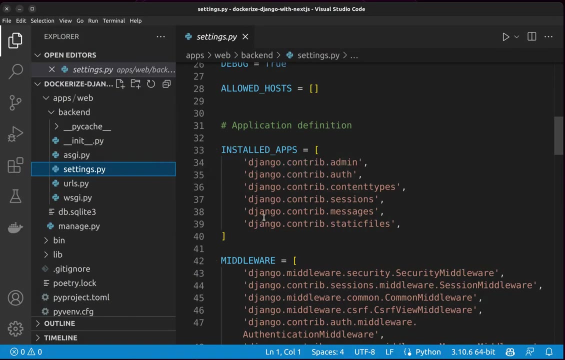 I'll do. I'll create Django hamster if I cd into web and now, if I run server and now I got a localhost. yeah, I see my Django app is perfectly working and now? now what I need to do is I need to configure various stuffs for it to use. 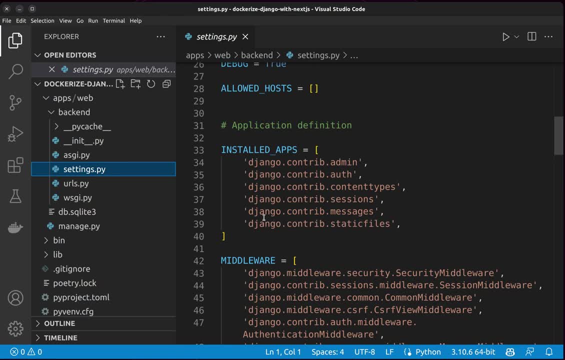 now what I need to do is I need to configure various stuffs for it to use docker, so. so first thing is I need to setup here and then we have any program. I will create a scripts folder inside web, new folder s-c-r-i-p-t-s. it will be a scripts. 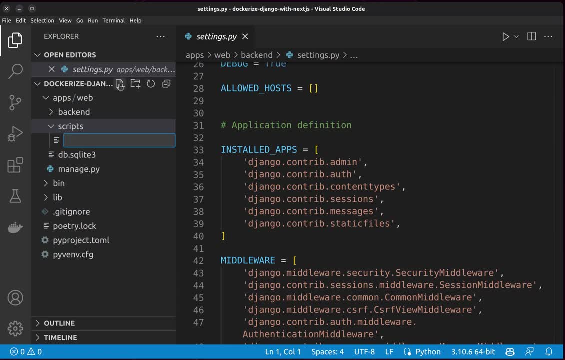 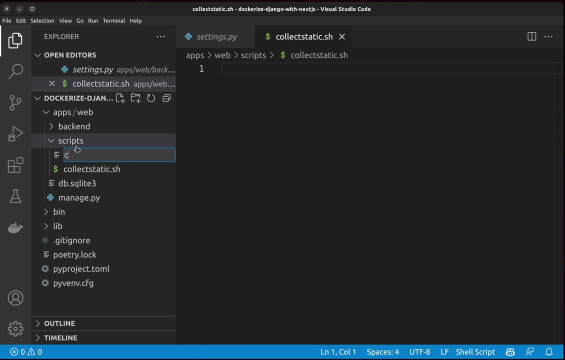 and then I will create a new file and that will be the file will be collect, staticsh. that will be one file and then the other file will be create: Super User, dot sh. and the other file will be Entry Point, dot sh. and the other file will be Migrations, dot sh. 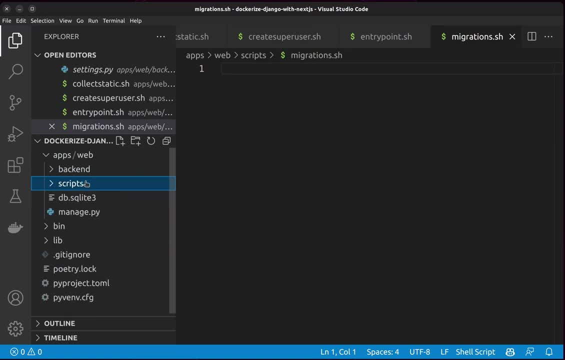 So These are the two files that I will create. the four files will be using and I'll create another folder inside apps, known as docker. so inside docker it will be a new folder web and inside web it will have docker file. yeah, and now inside docker- new folder www, it will have a. 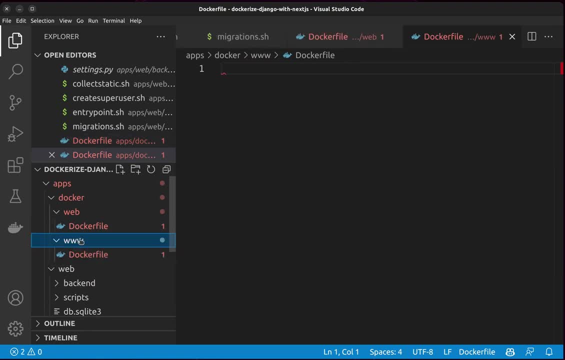 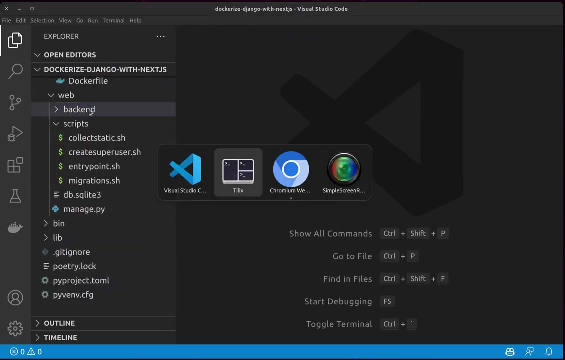 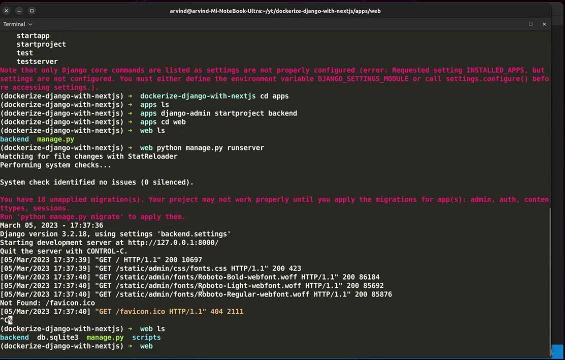 docker file. yeah, and now inside docker, another folder: nginx. so nginx will have another docker file and then its config file will come here. so, yeah, so let me go to the terminal and I'll. now what I do is I'll start another app. start app. I'll call it custom commands, because we need to run to create a super user. yeah. 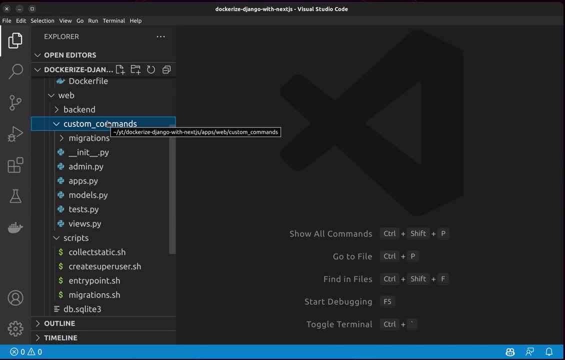 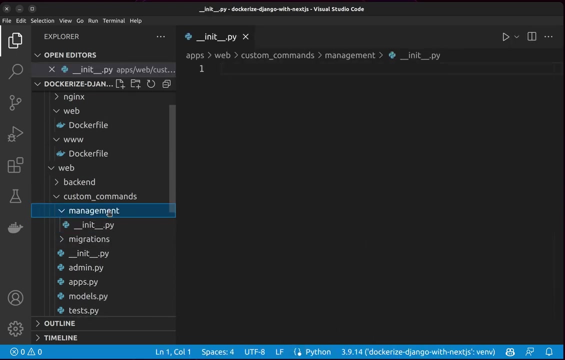 so this file, this is just to run certain commands, yeah, to run certain commands, which will create the super user. so hit manage den T to be management in it, that way to make it as module and new folder. that will be commands command. so inside commands, that will be another. 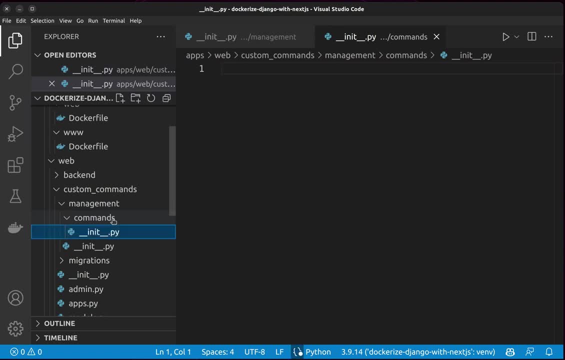 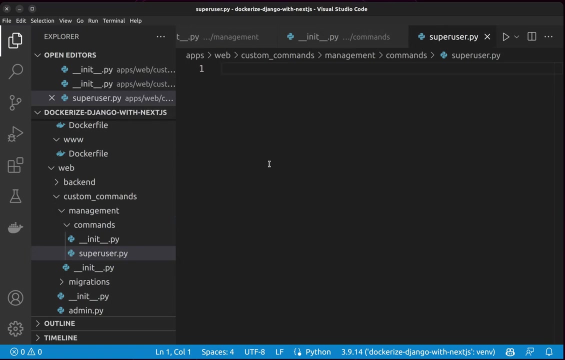 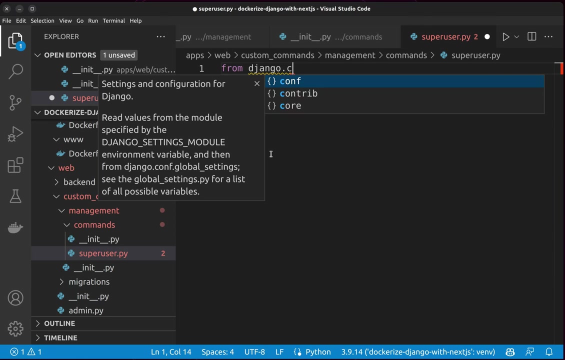 OK, initpy, and inside commands it will be superuserpy. so now we are going to create a custom command to create a super user. so yeah, from the anchor dot it will be core dot, management dot, base, import, base command. yeah, and it will be command error okay. 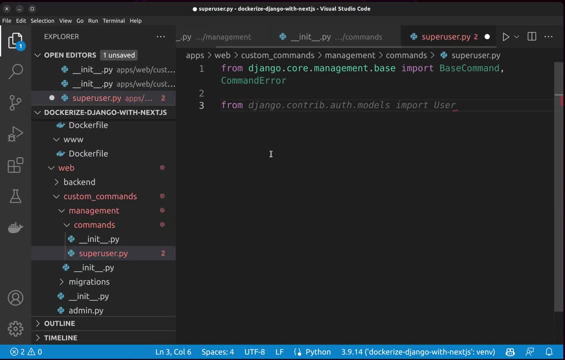 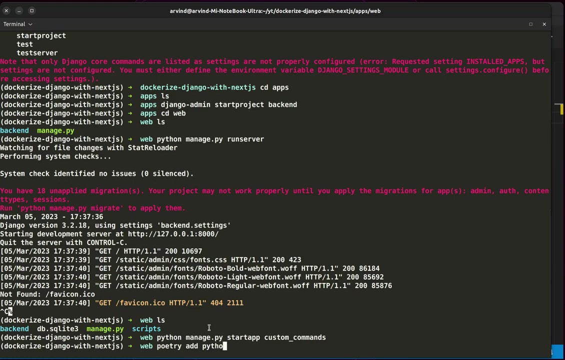 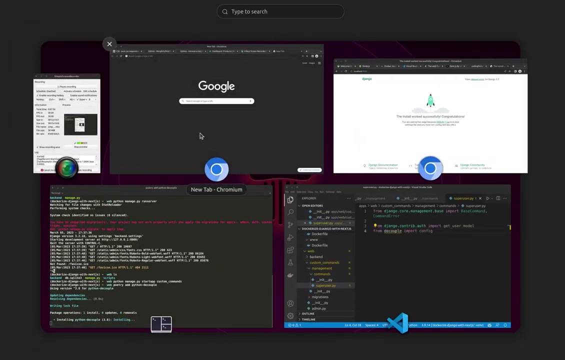 so, and now from django: no, from contractauth, it will be import. yeah, it will be import. and then, and then from decouple c o u import config. so we haven't installed decouple. so poetry add: it will be python decouple. yeah, so, yeah, let it add: yeah, so and now? 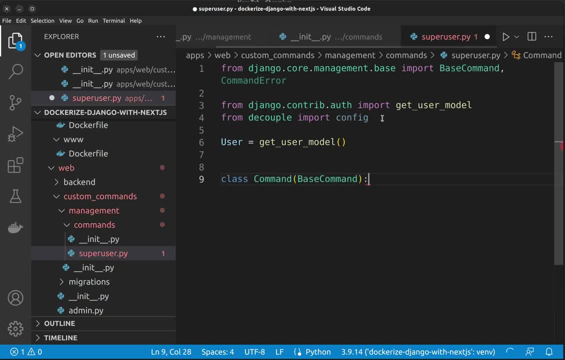 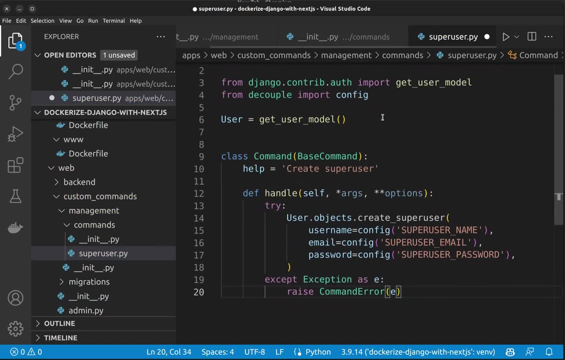 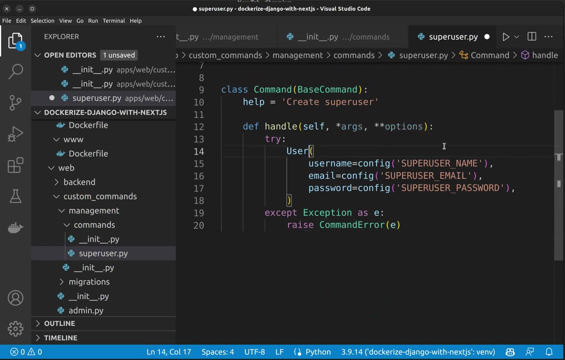 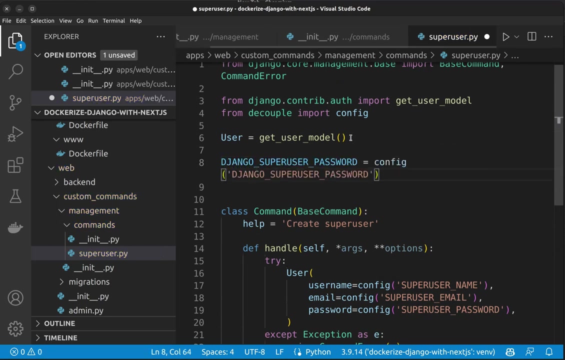 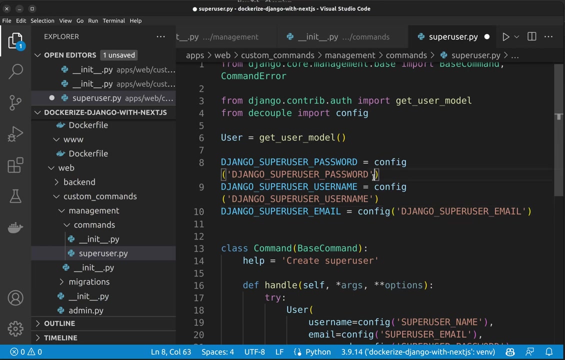 user is equal to get user model. and now class base command. yeah, base command. okay, so it is helping me. i'm not going to do like this. yeah, django super user. yeah, django super user email. okay, so this is actually correct. so i'll cast all those things to string. 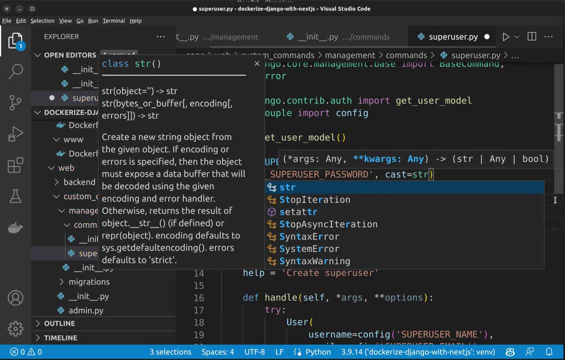 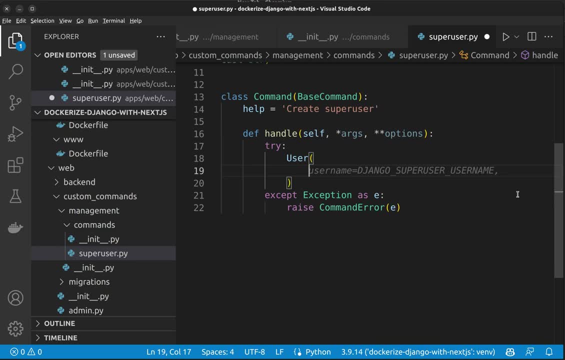 so there is a inbuilt function called cast yeah, which will yeah, so this looks perfect. so it will be user yeah, so it will be email email is django super user email username, and what i'll do is user dot set password, yeah, and then this is user is equal to yeah, and now user dot is super user is staff. 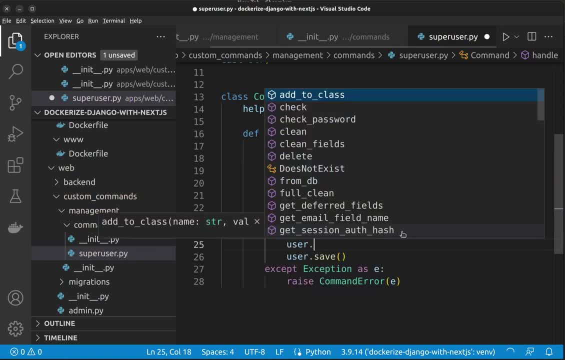 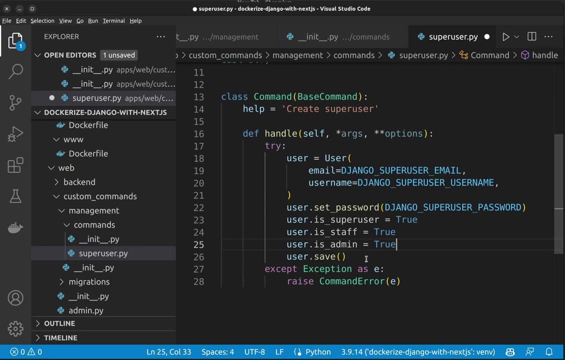 and then i'll do: even is admin, yeah, and then i'll do: even is admin. and then i'll do: even is admin is underscore admin is true, and now i'll hit save. and now is underscore admin is true, and now i'll hit save. and now. 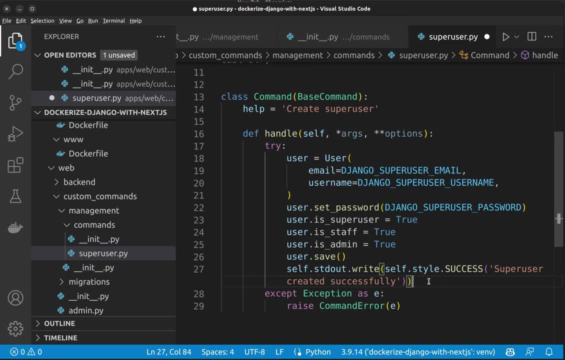 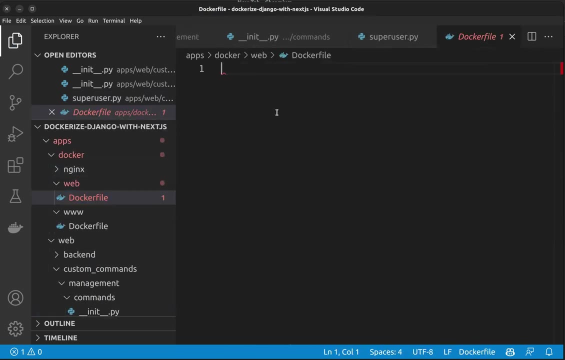 yeah, super user created successfully. so we have created one part of this. so the super user command will run. and now, yeah, and now let's create a docker file. boom it's for web. yeah, and now, let's create a docker file. boom it's for web. and yeah, let's. so it will be from. it will be python. since i'm going to use three point. 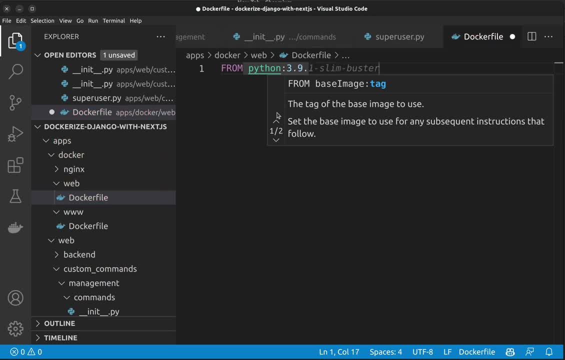 three point, oops, nine point. thirteen: hyphen slim, it's just slim, and now i'll hit run. so i'll make a python 3, hyphen m: it will be v e n v inside otp and then v e n v. okay, and now what i'll do is i'll create cmd. 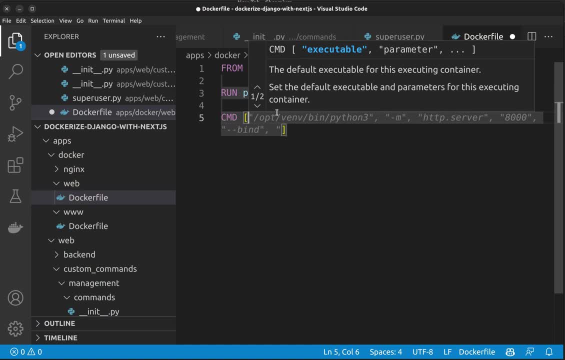 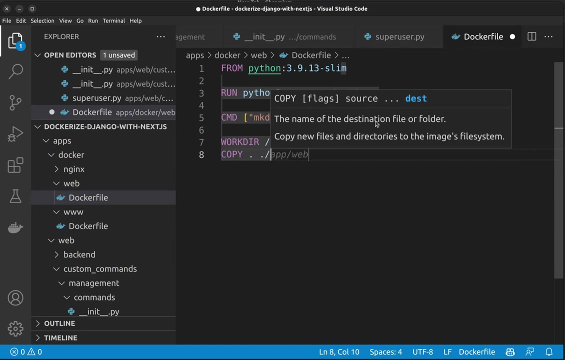 it will be. it will be in double quotes. make the: yeah, it's gonna be app slash web. okay, so, and now it will be working. the working: there is appweb and now it's going to be copy copy dot. no, no, it's copy dot slash, app slash web. 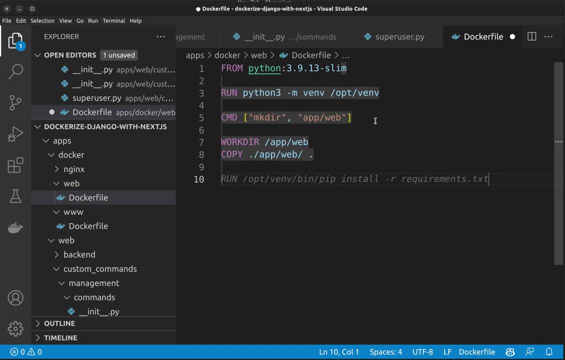 to dot: yeah. and now where it comes the important part. so we are going to run otp v e n v bin pip now. first we'll upgrade pip. yeah, so pip, yeah, so pip, install pip upgrade. and then you put comma: yeah, pip installed as our requirements. it will be instead of requirements, it will be: slash, app, slash web, slash requirementstxt. 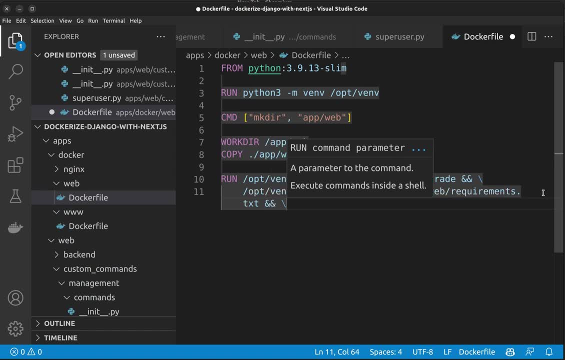 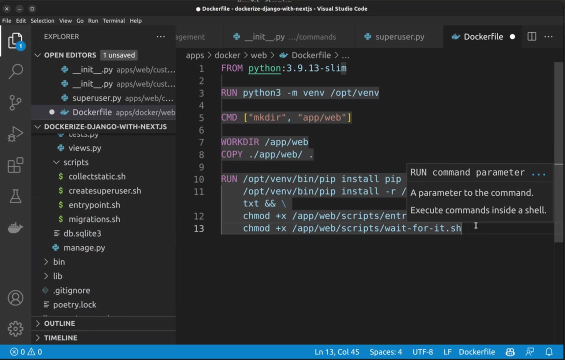 and you will run siamo and you will run. so yeah, so, whatever scripts we created here. so first one will be: instead of entry, collect static, and now cr, create superusersh. and now chamode plus x, it will be migrationssh. and now, instead of run server, it will be collect. 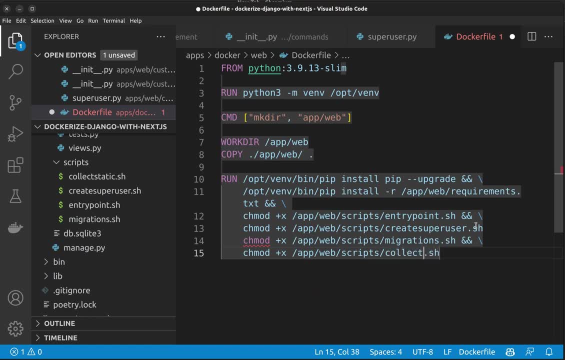 static, collect staticsh. and what are you gonna do? you are going to run, so bash is gonna be bash, and then we are going to run. first we run the migrations- yeah, it's gonna be migrations- and then we'll run the collect static. and after you run the collect static, we are going to run the create super user. 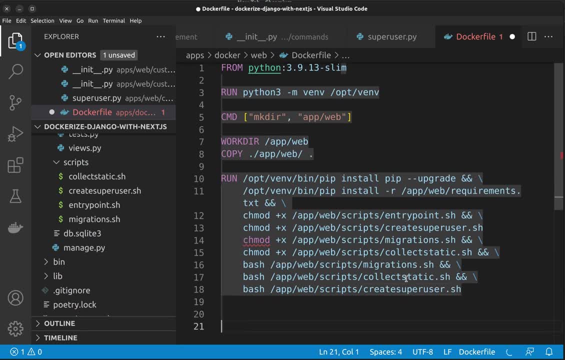 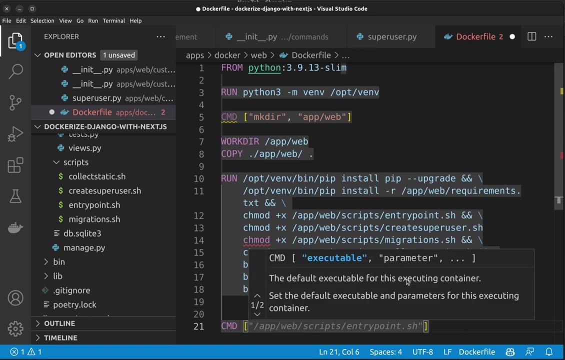 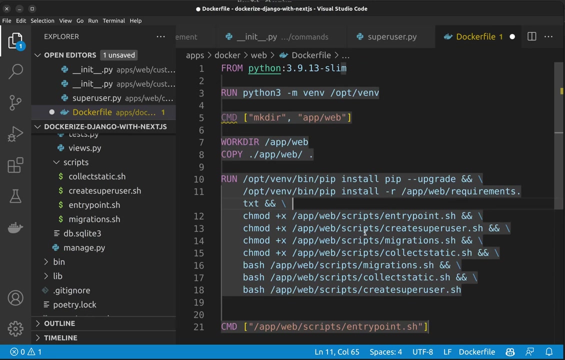 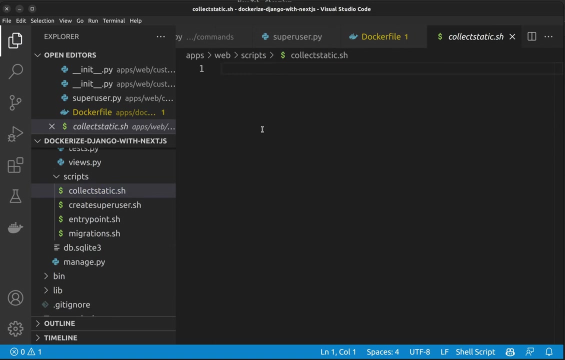 yeah, and at the last it will be a CMD. yeah, we are going to run. yeah, that one. so this is the it's pointing me out. yeah, so this is the docker file, and now we should fill all these things. so let's go to collect static dot sh for a second. 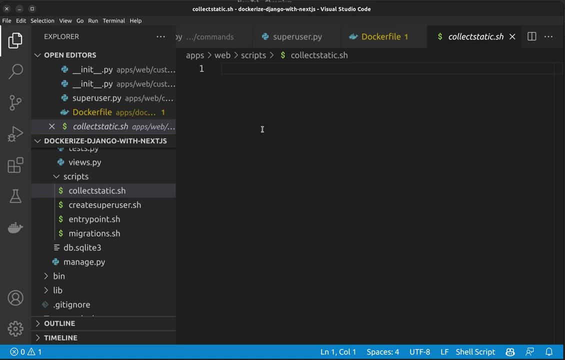 yeah, so it will be hash, call hash, and then it's a bang slash, it's going to be bin slash, bash. okay, so it's going to be OTP slash, VENV slash, bin slash, bin slash, hash. and then it's a bang slash, it's going to be bin slash, bash. okay, so it's going to be OTP slash, VENV slash bin. 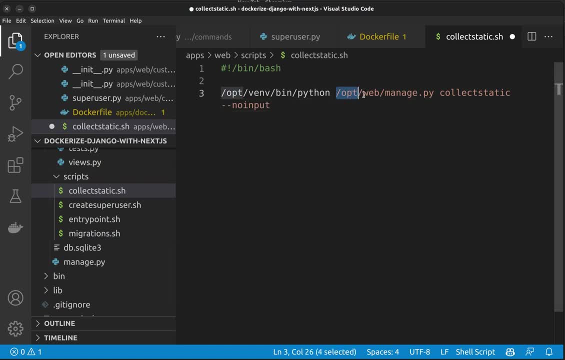 slash Python. it's gonna be managepy by. yeah, so yeah, so gonna be managepy- collect static. no input, CL. yeah, clear, okay. so this is going to be for collect static. for create super user is going to be managepy- superuserpy. you don't need to give anything over here, and now let's go to migrations. 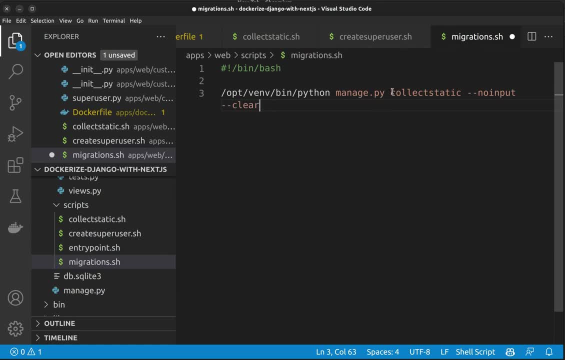 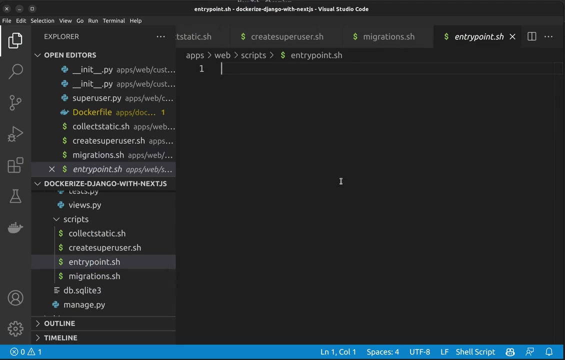 migrations is going to be managepy. first we'll make, make, make migrations and then no input, and then migrate, no input. okay, so all these things are working perfectly, and now let's go to the entry pointsh. so that is the very, very important file. so it's. 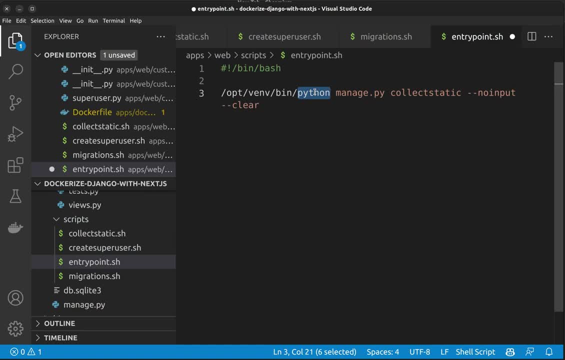 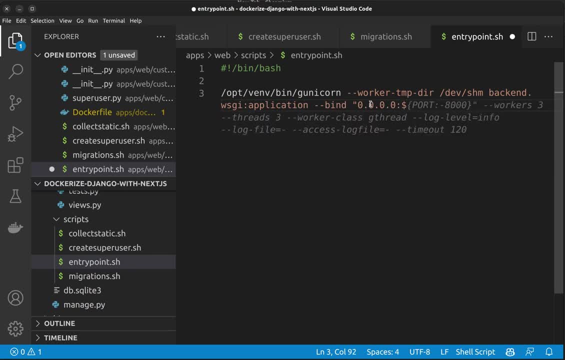 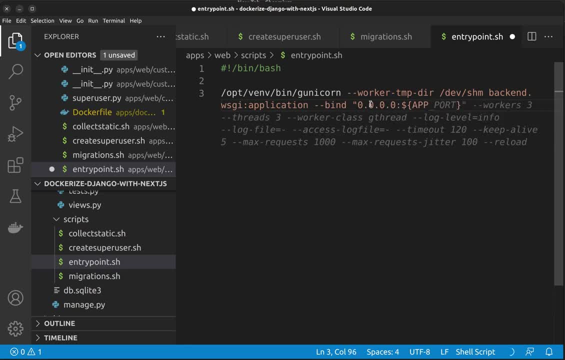 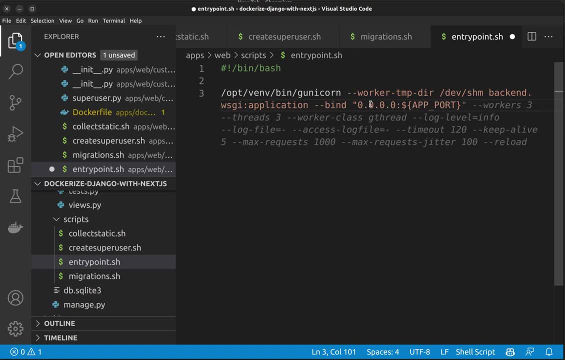 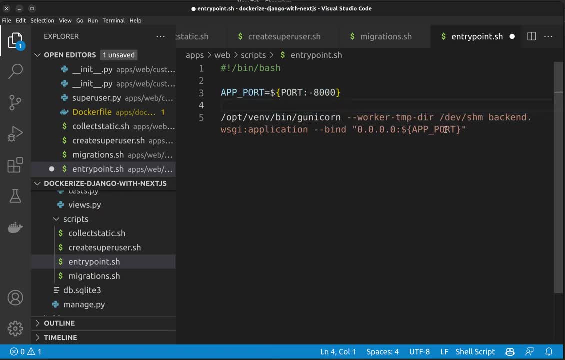 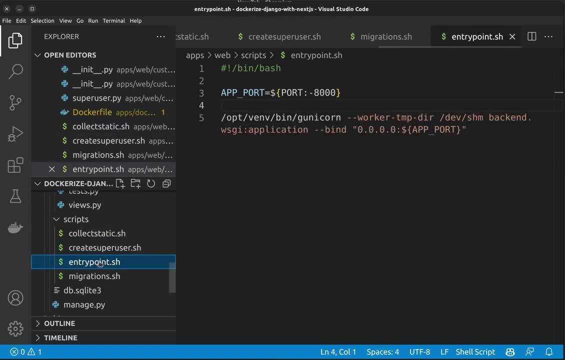 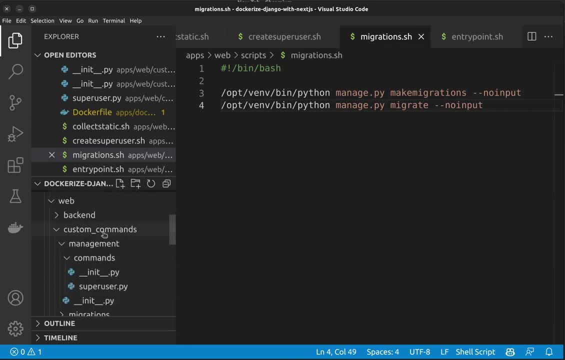 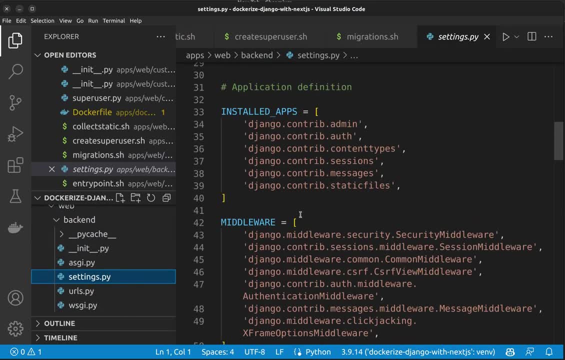 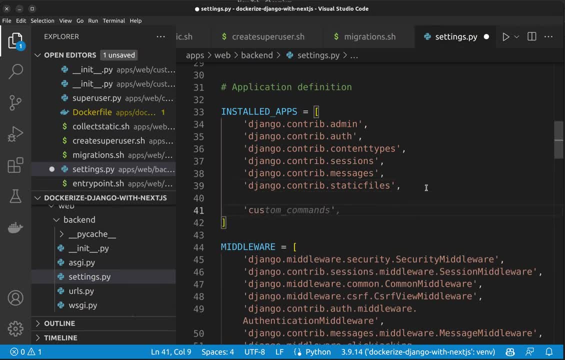 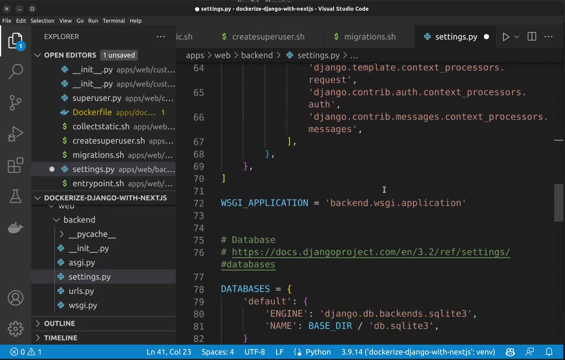 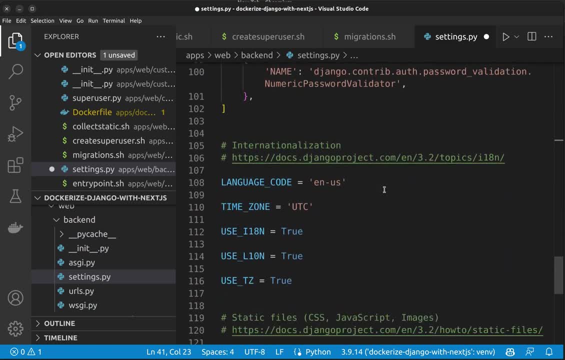 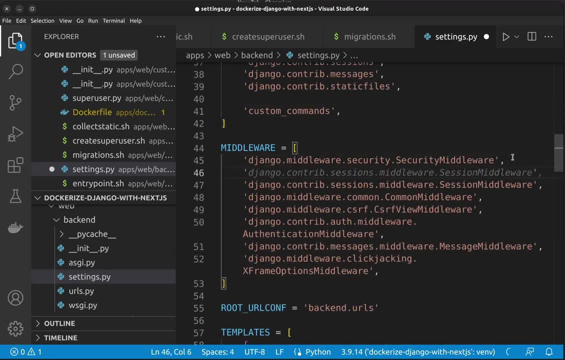 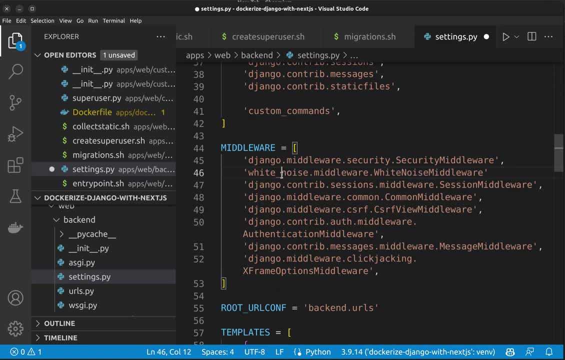 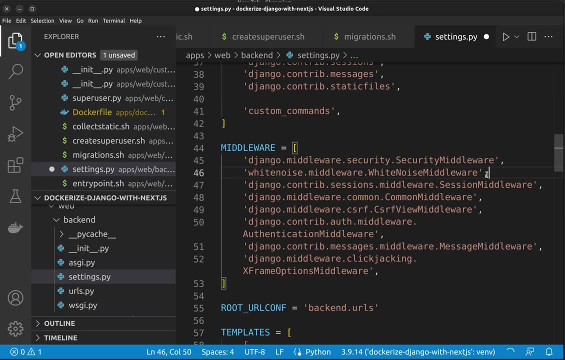 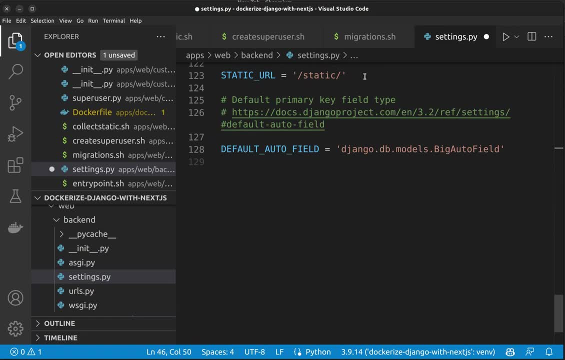 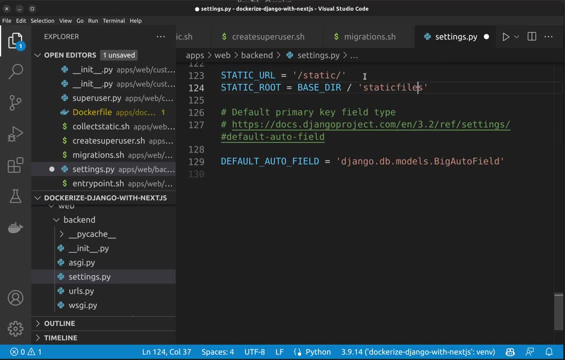 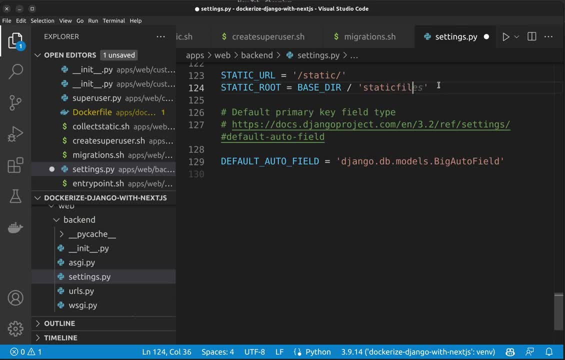 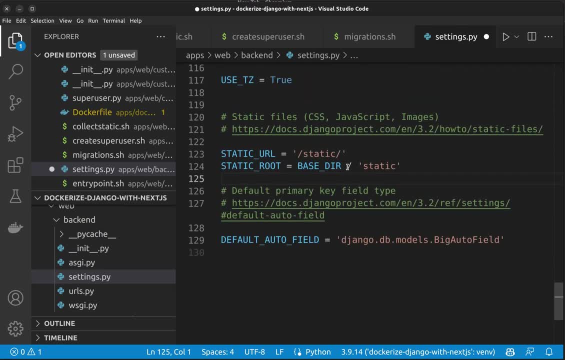 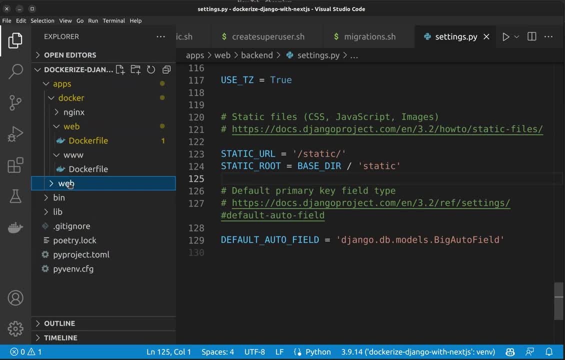 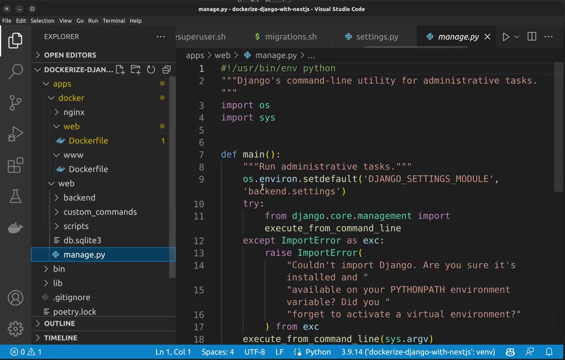 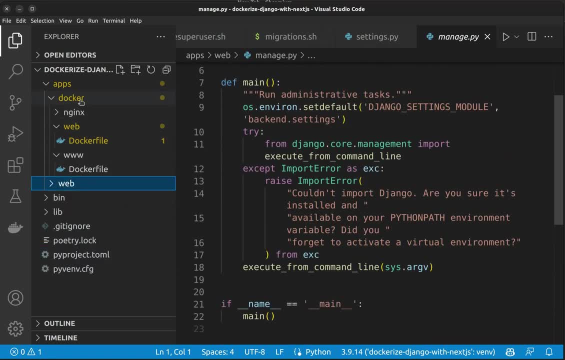 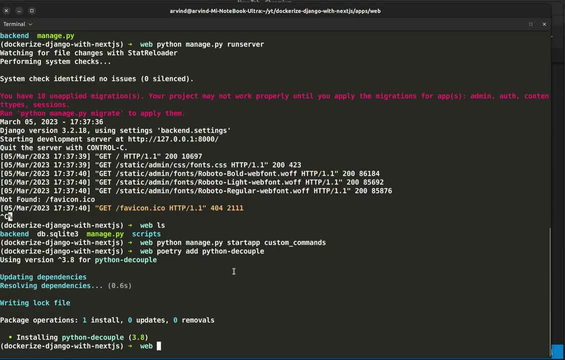 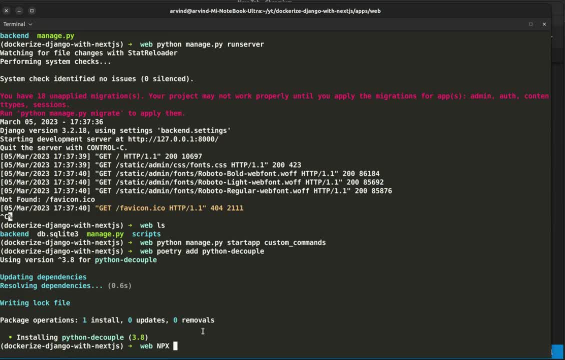 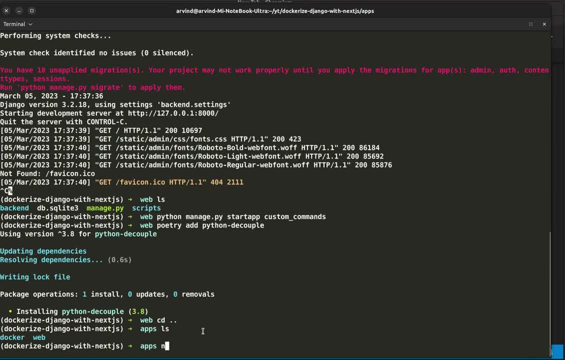 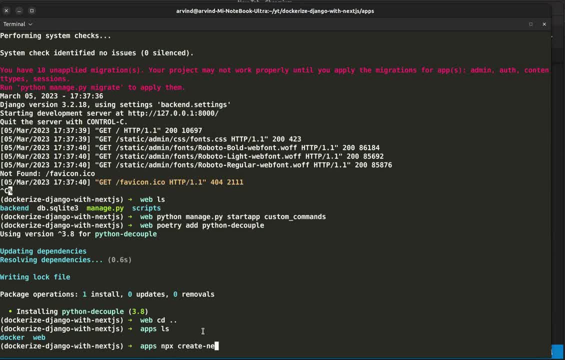 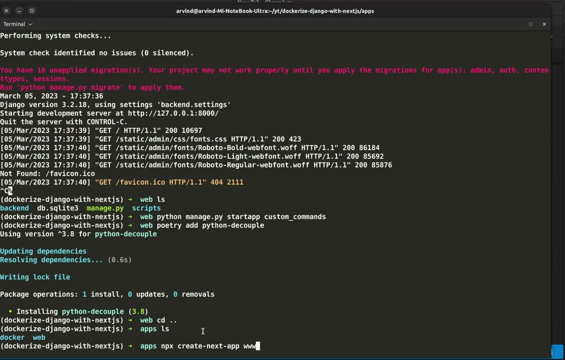 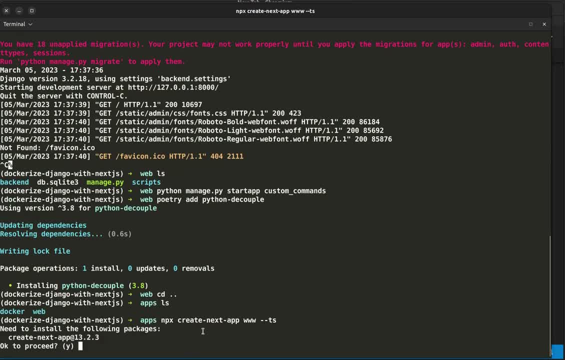 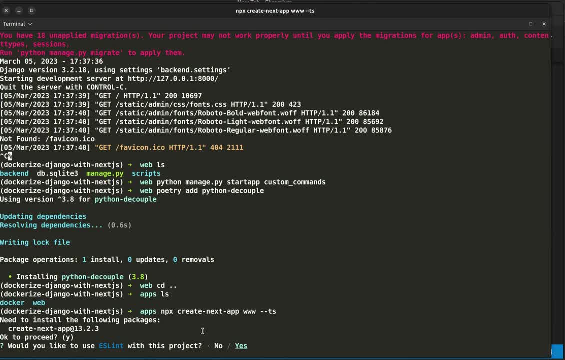 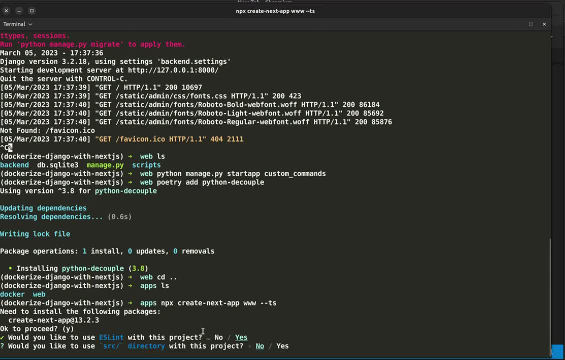 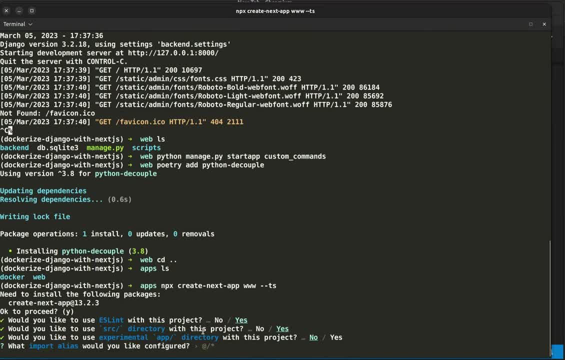 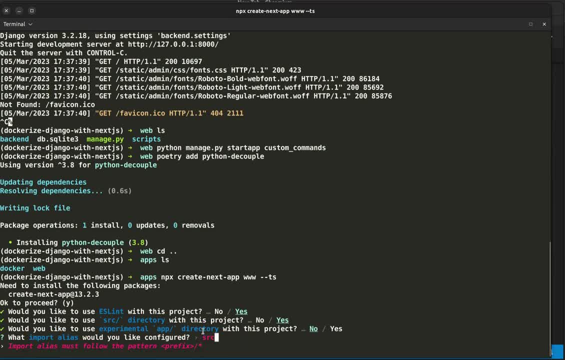 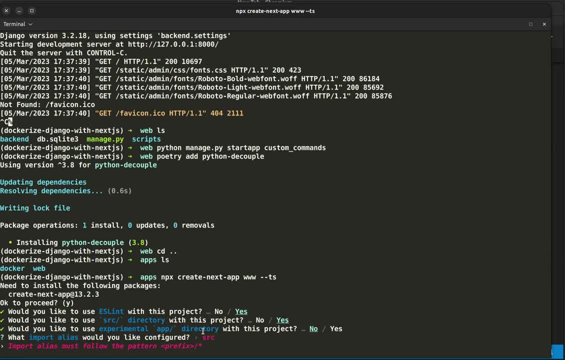 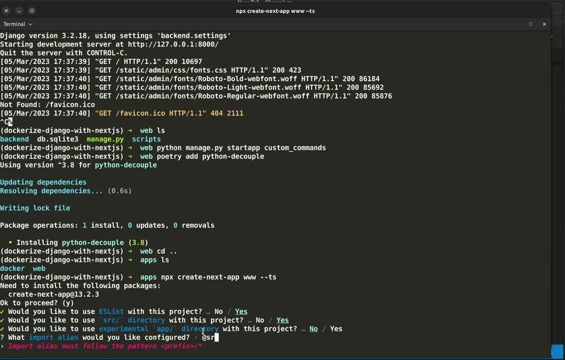 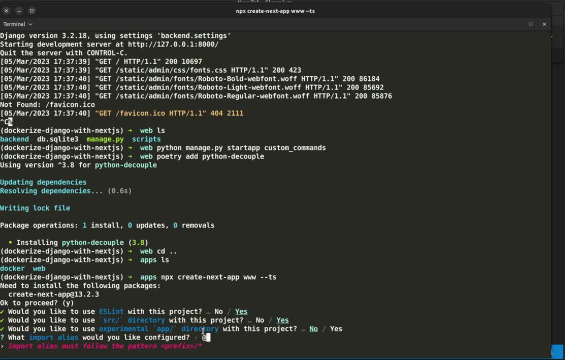 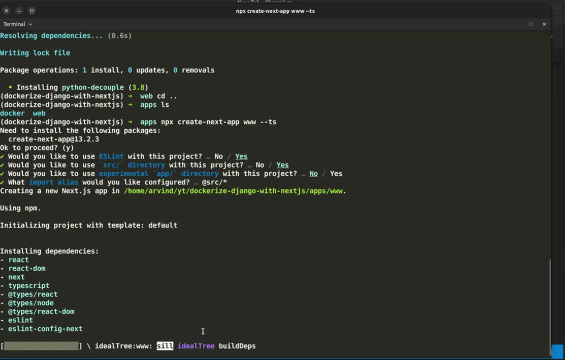 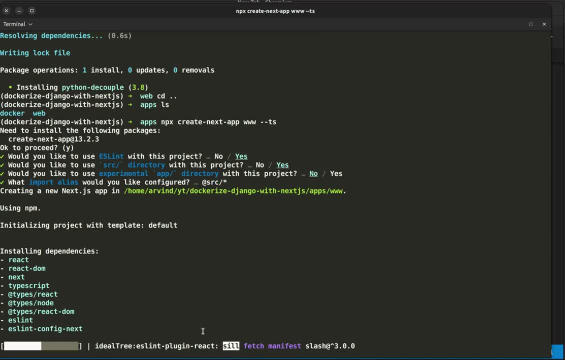 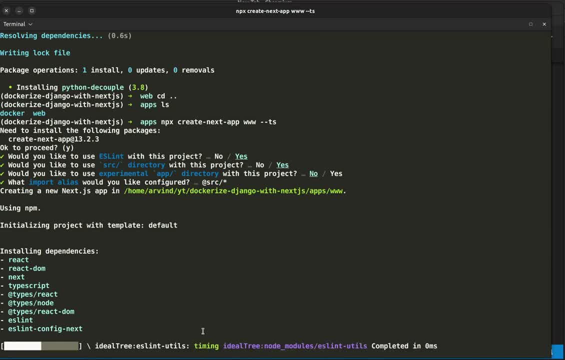 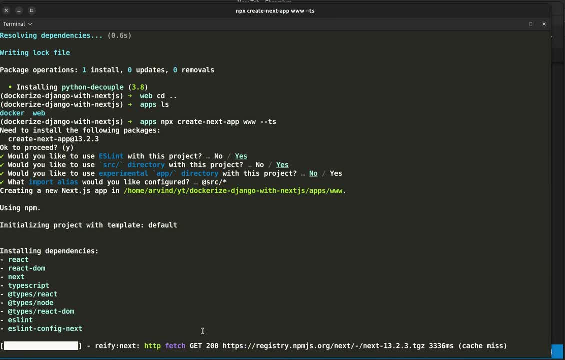 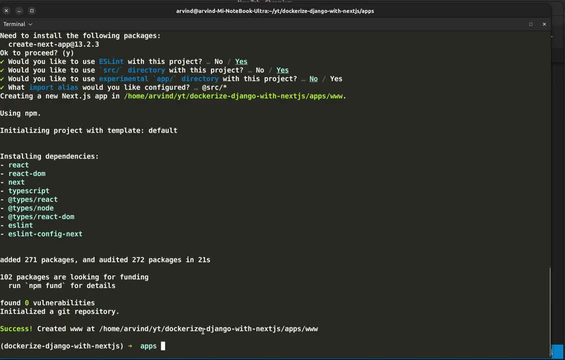 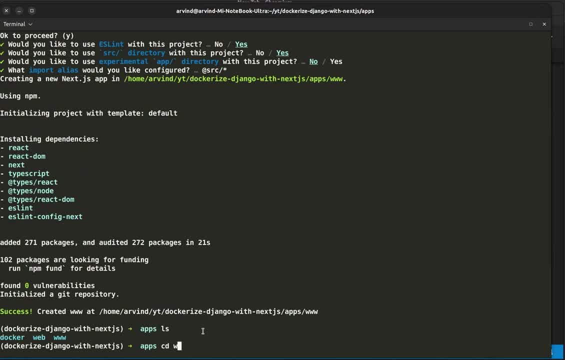 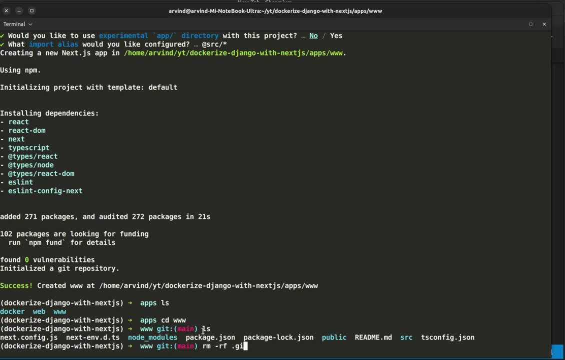 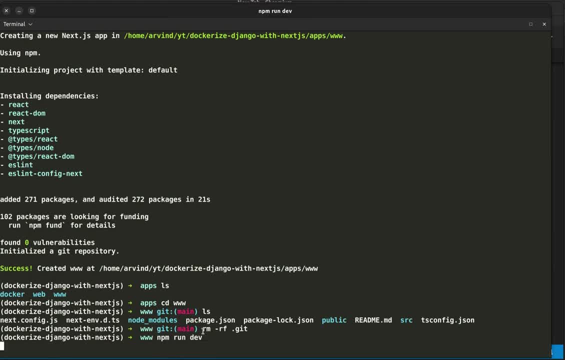 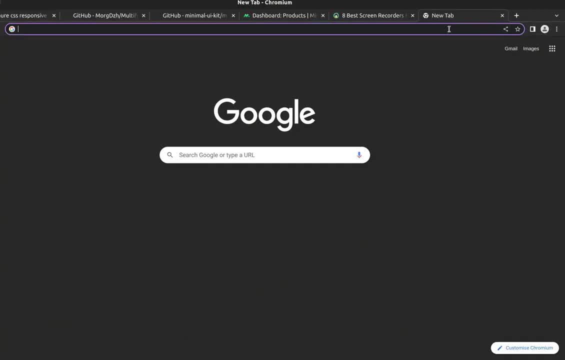 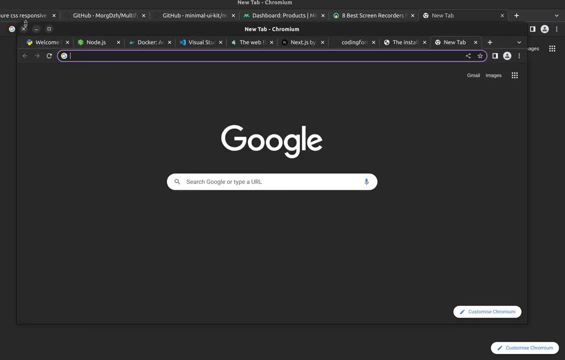 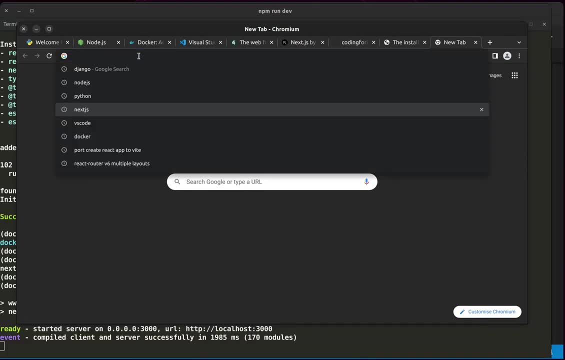 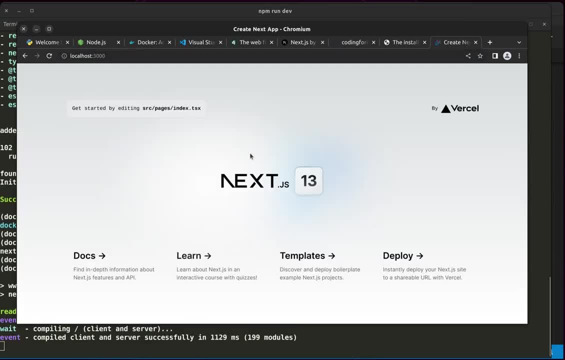 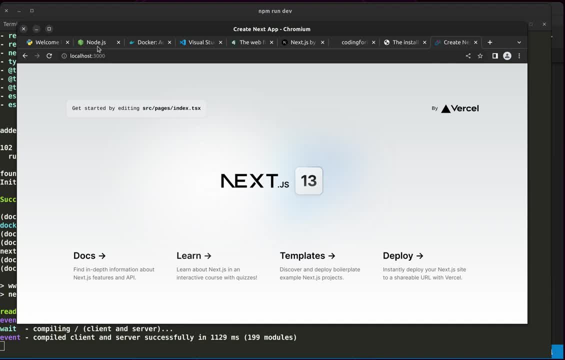 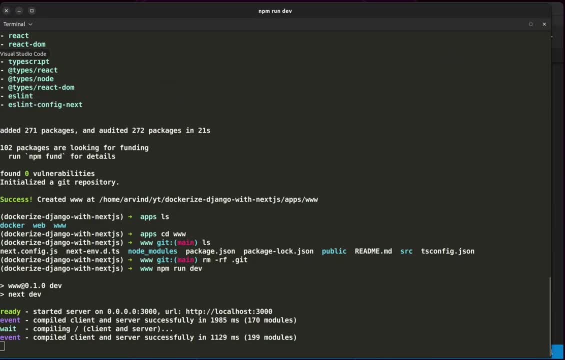 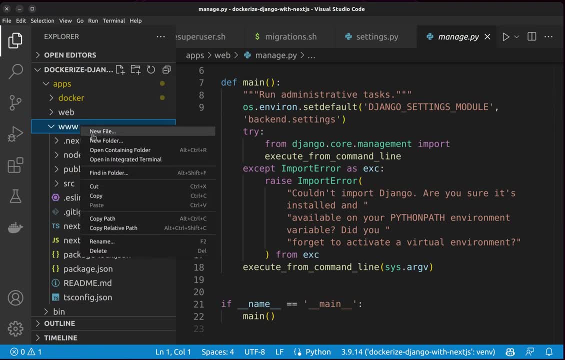 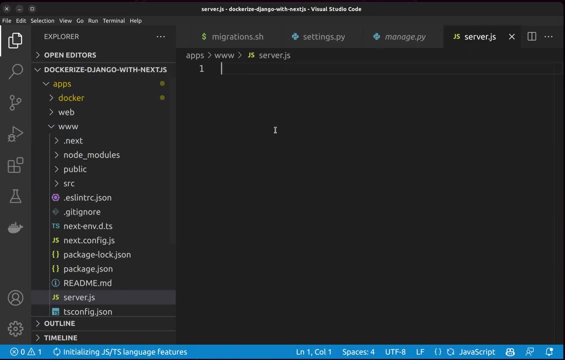 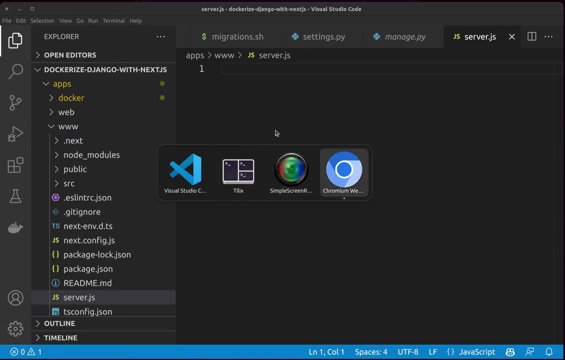 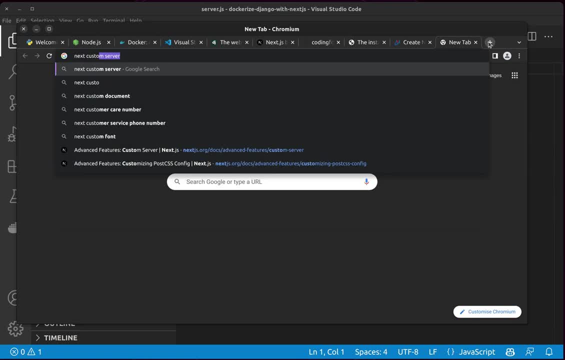 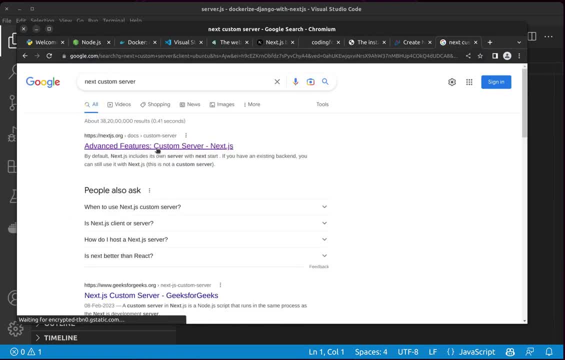 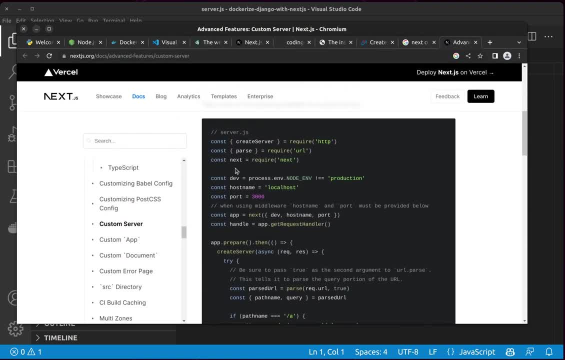 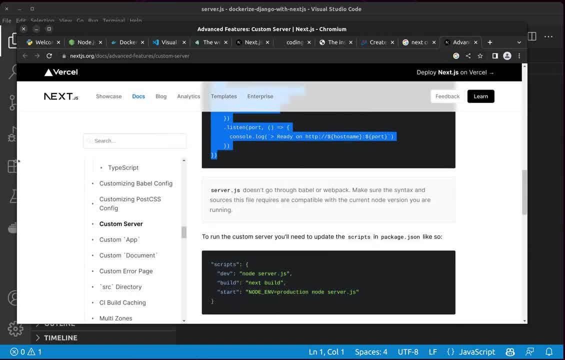 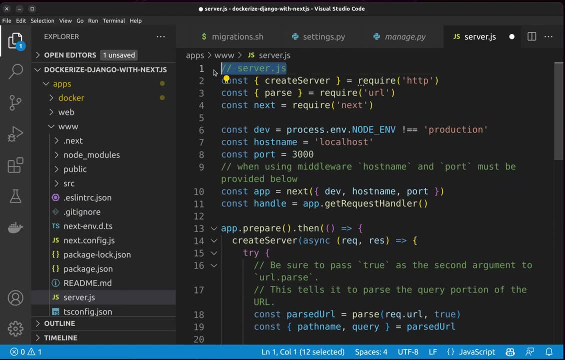 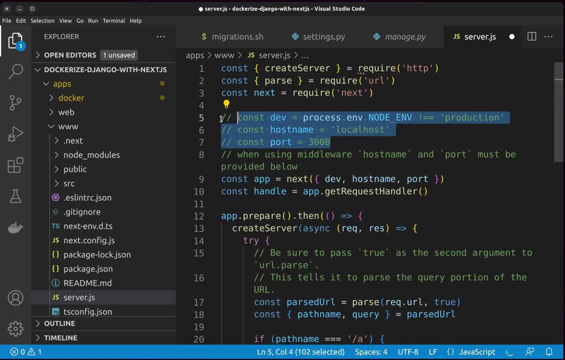 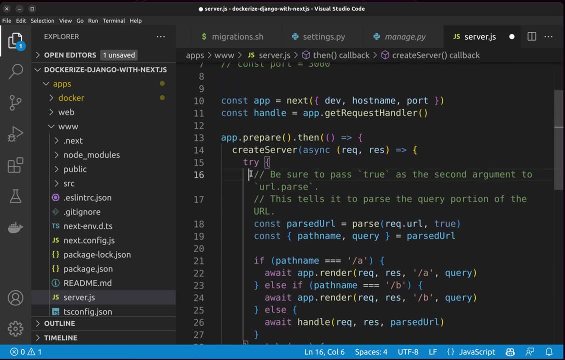 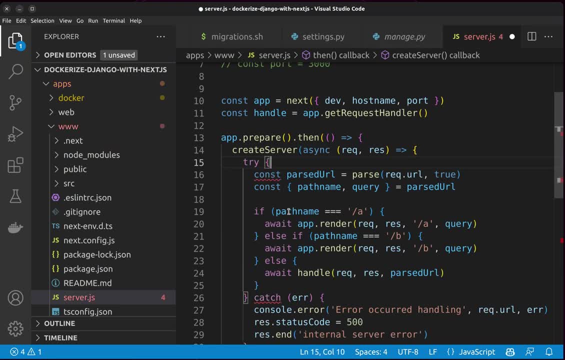 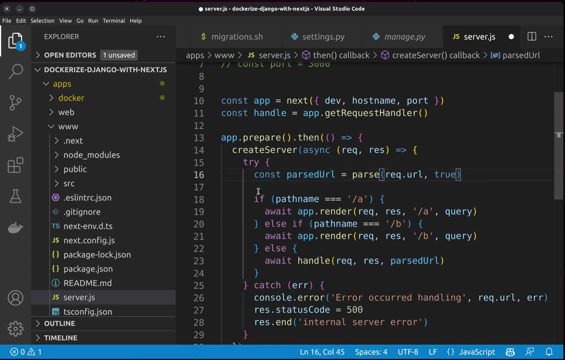 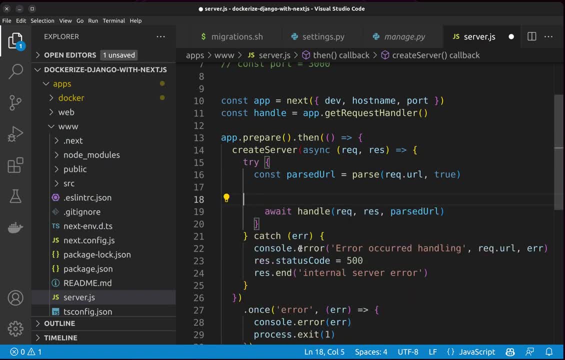 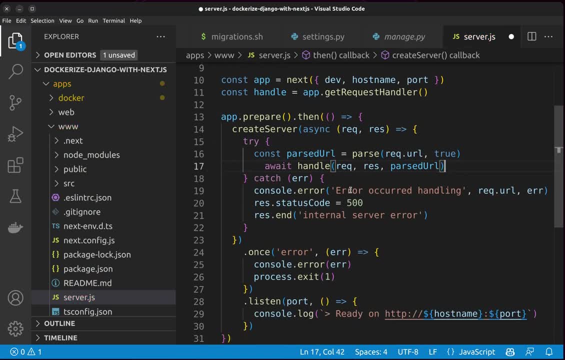 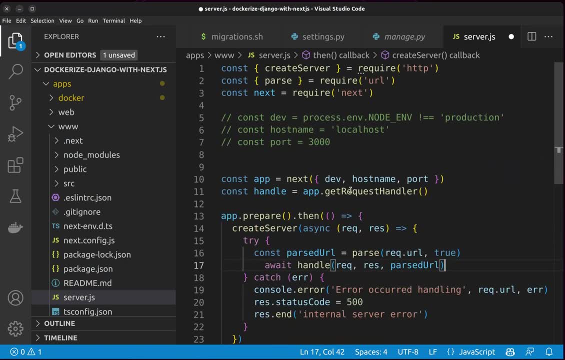 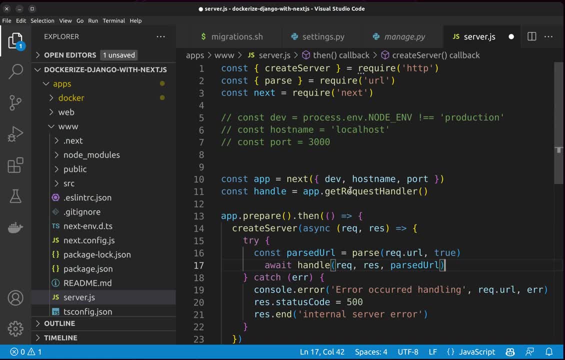 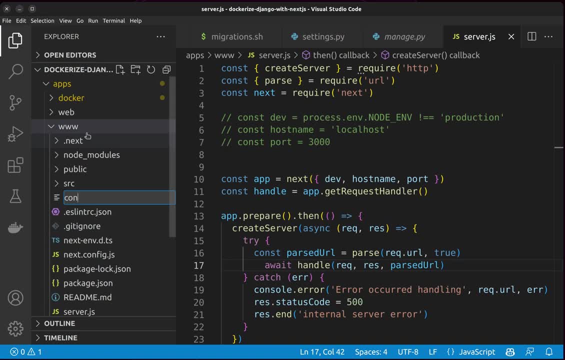 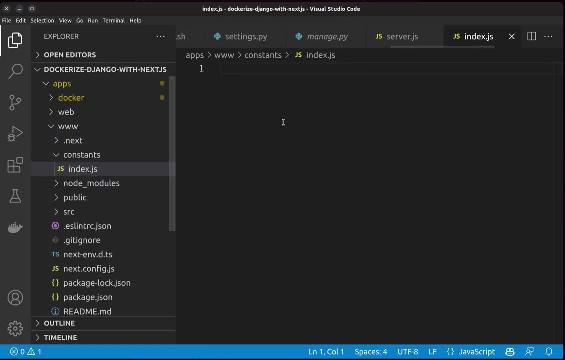 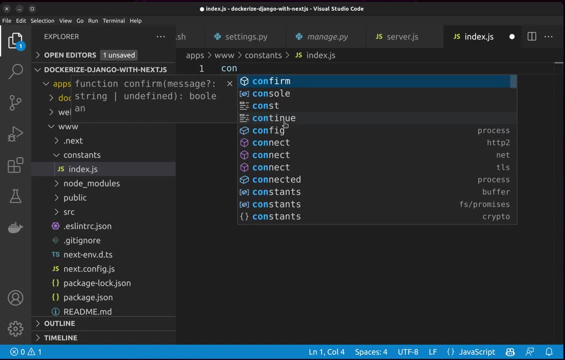 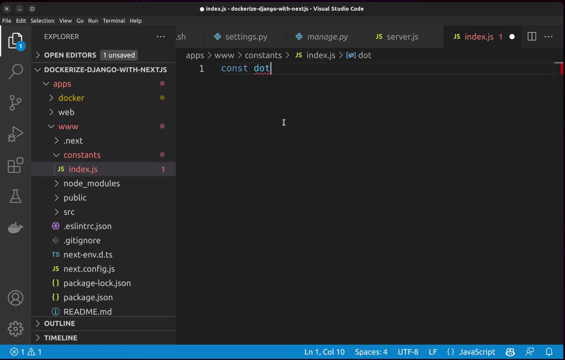 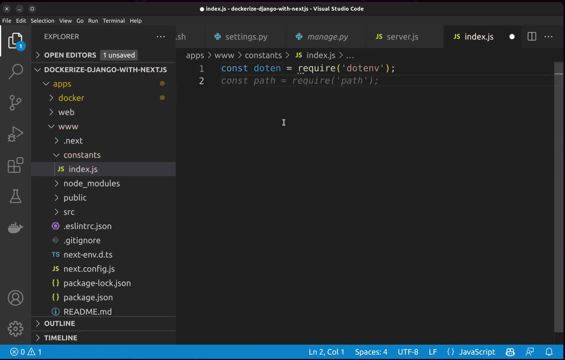 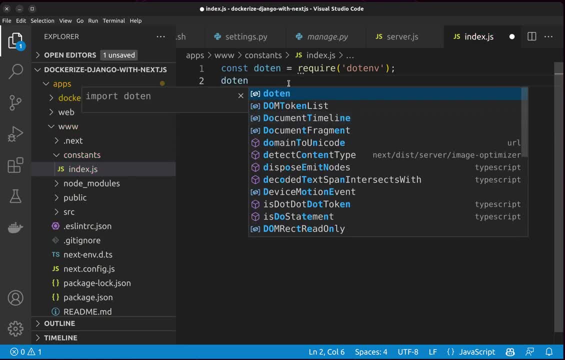 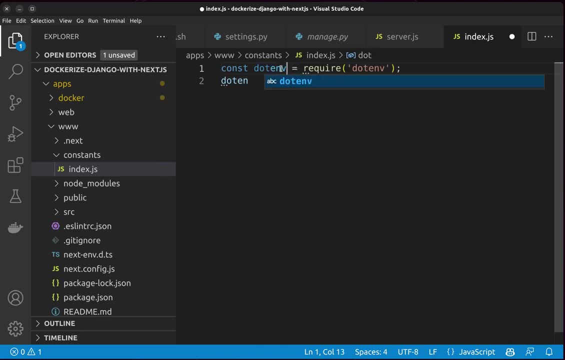 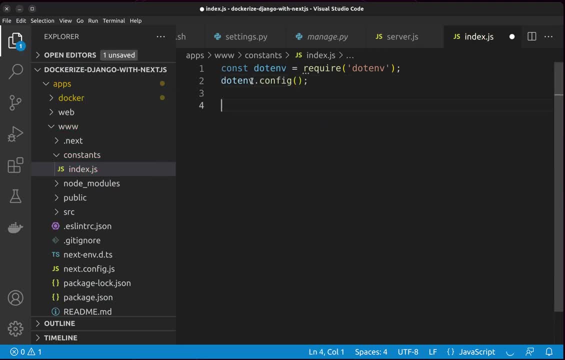 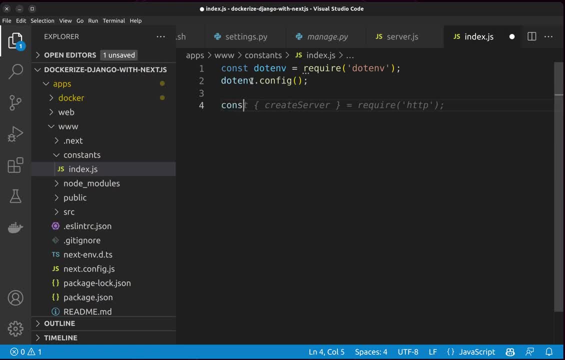 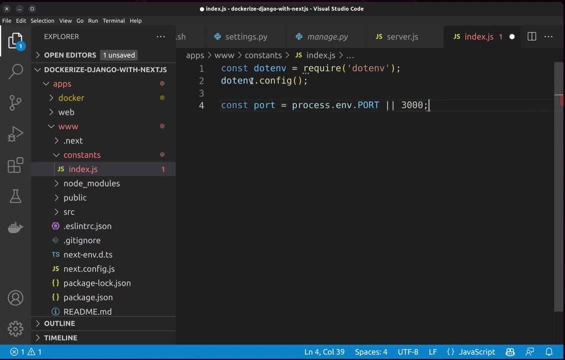 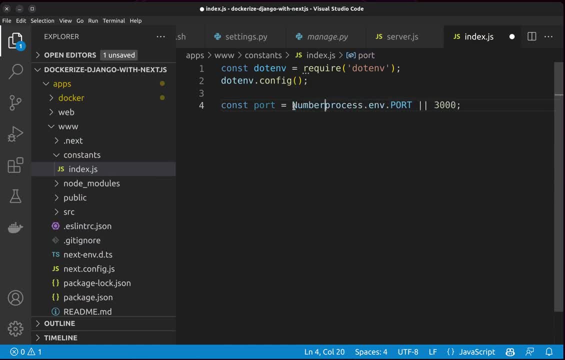 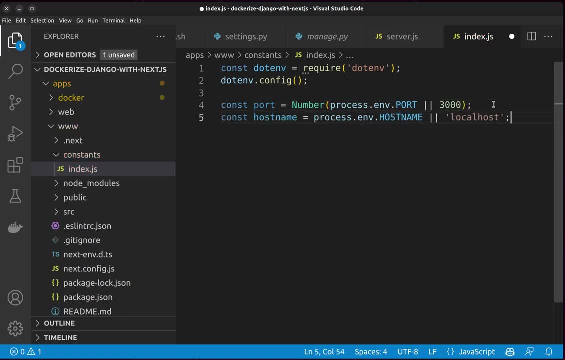 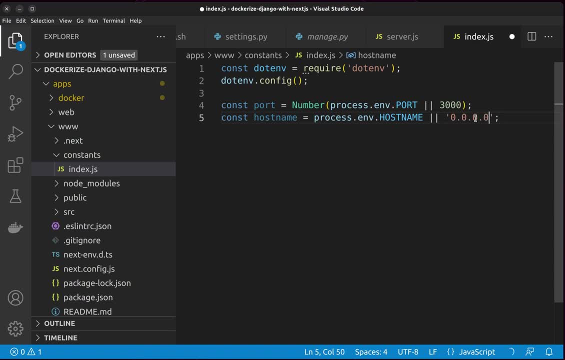 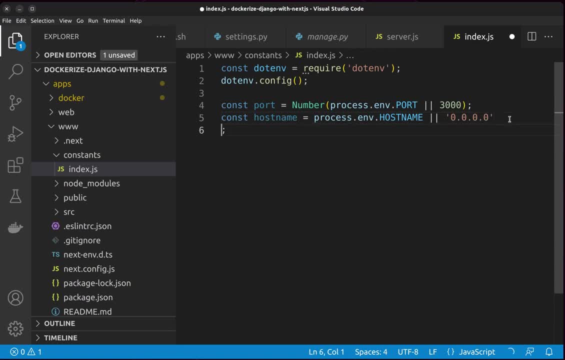 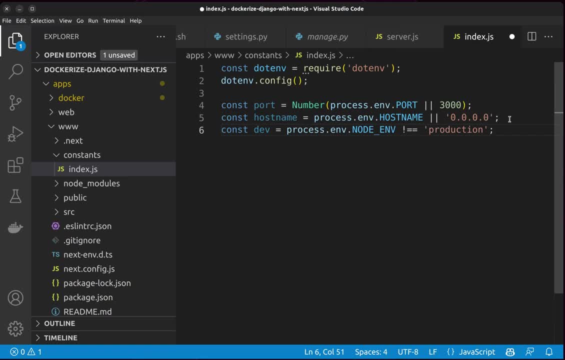 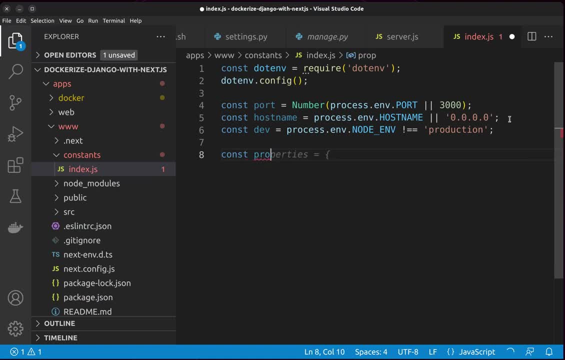 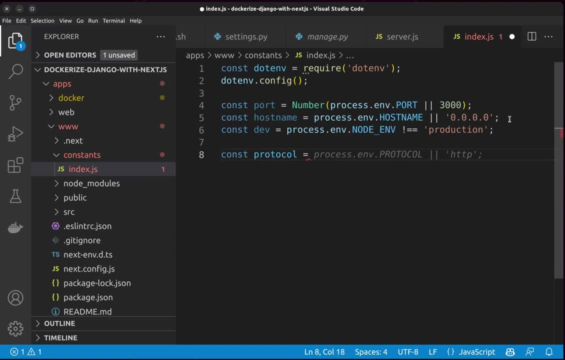 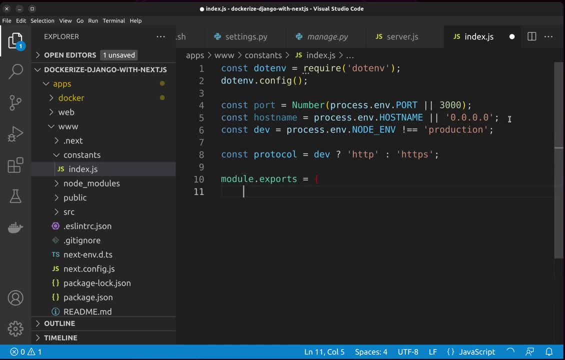 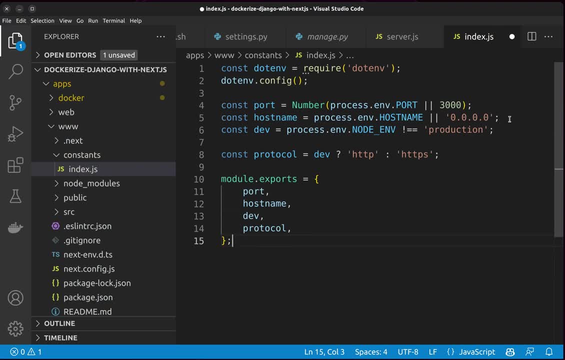 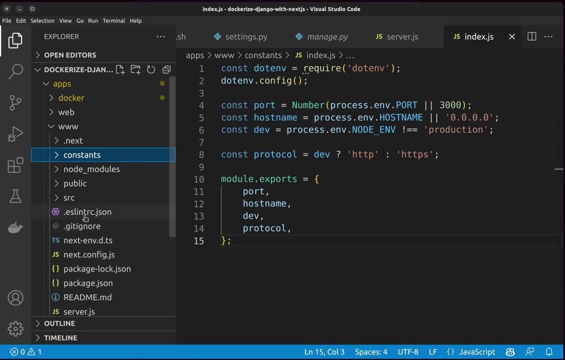 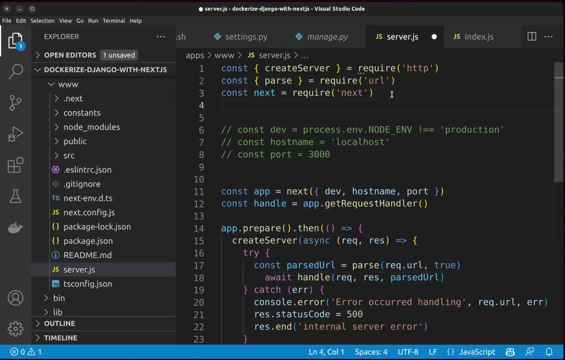 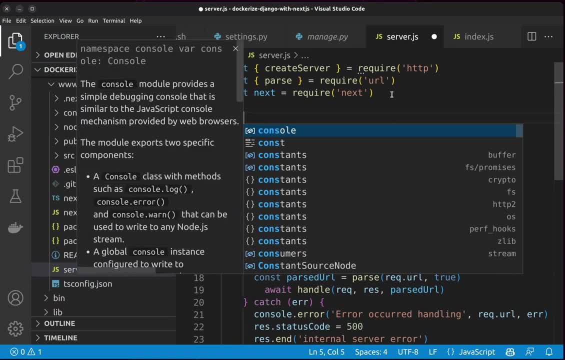 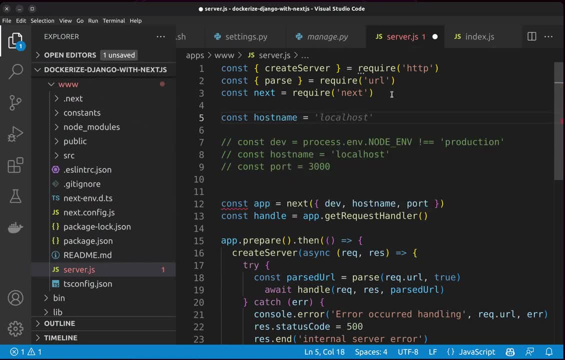 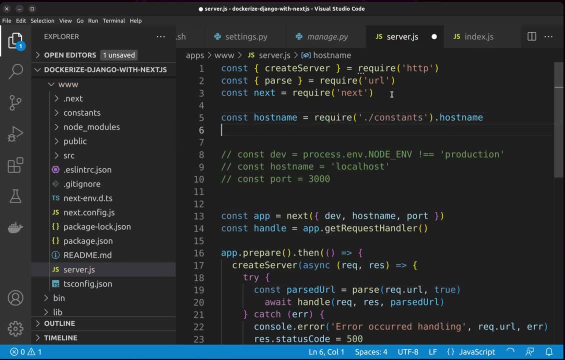 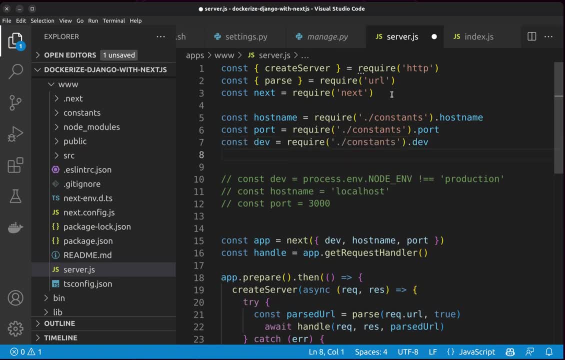 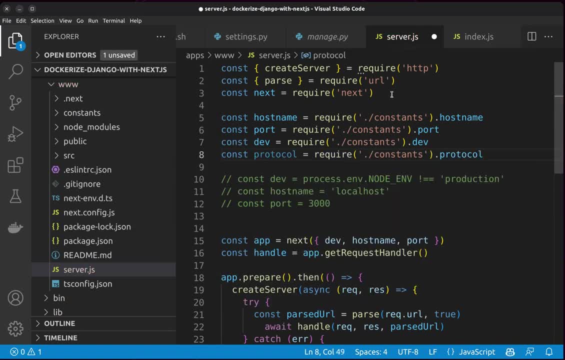 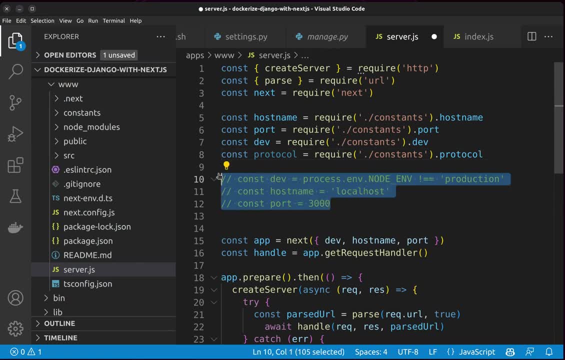 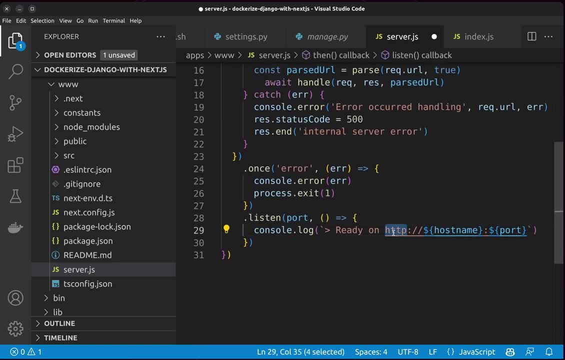 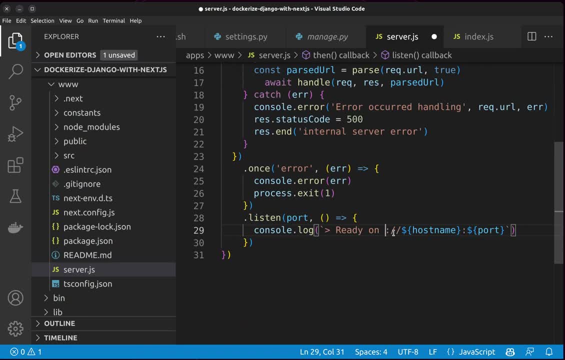 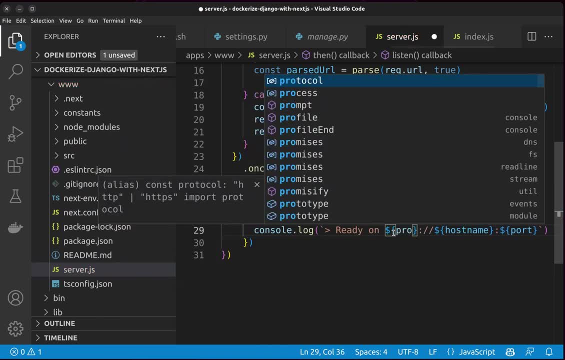 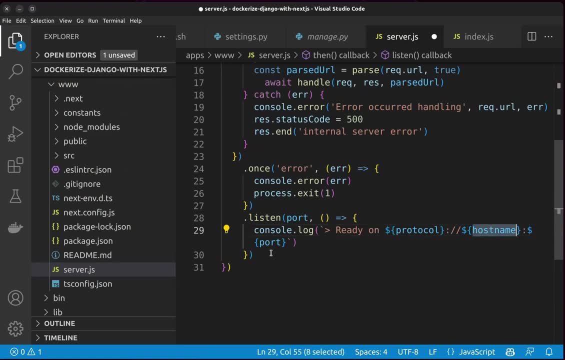 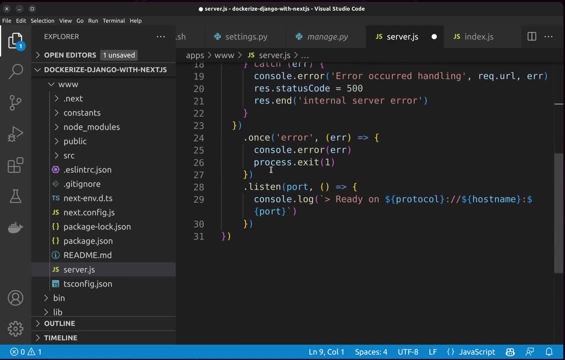 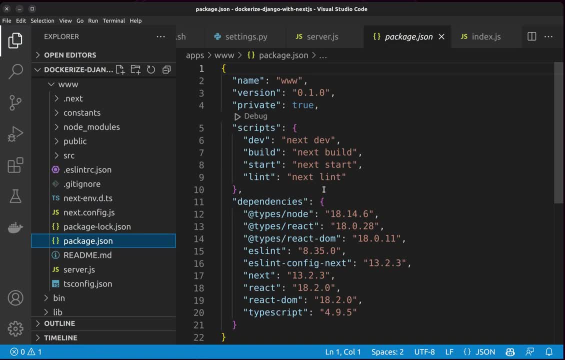 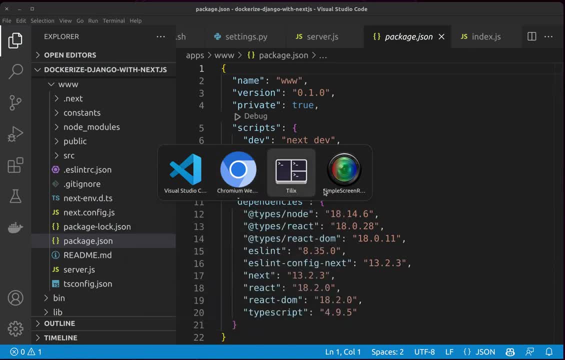 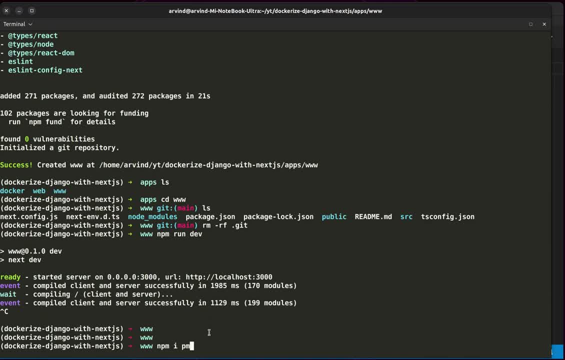 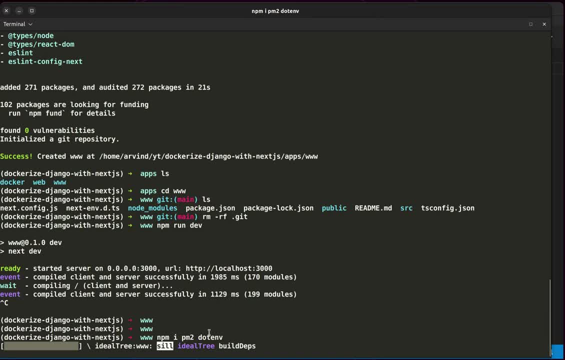 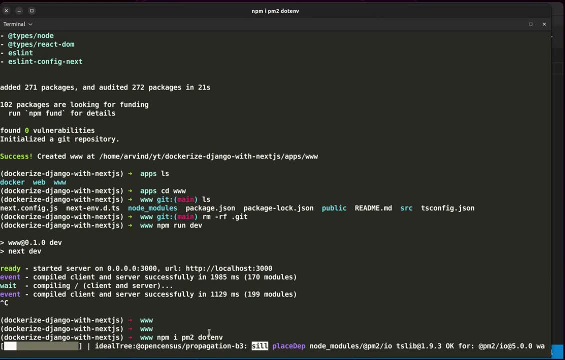 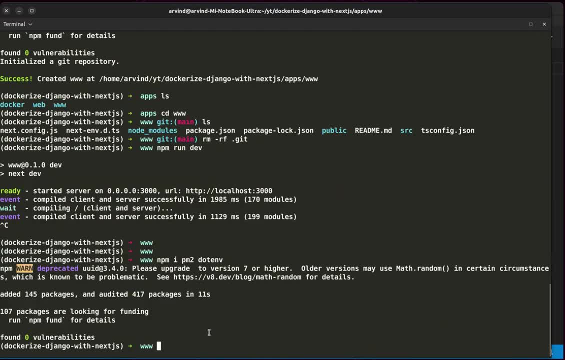 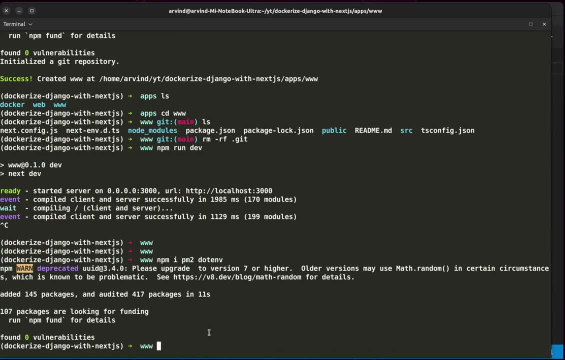 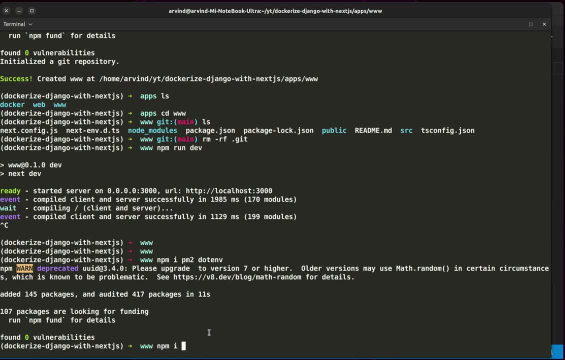 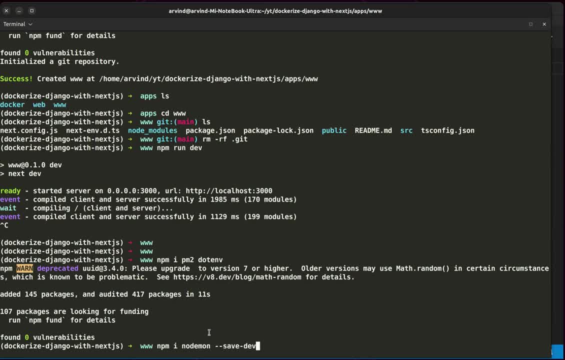 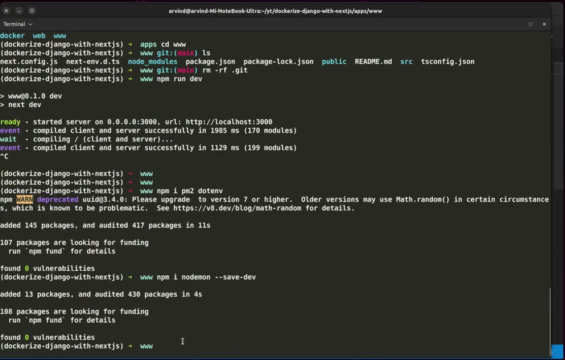 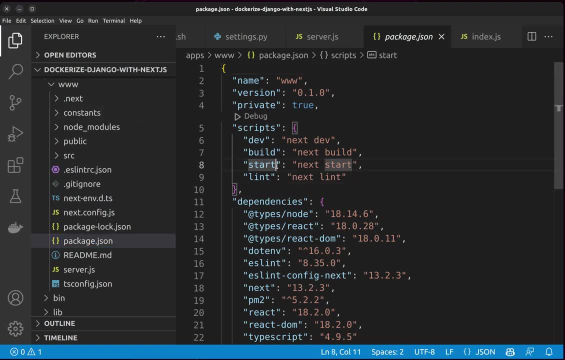 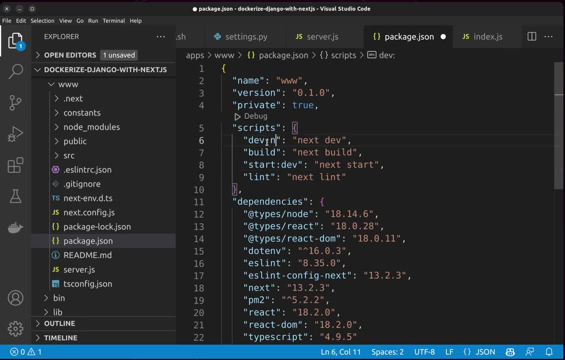 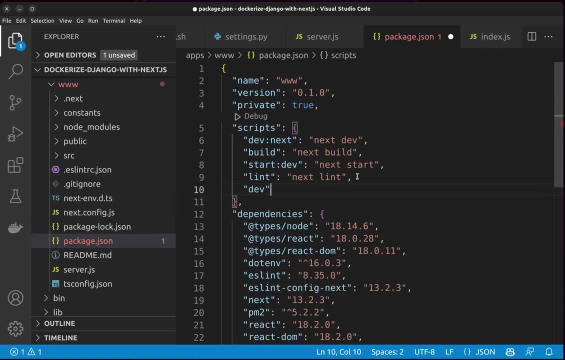 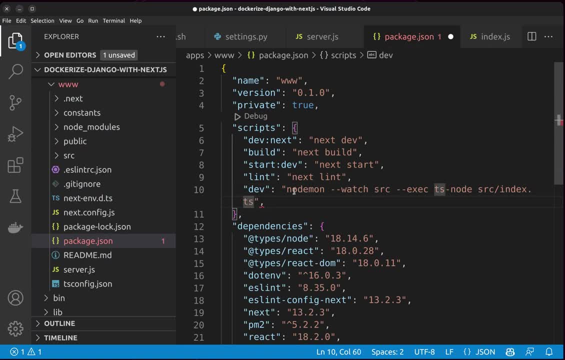 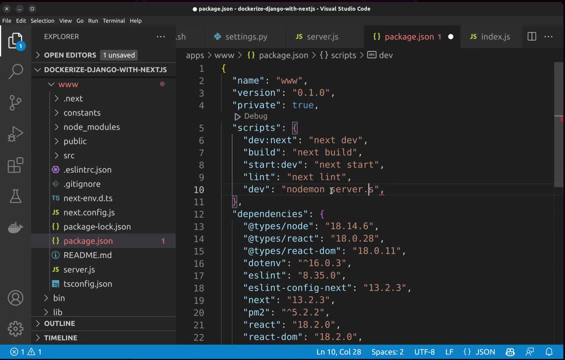 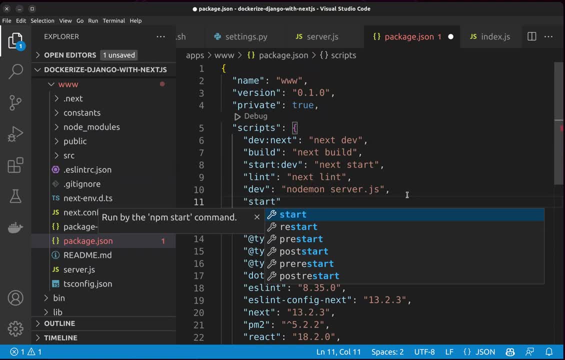 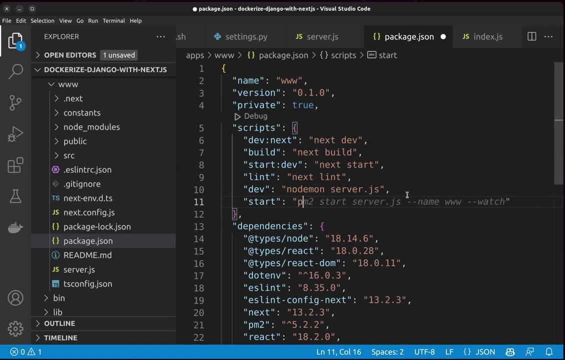 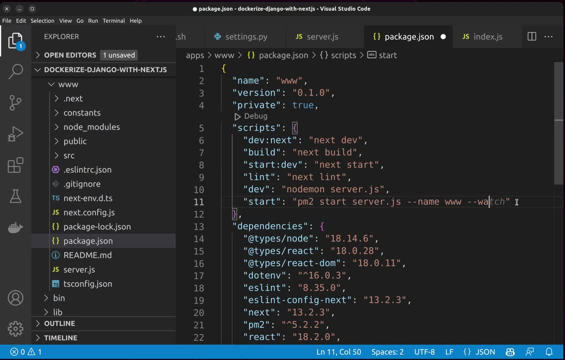 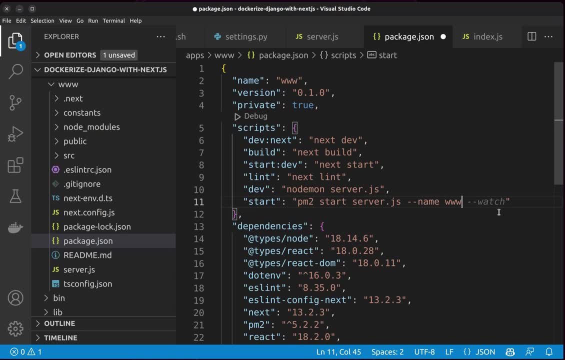 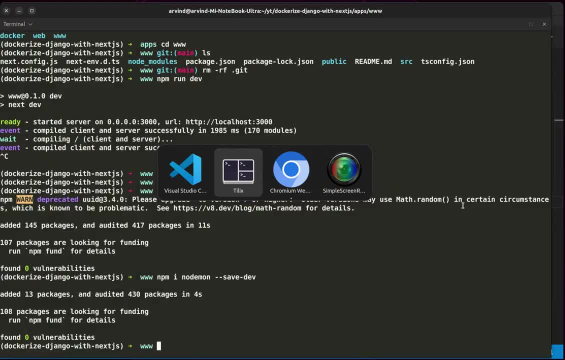 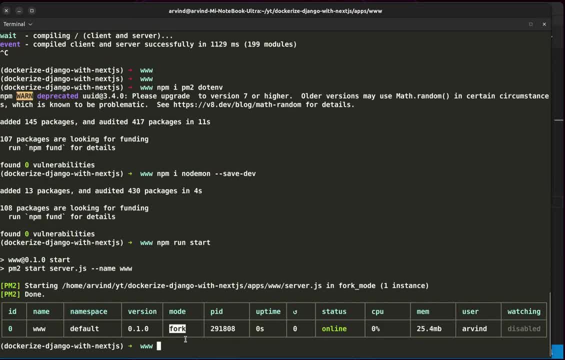 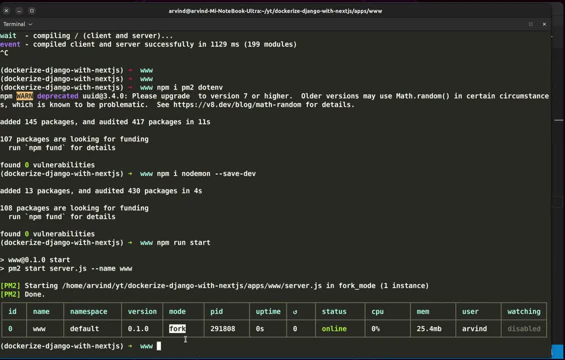 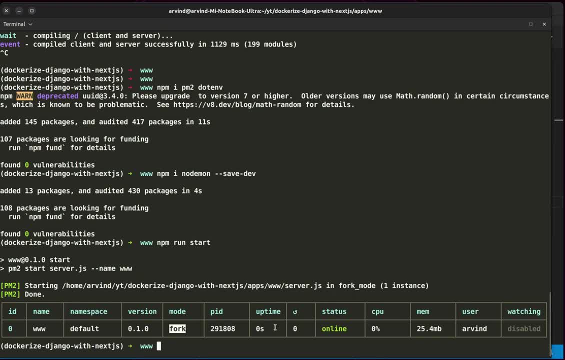 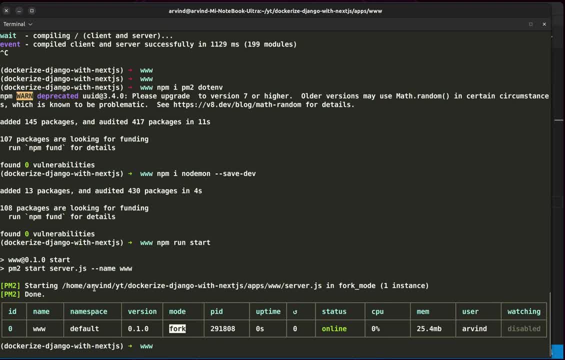 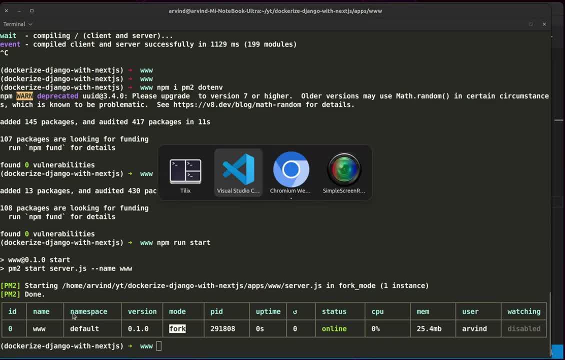 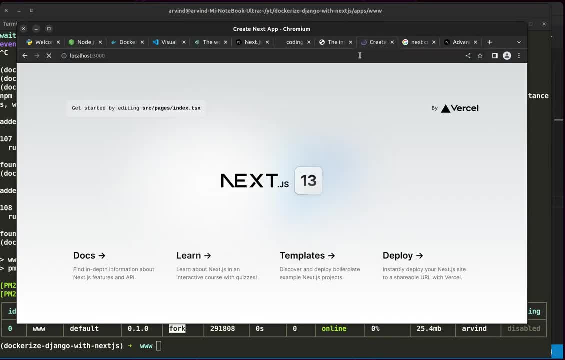 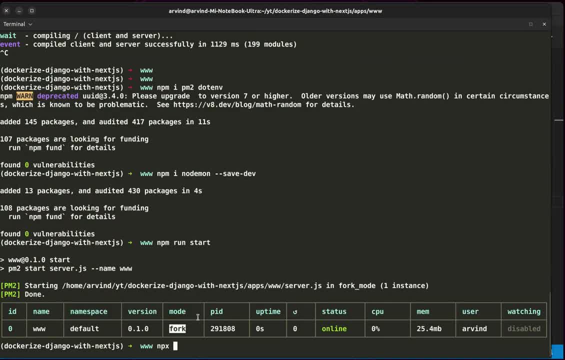 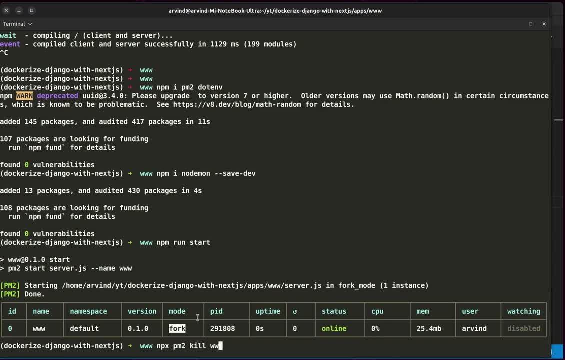 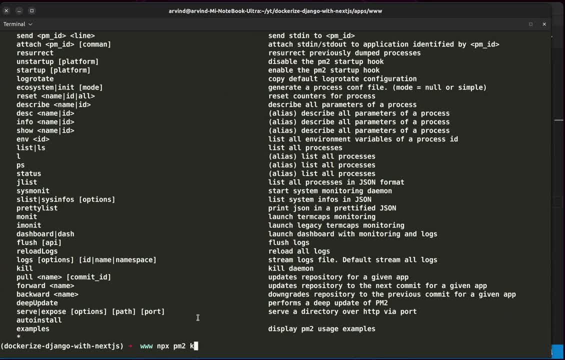 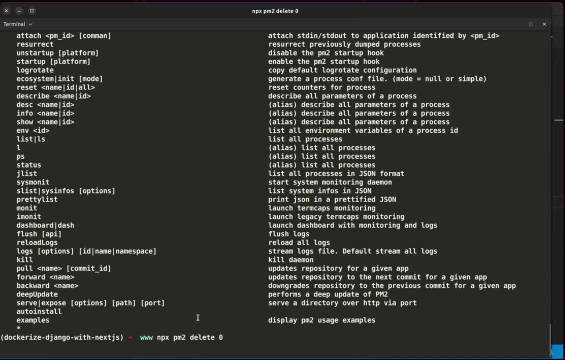 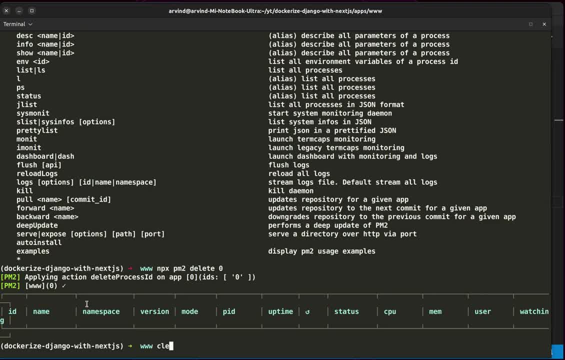 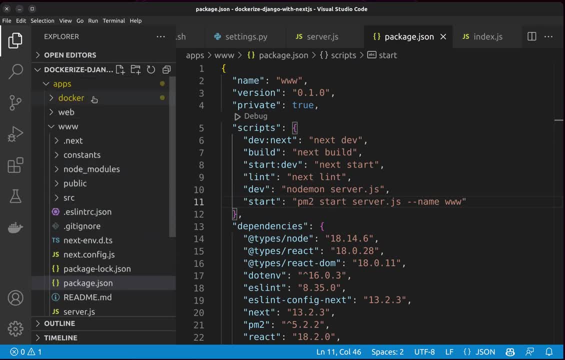 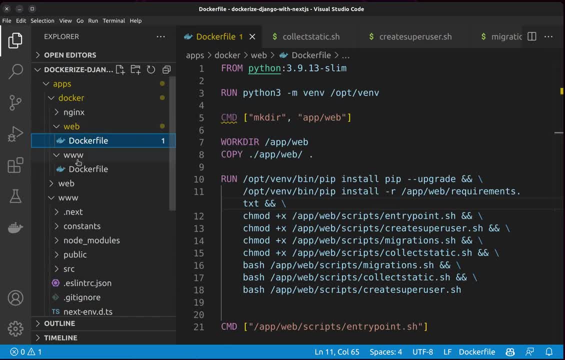 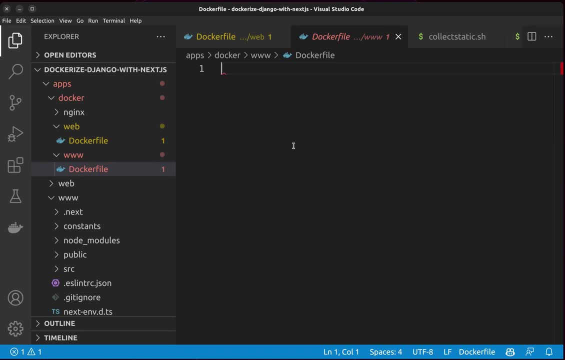 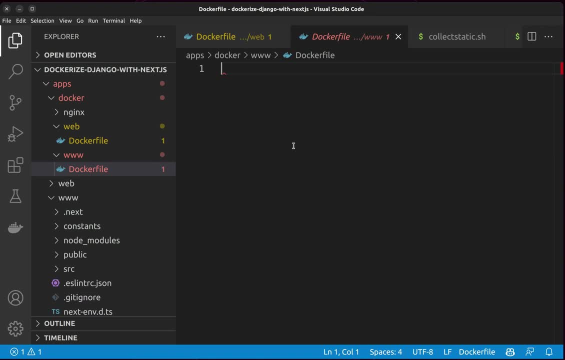 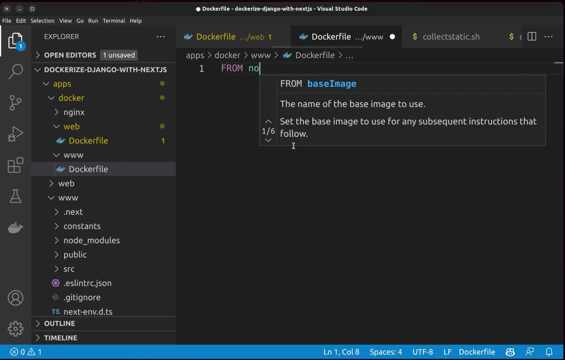 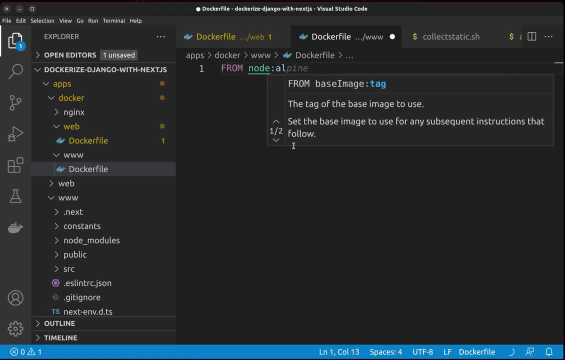 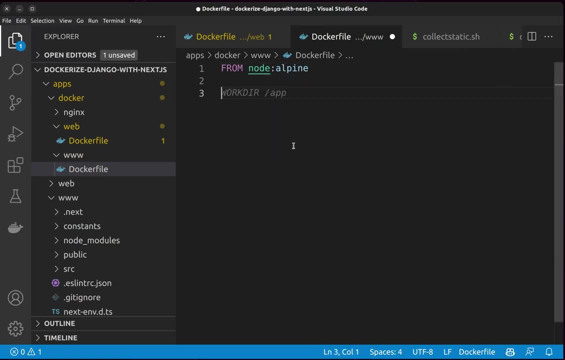 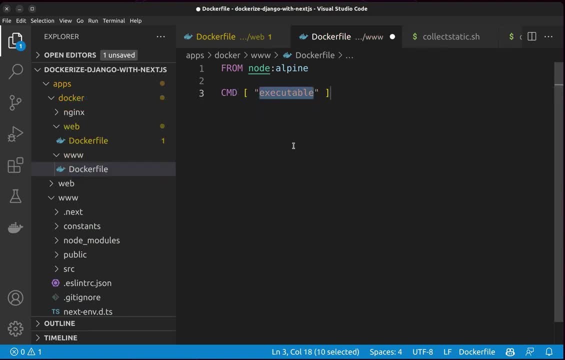 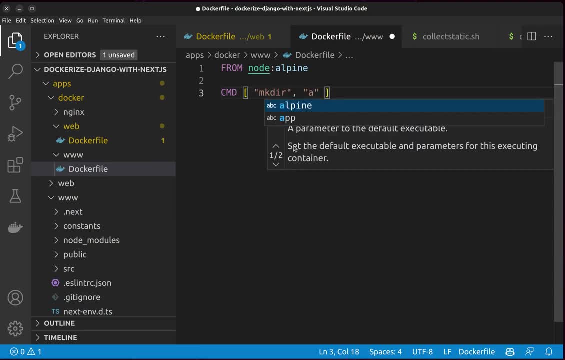 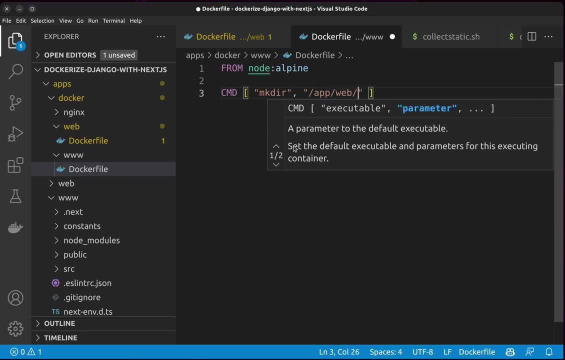 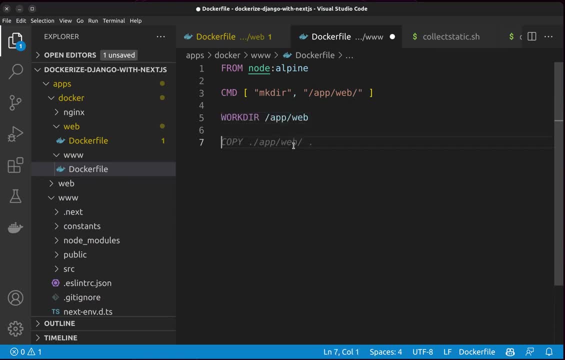 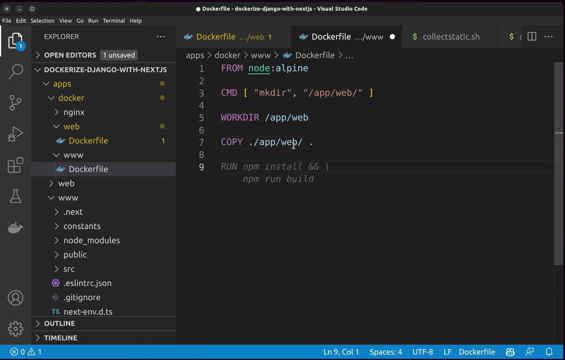 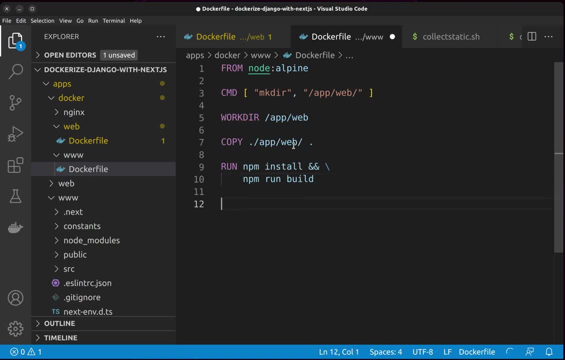 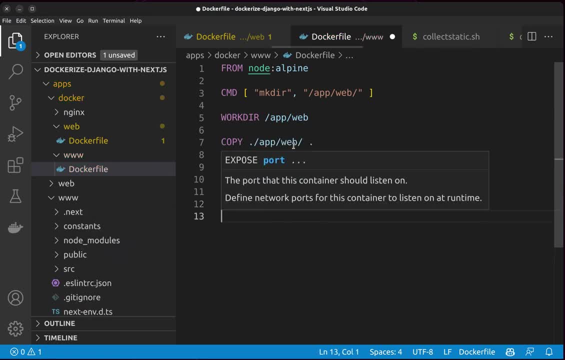 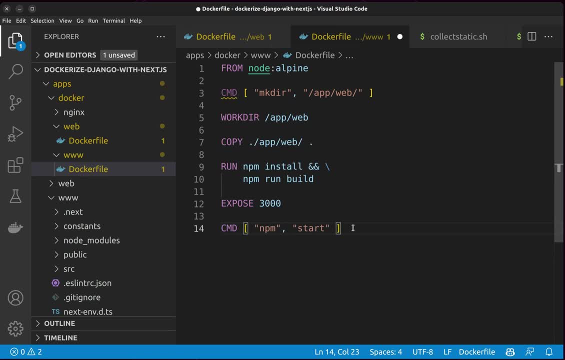 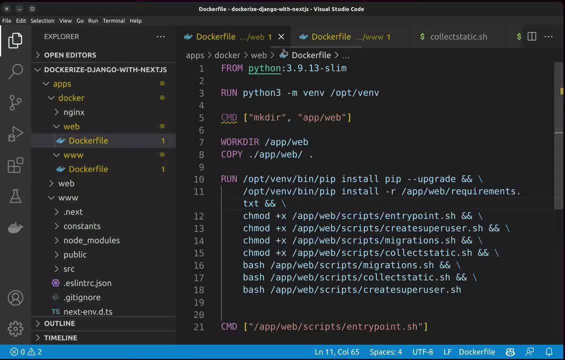 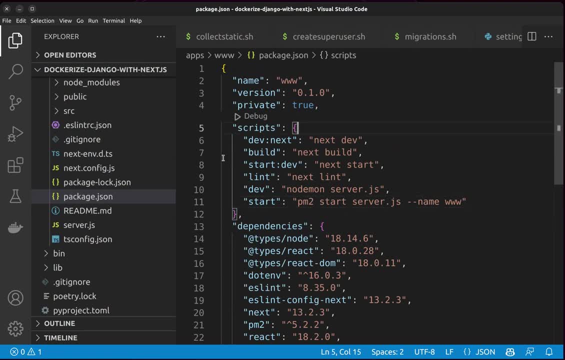 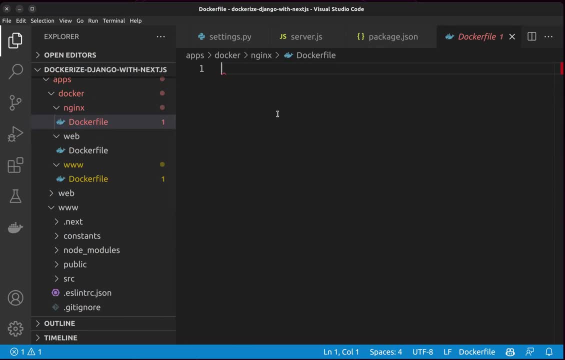 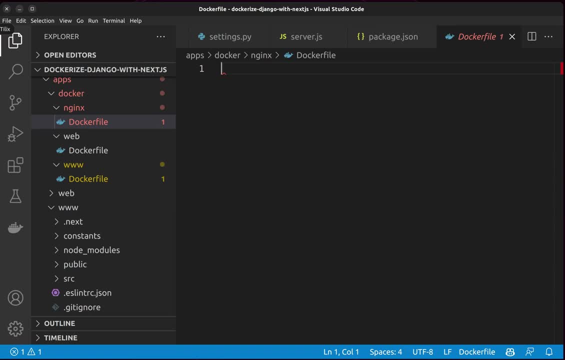 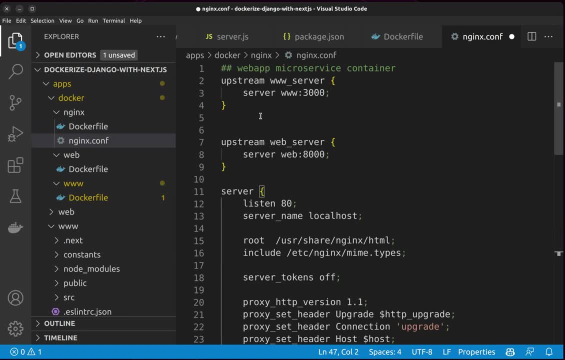 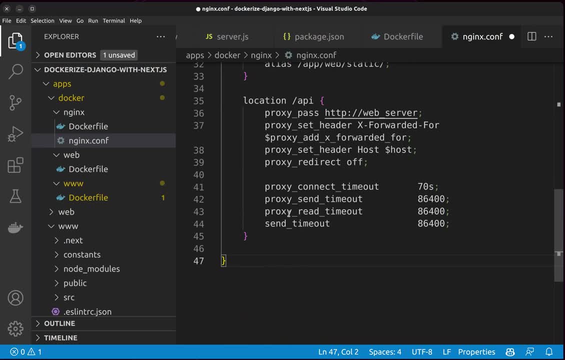 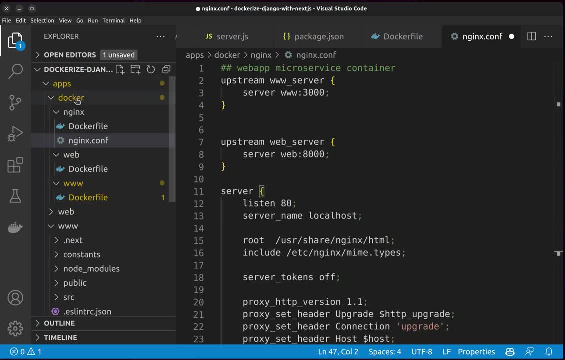 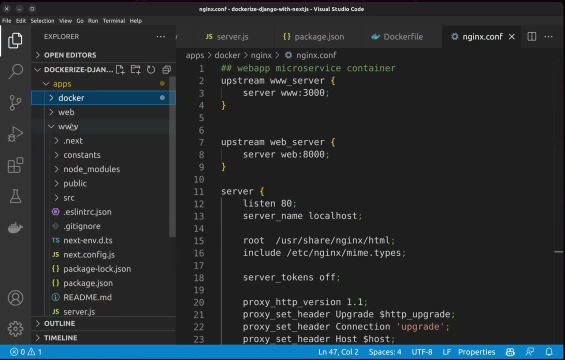 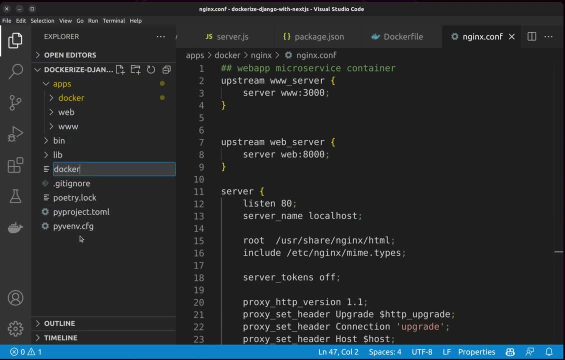 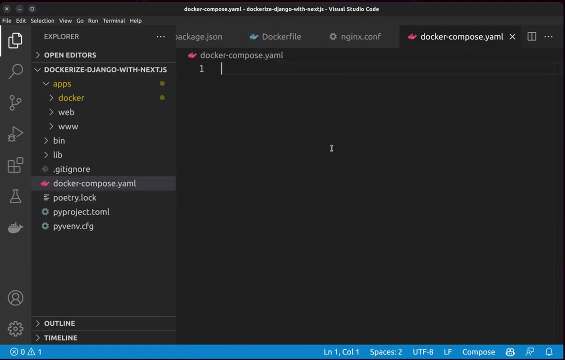 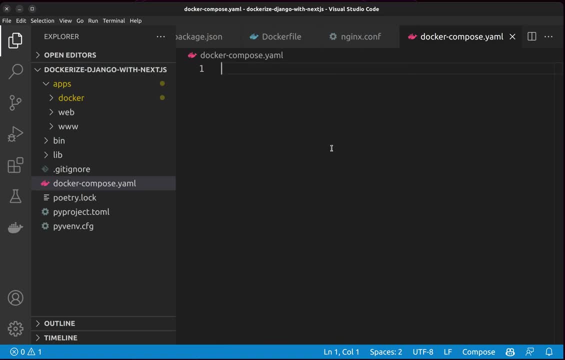 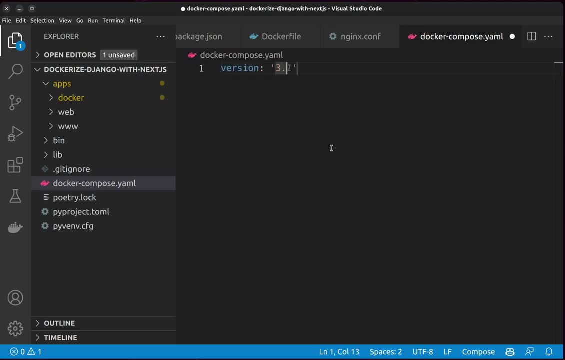 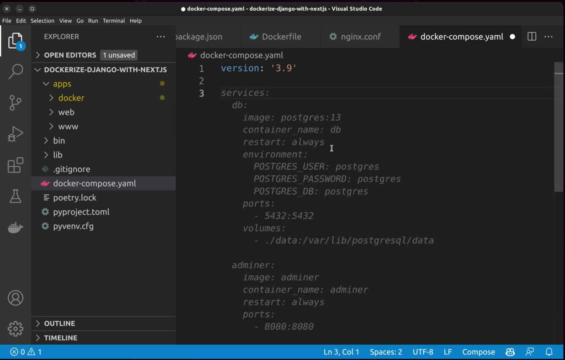 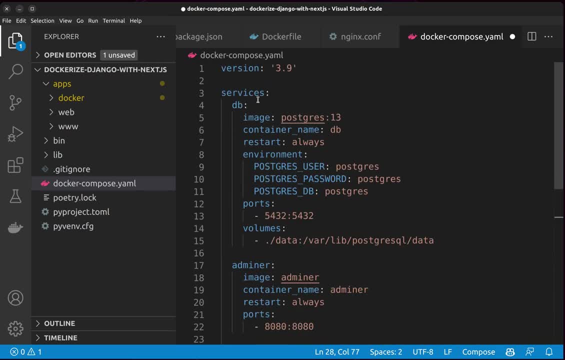 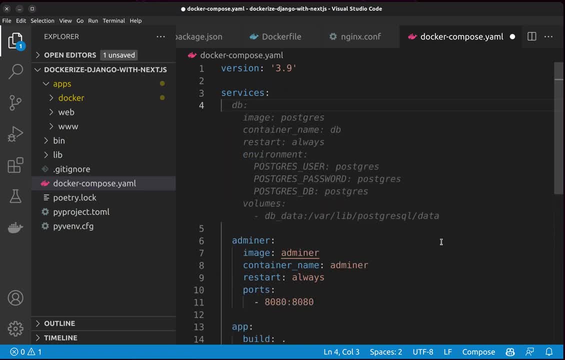 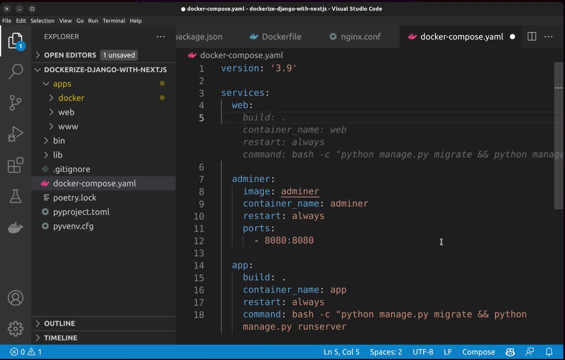 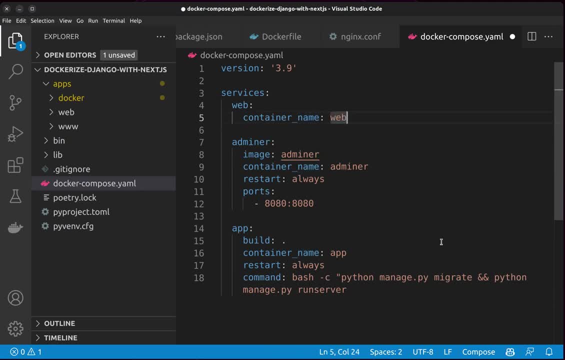 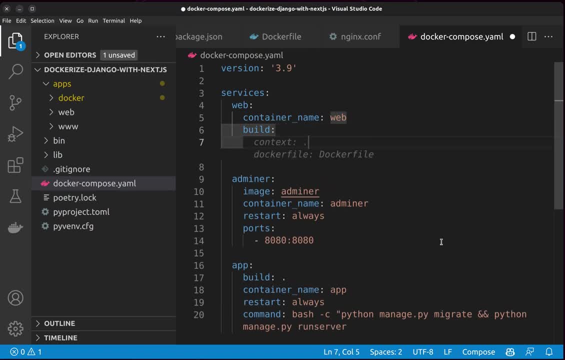 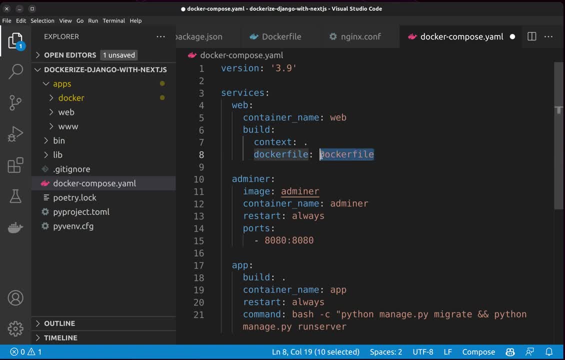 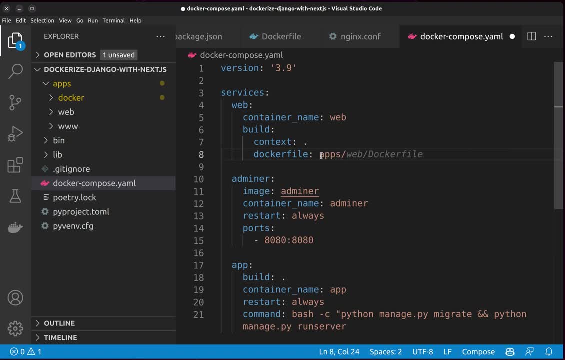 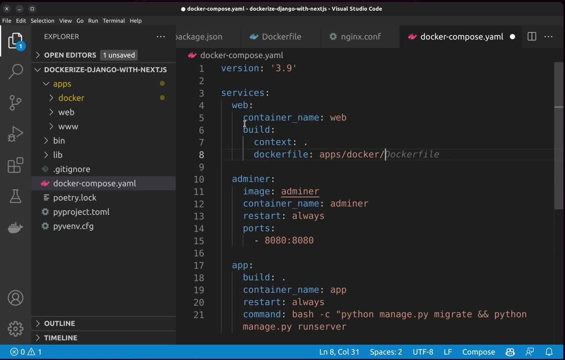 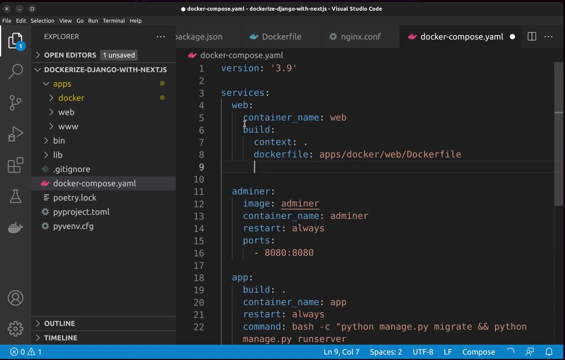 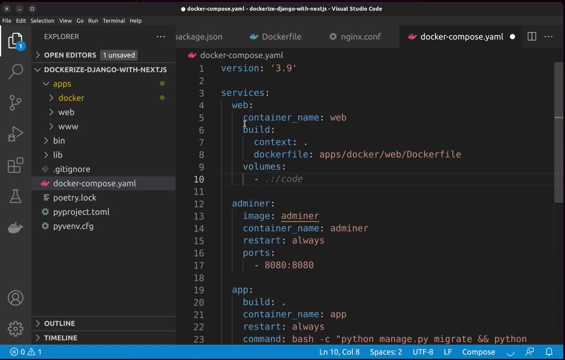 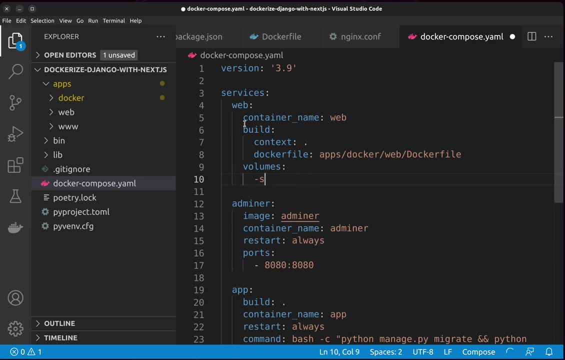 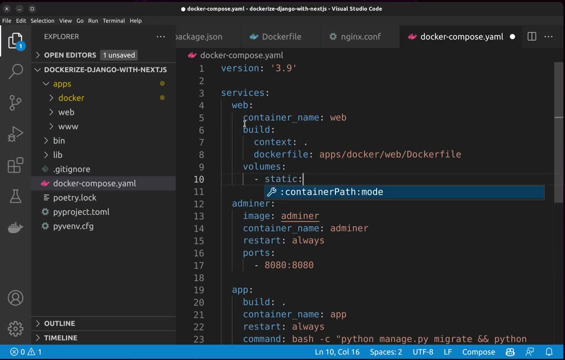 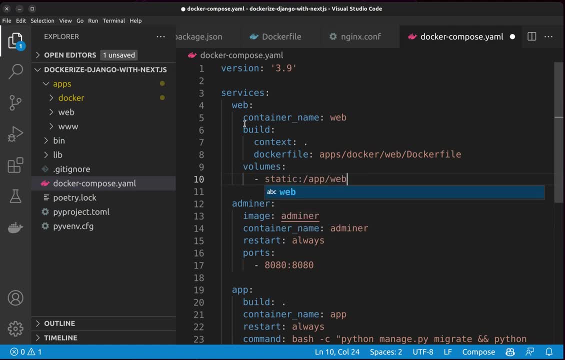 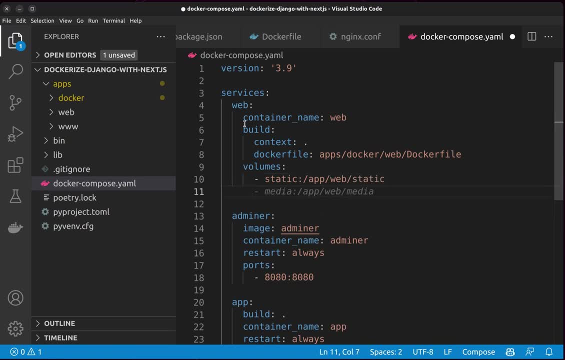 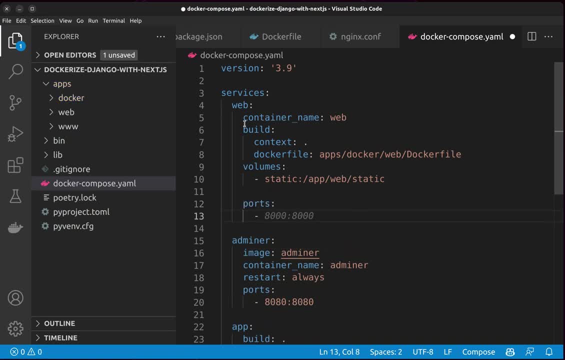 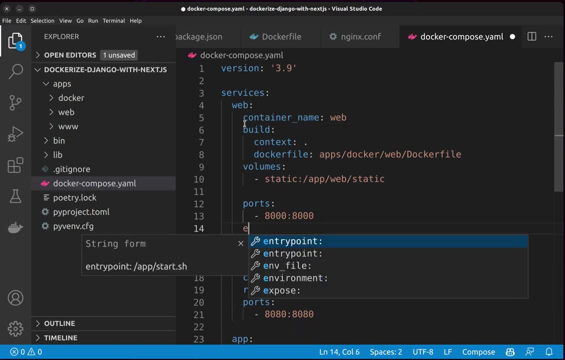 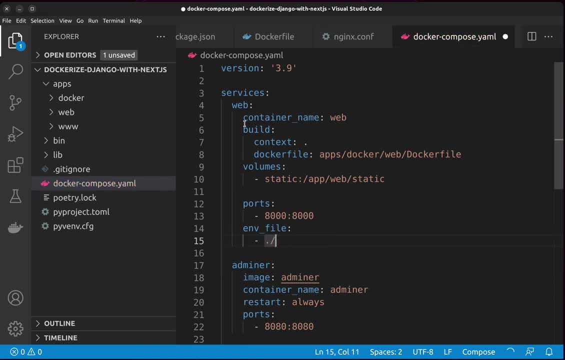 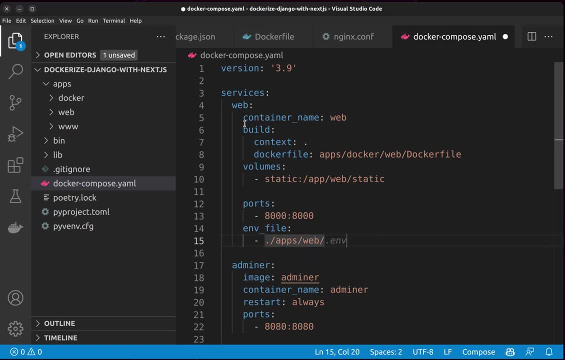 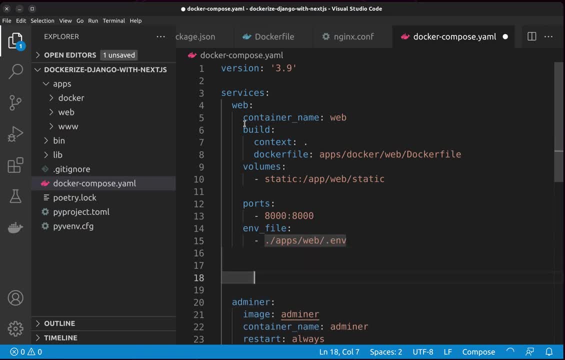 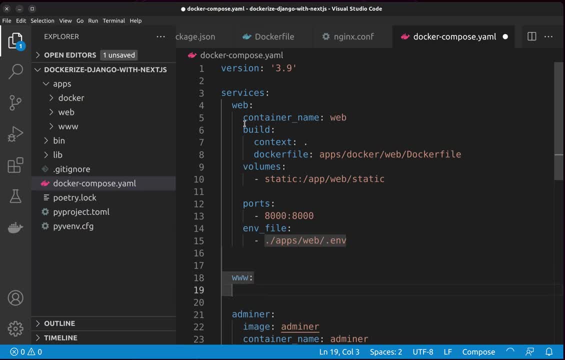 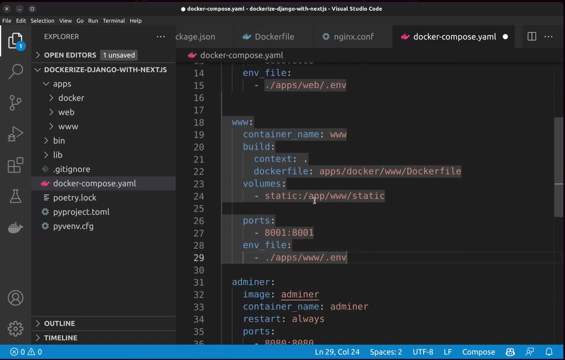 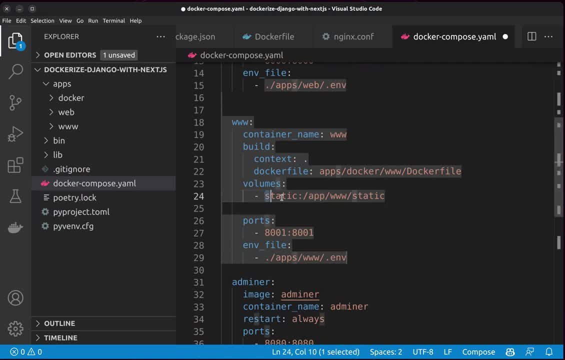 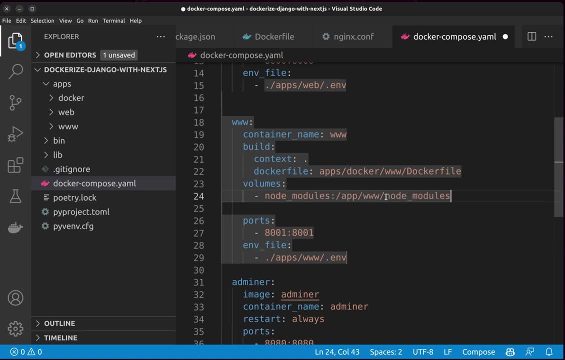 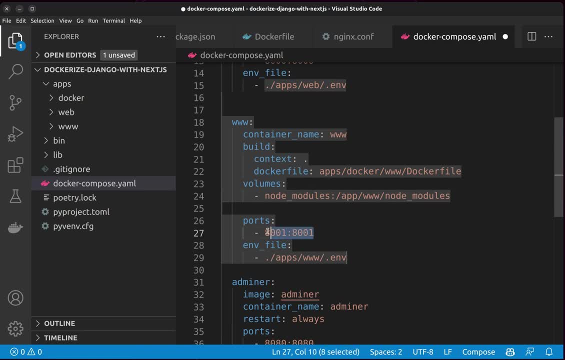 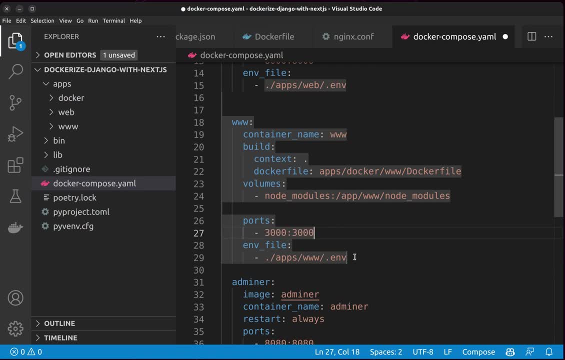 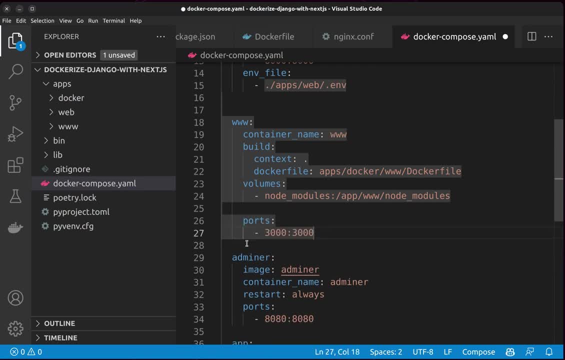 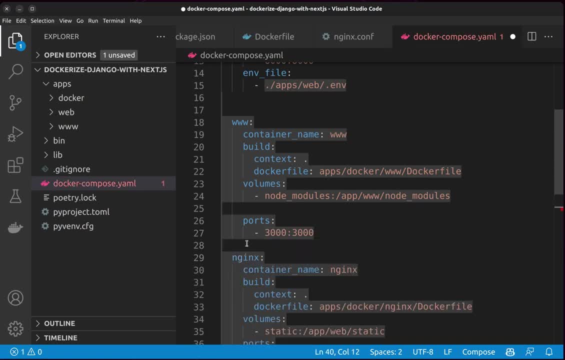 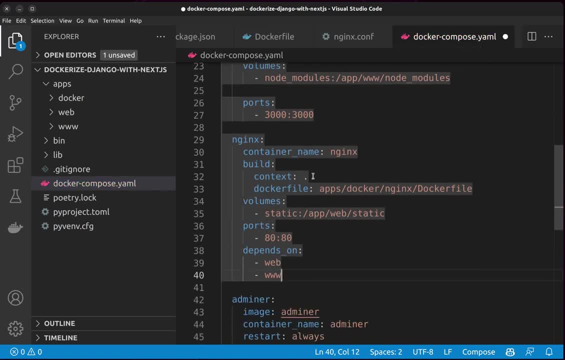 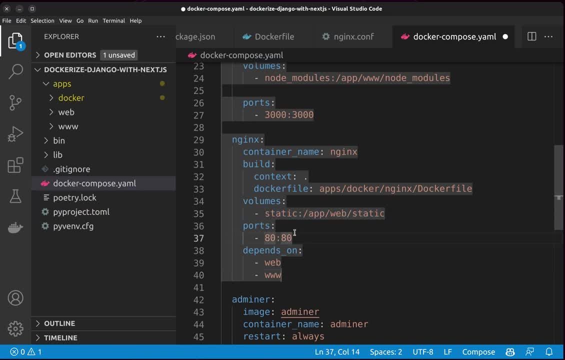 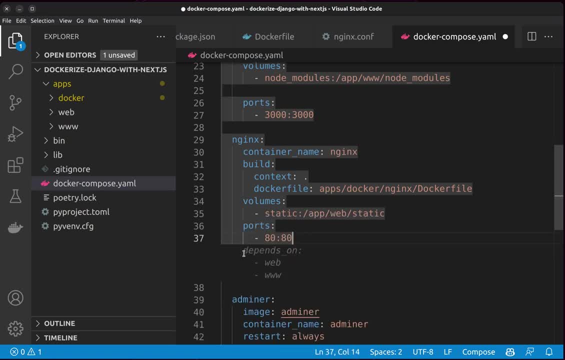 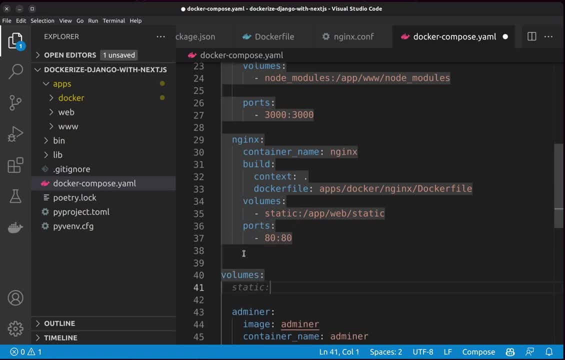 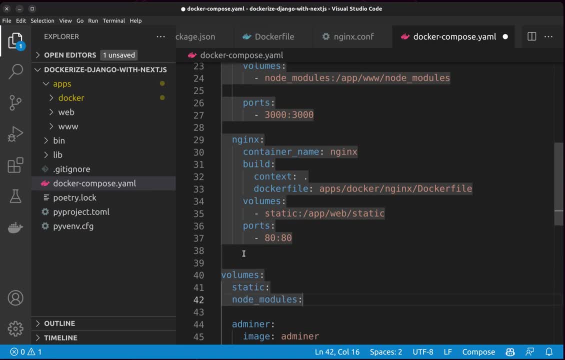 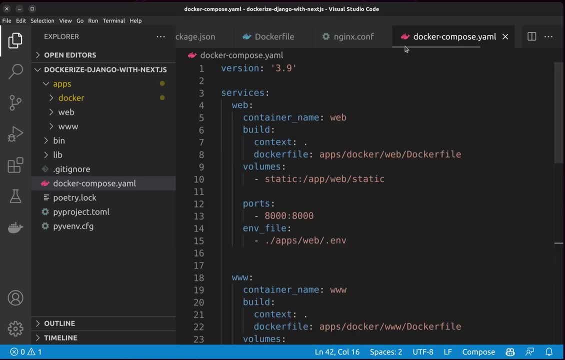 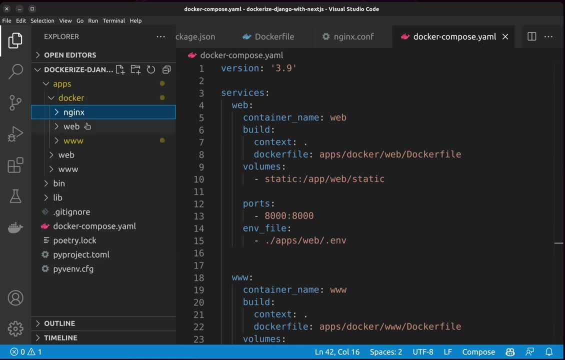 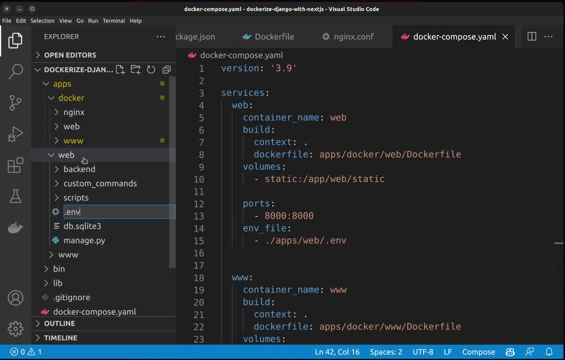 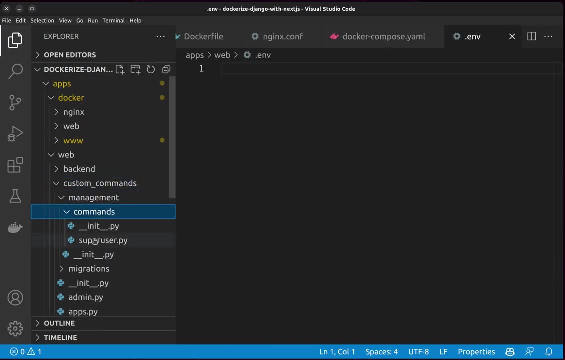 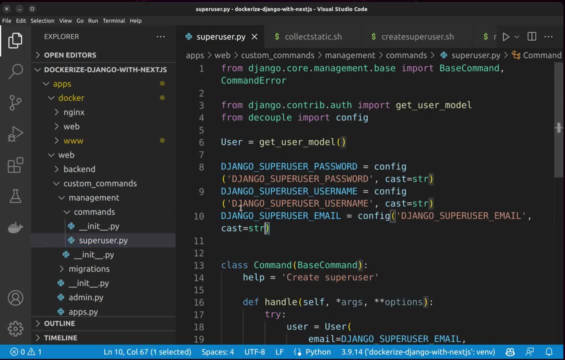 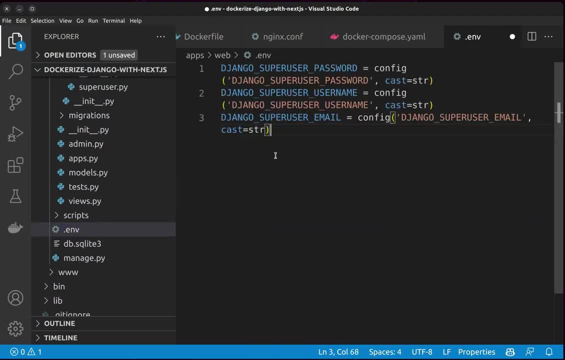 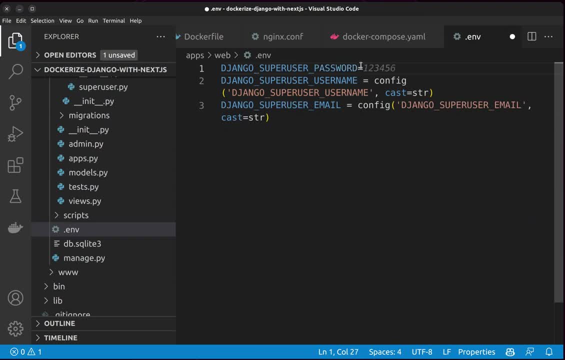 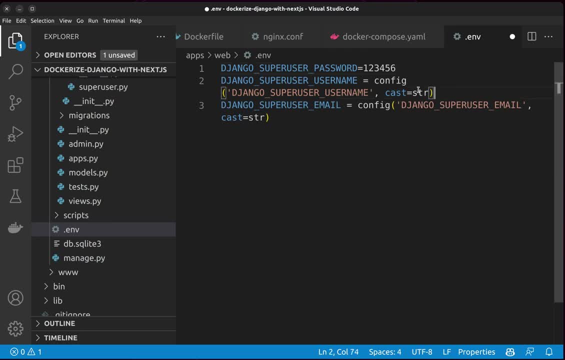 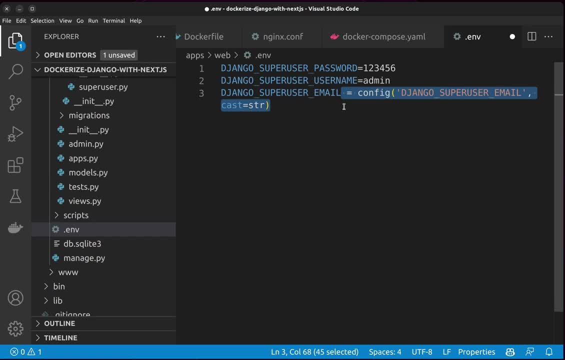 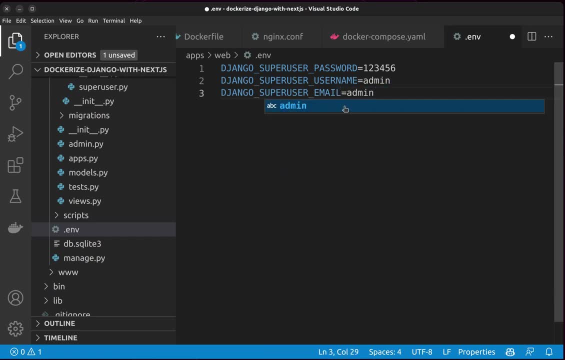 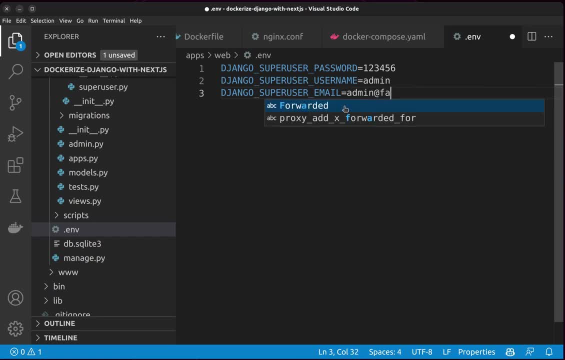 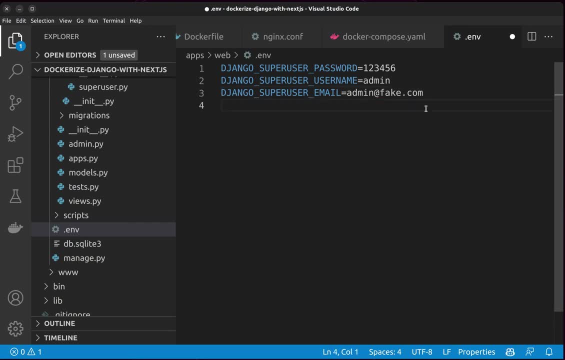 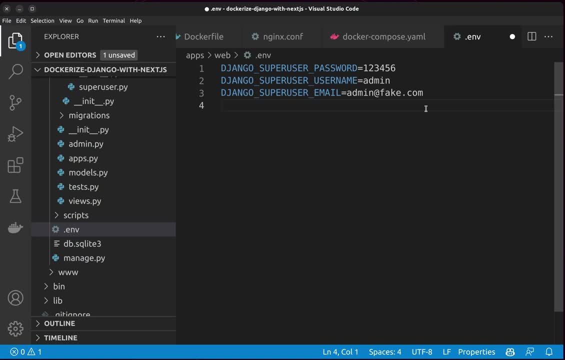 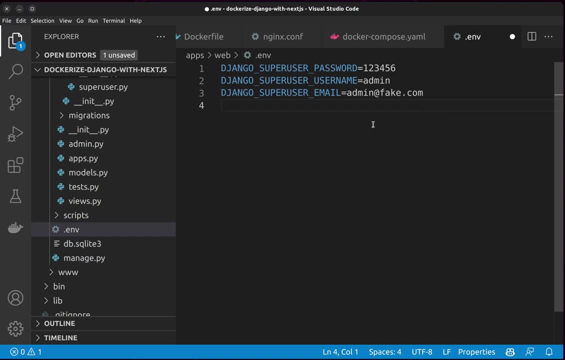 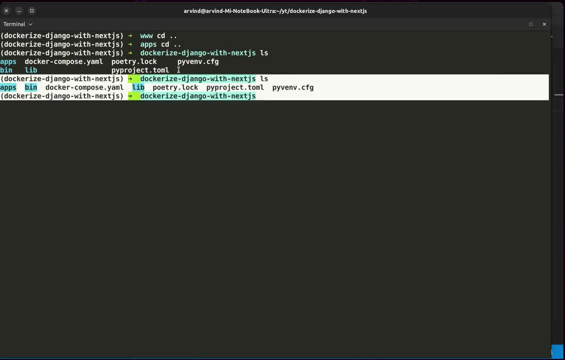 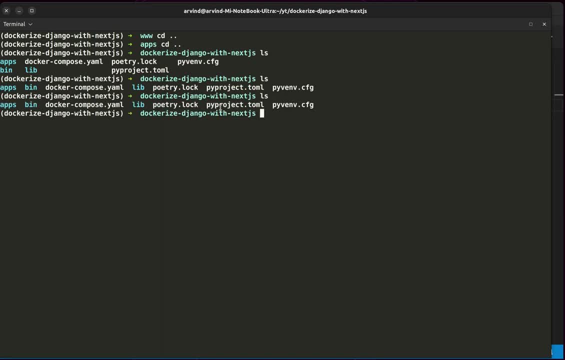 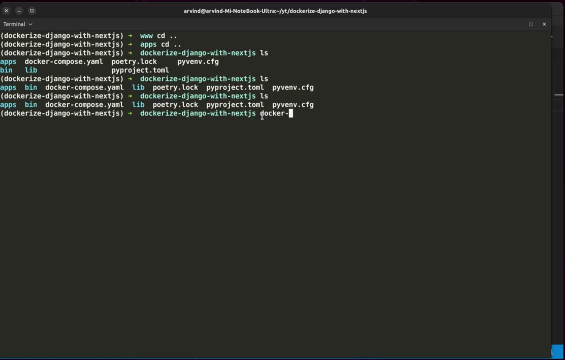 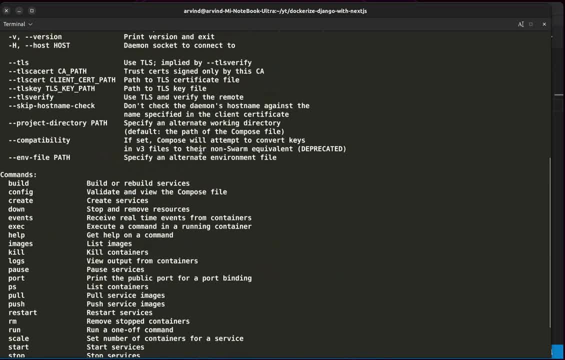 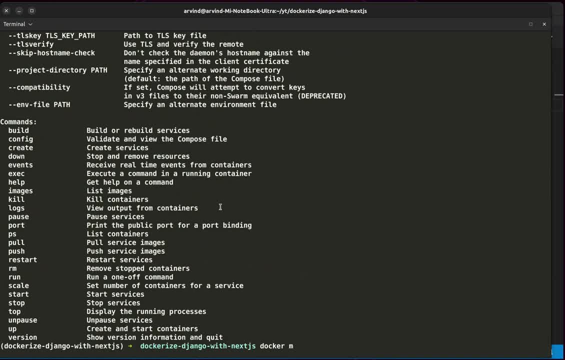 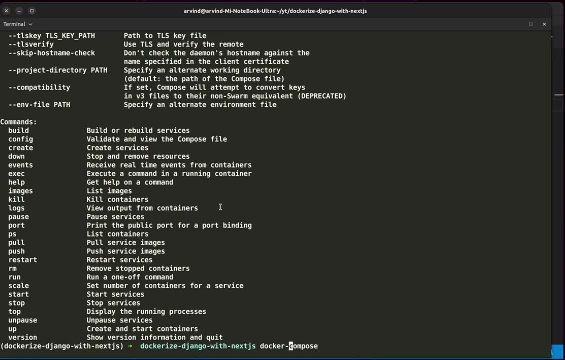 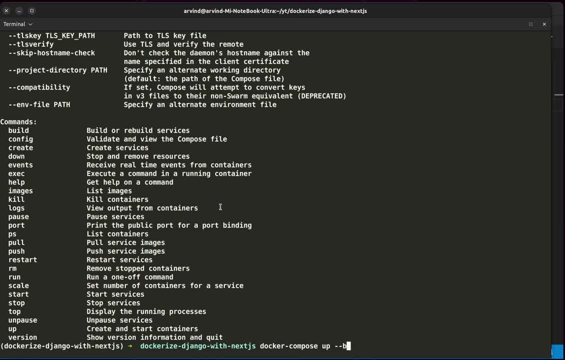 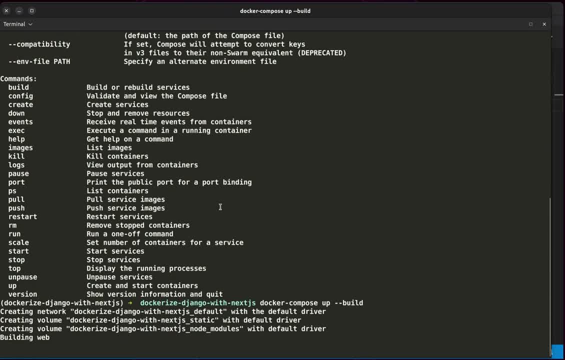 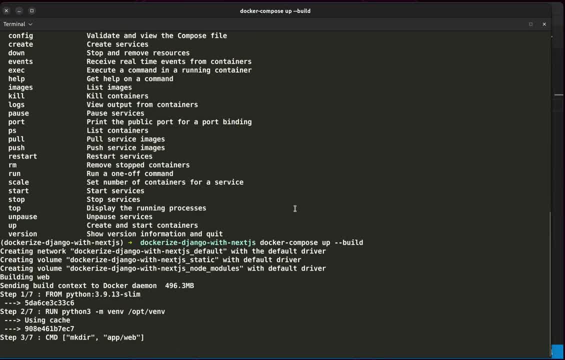 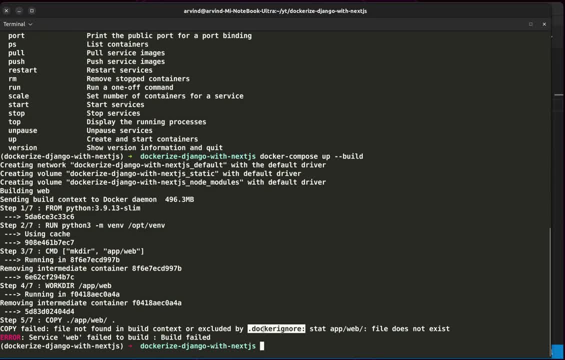 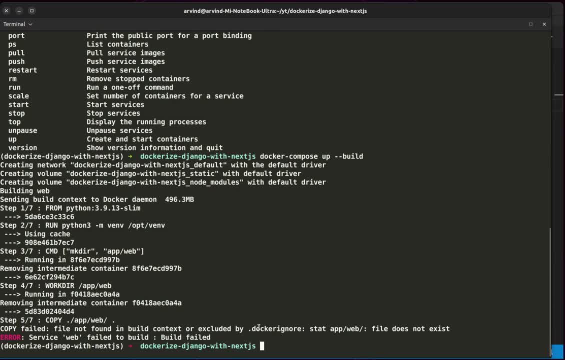 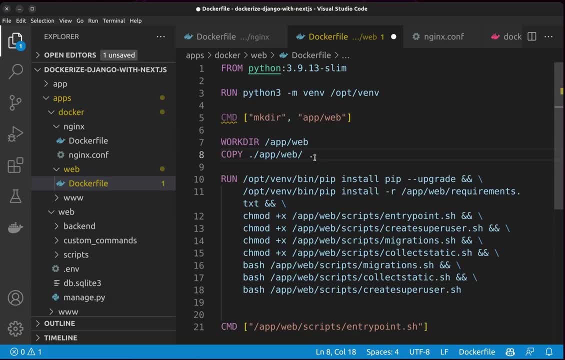 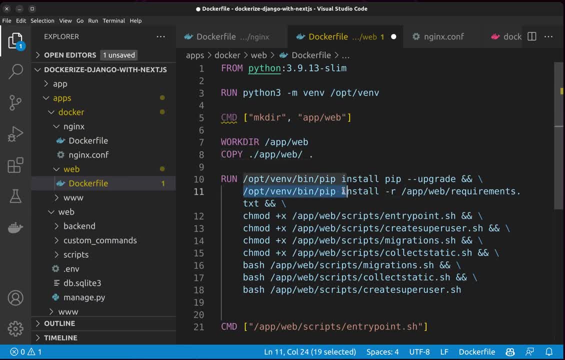 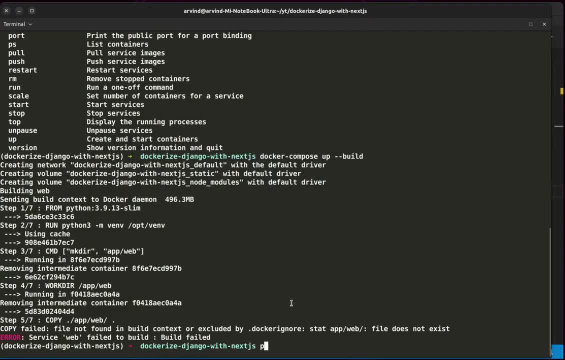 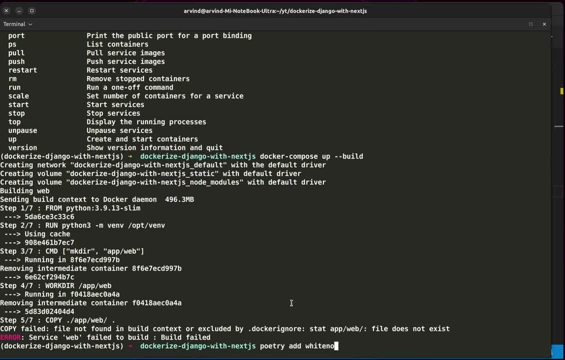 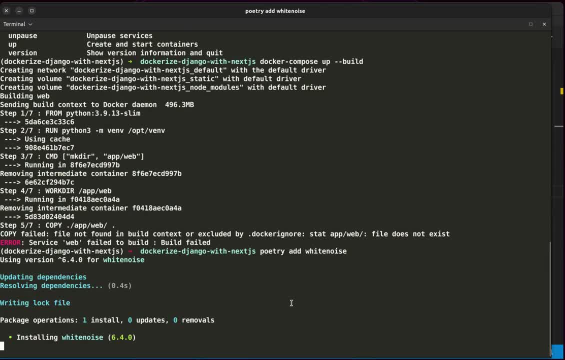 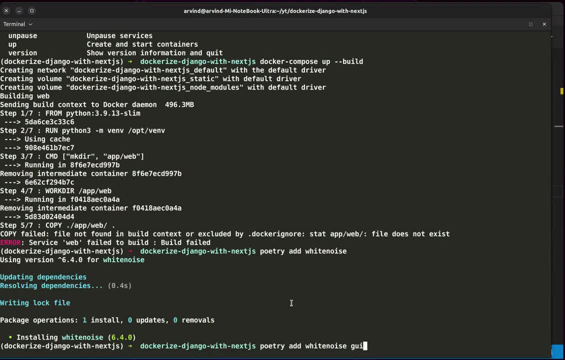 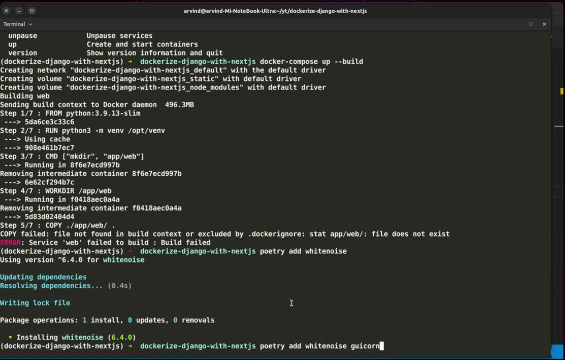 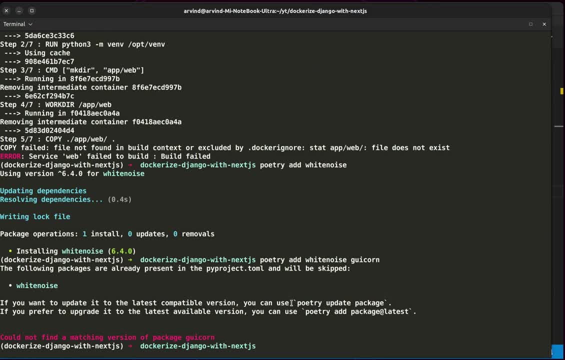 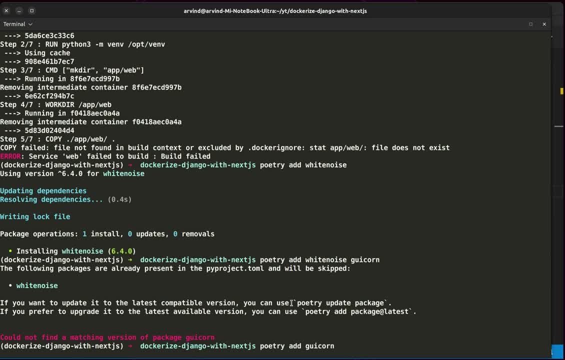 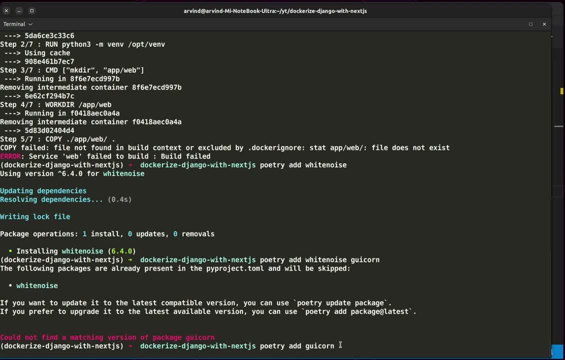 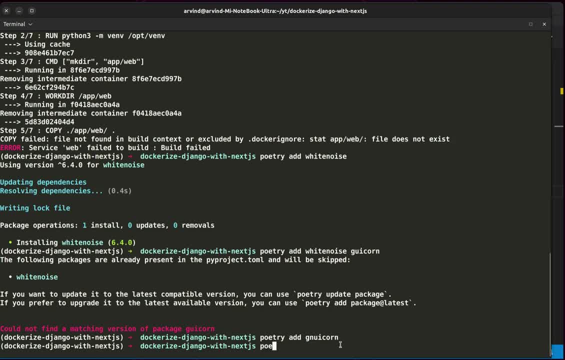 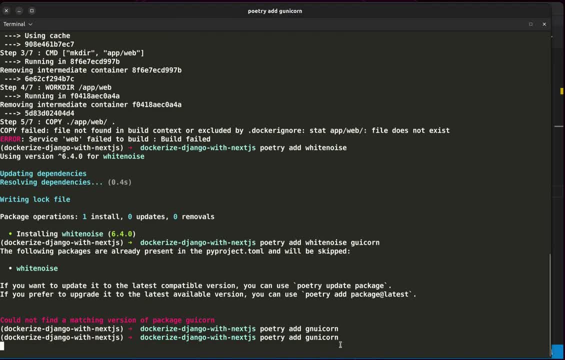 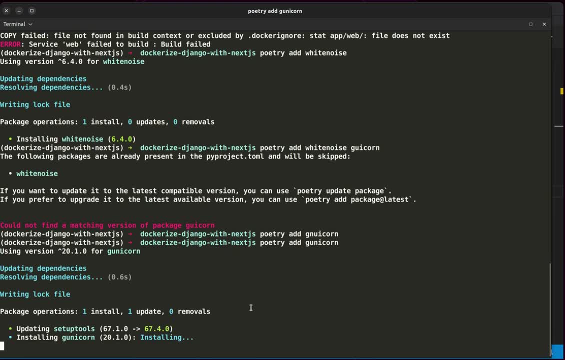 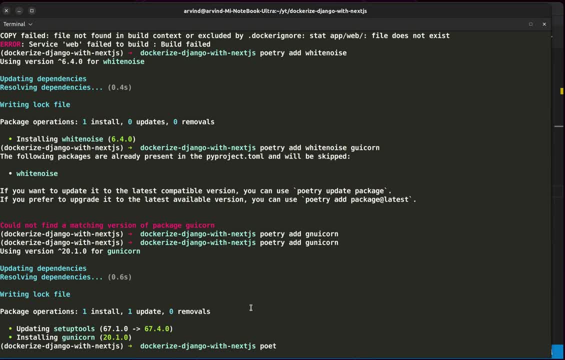 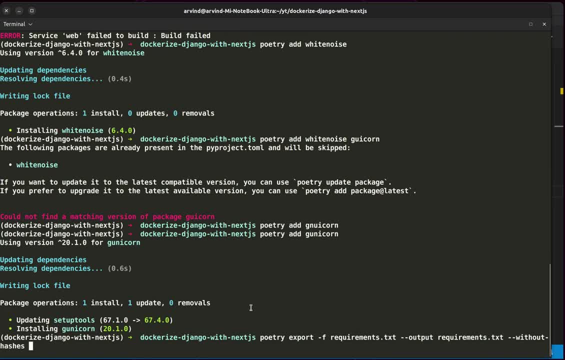 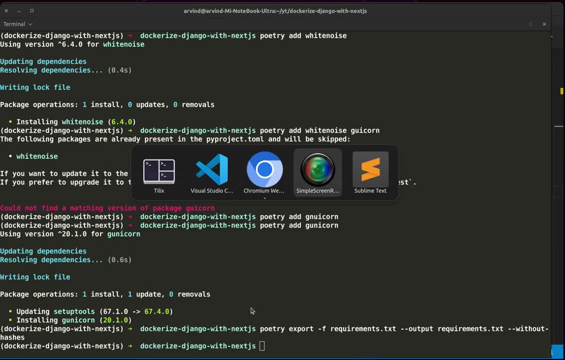 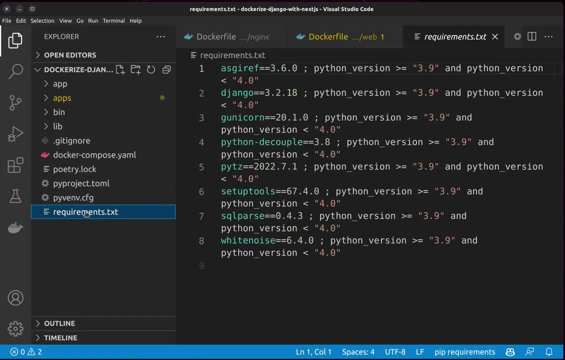 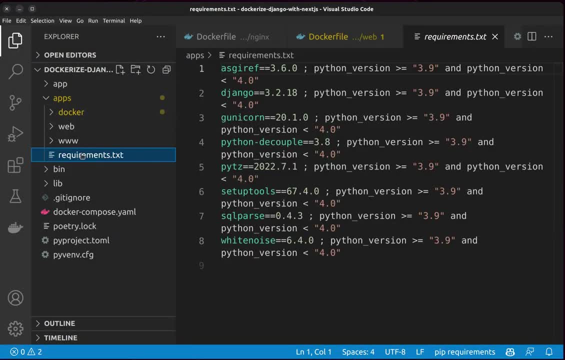 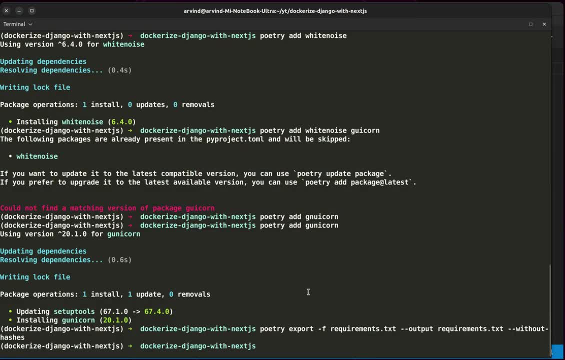 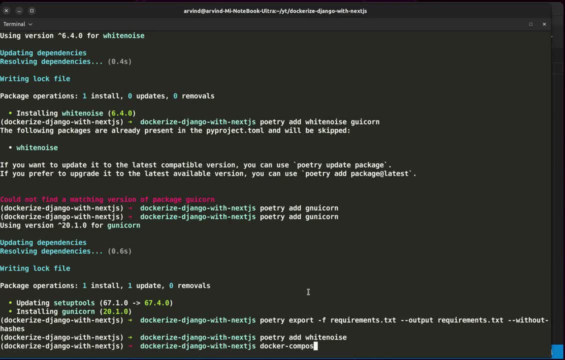 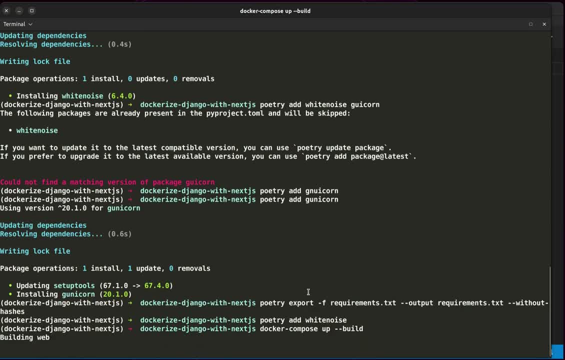 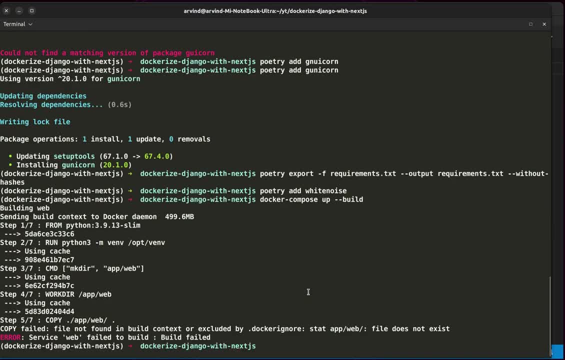 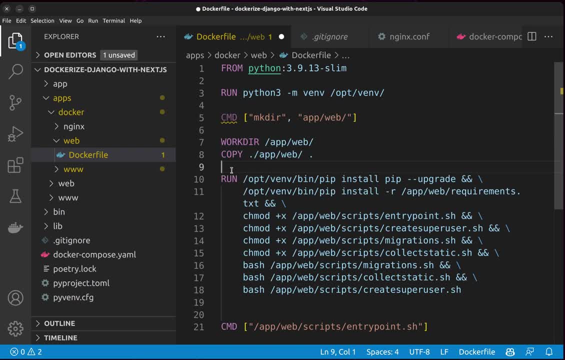 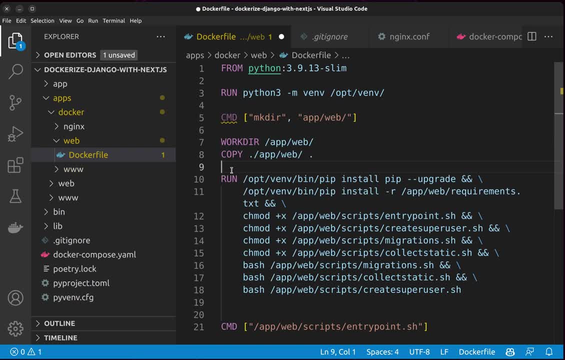 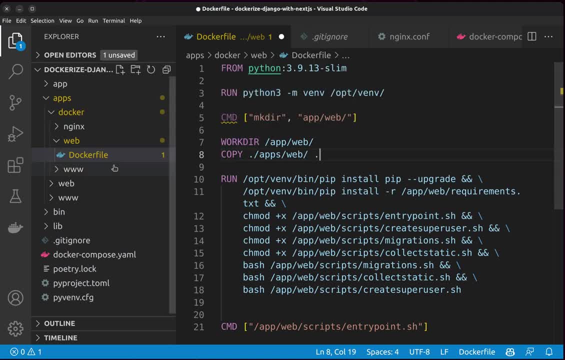 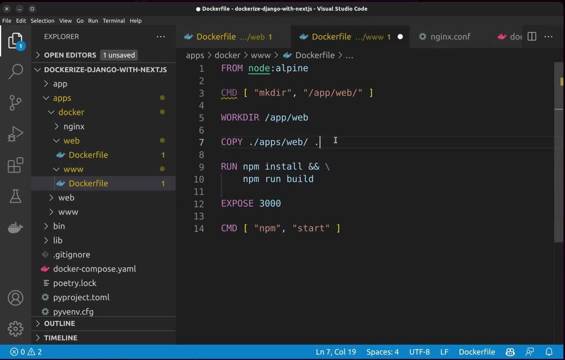 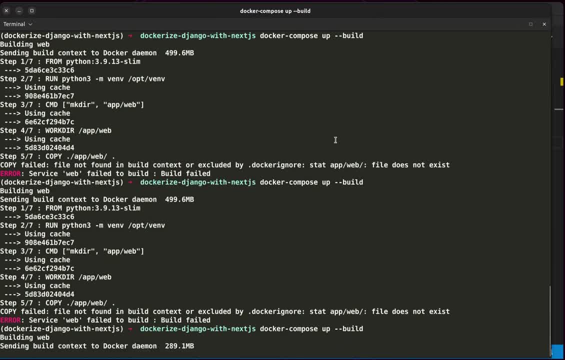 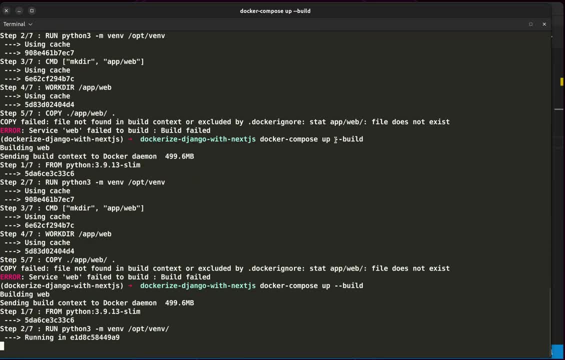 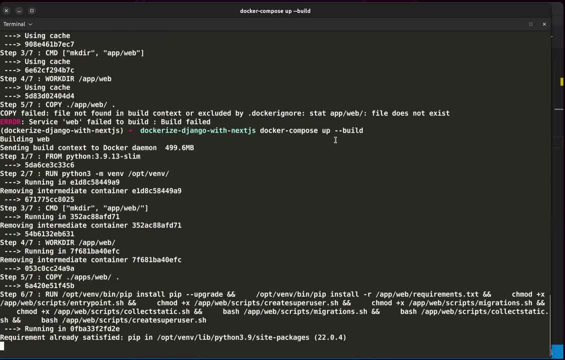 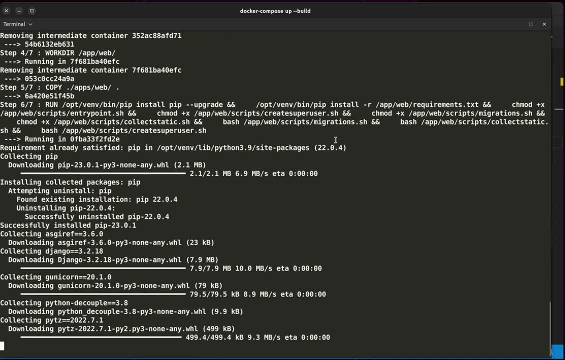 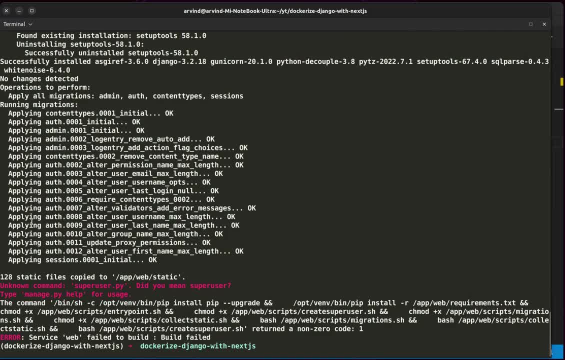 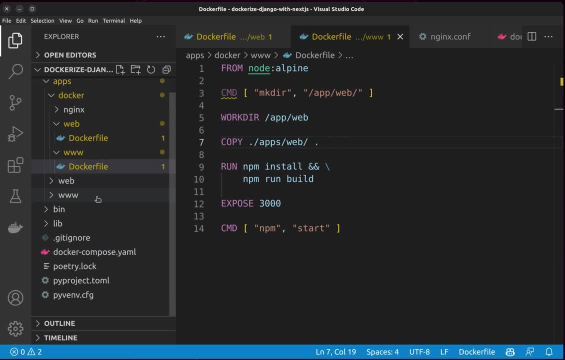 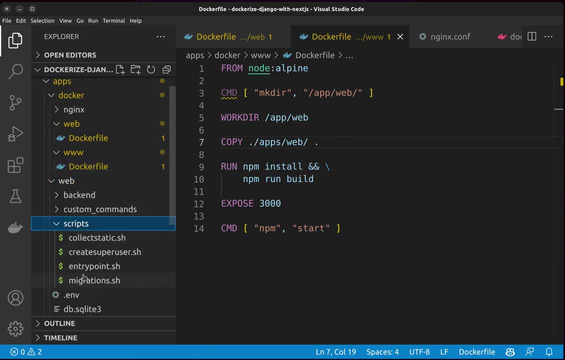 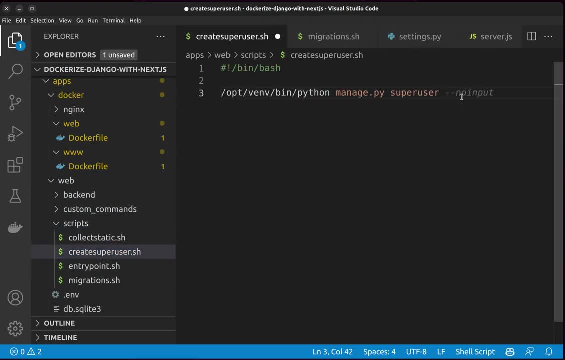 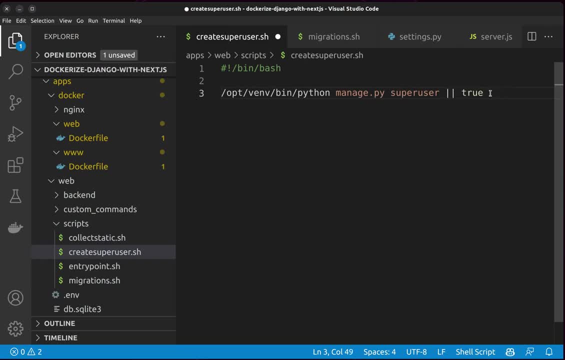 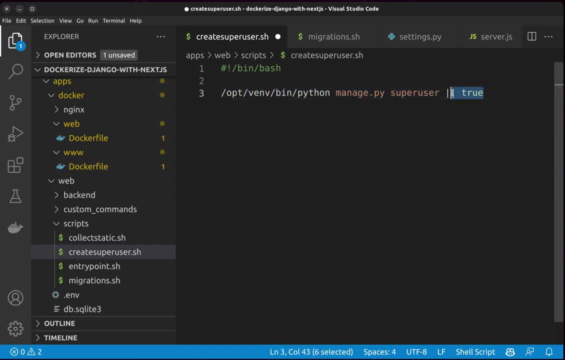 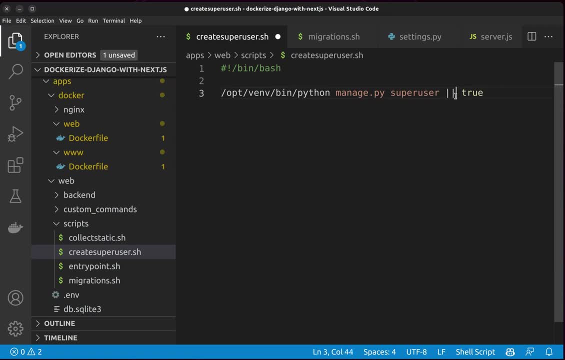 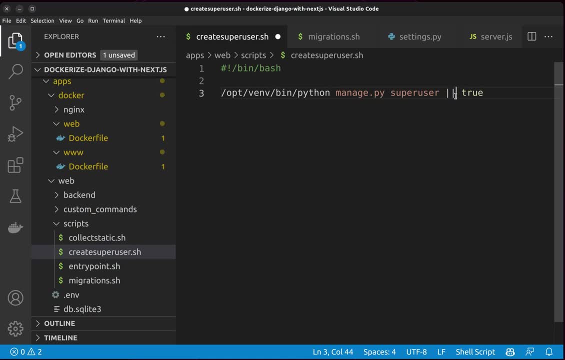 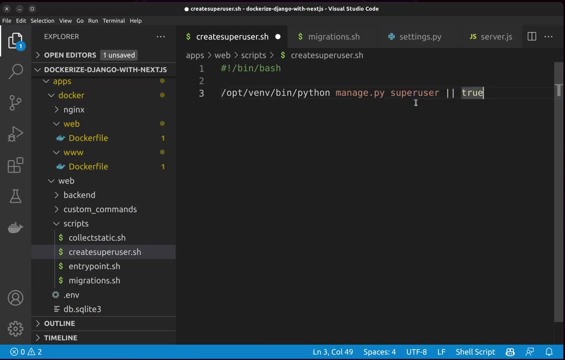 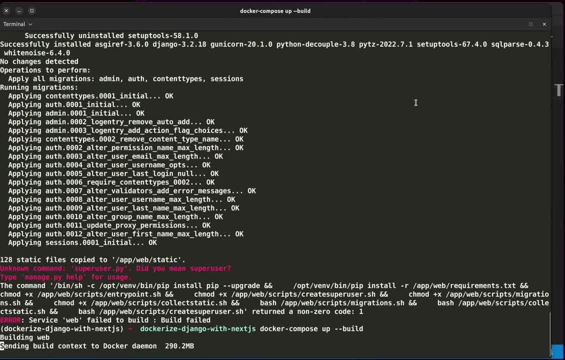 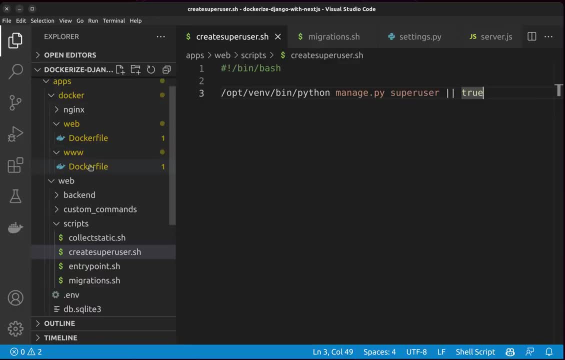 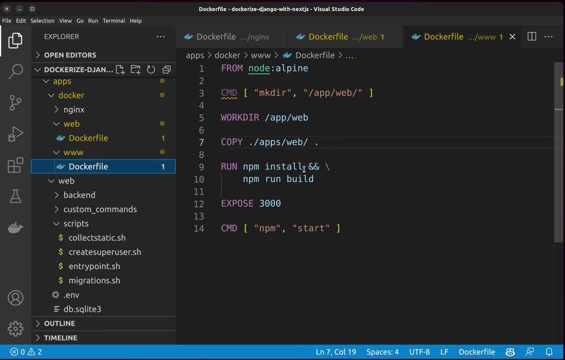 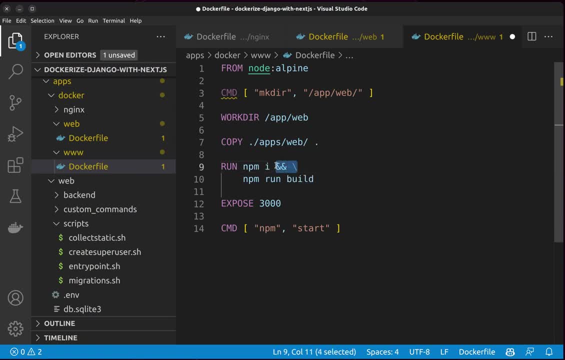 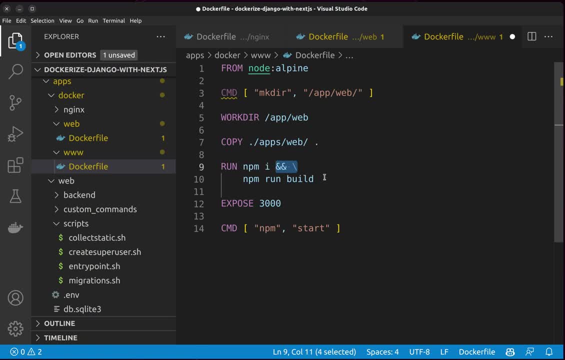 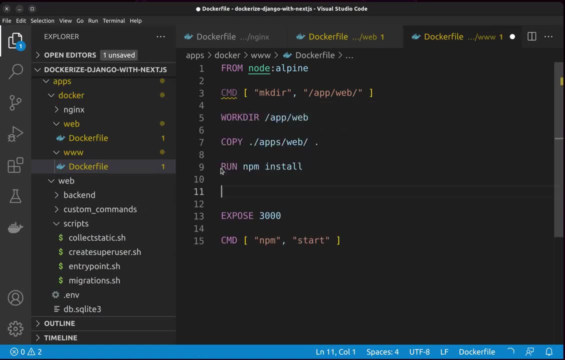 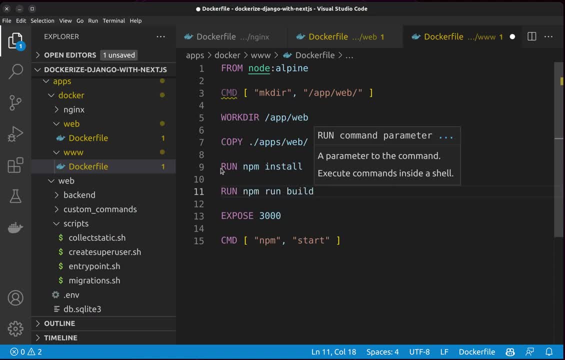 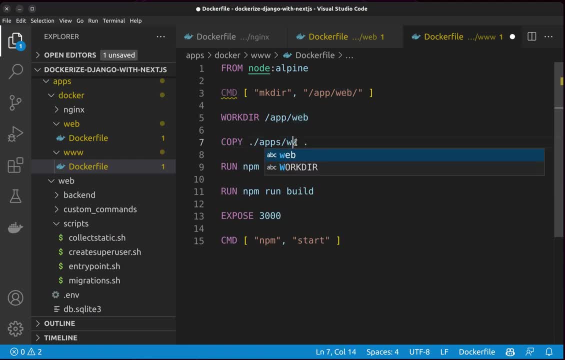 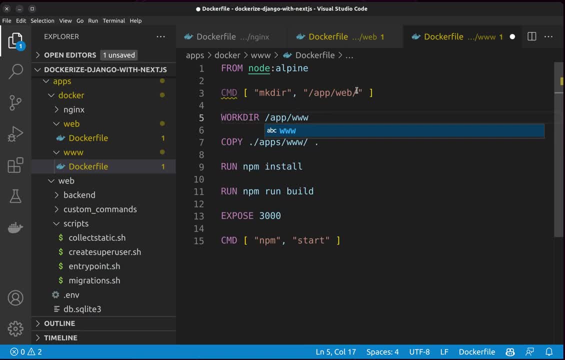 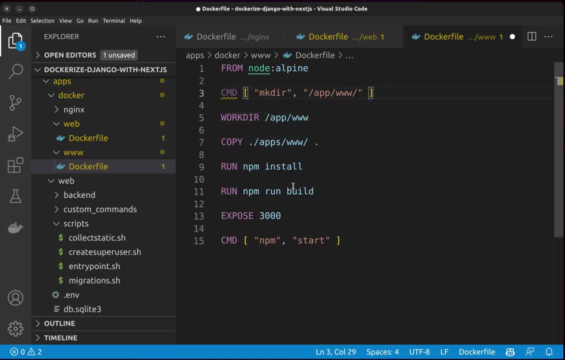 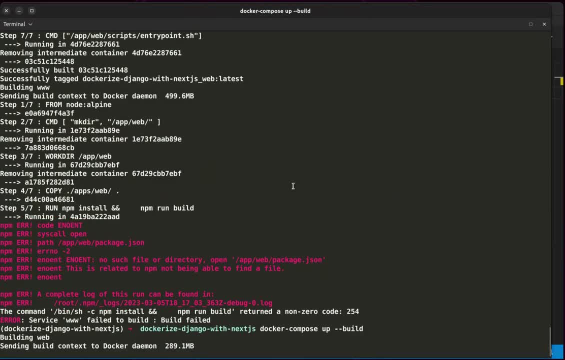 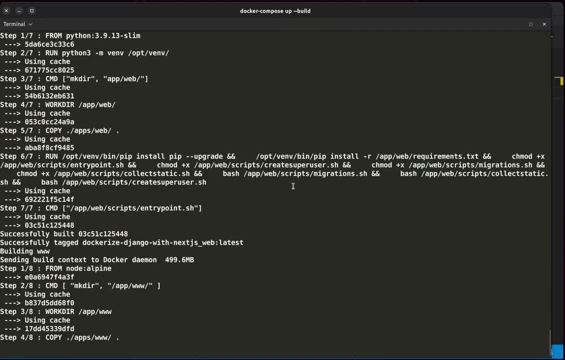 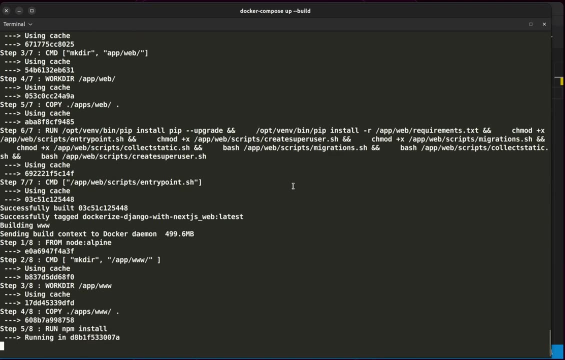 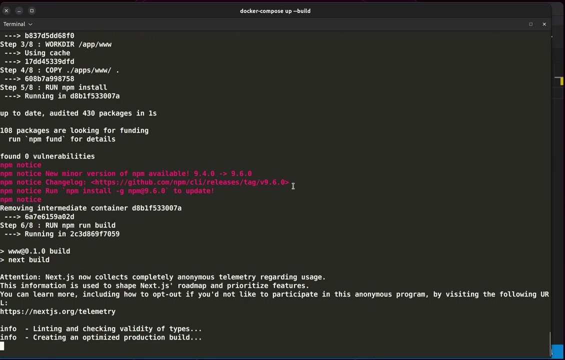 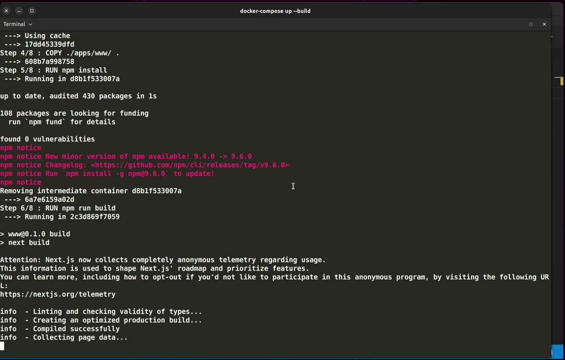 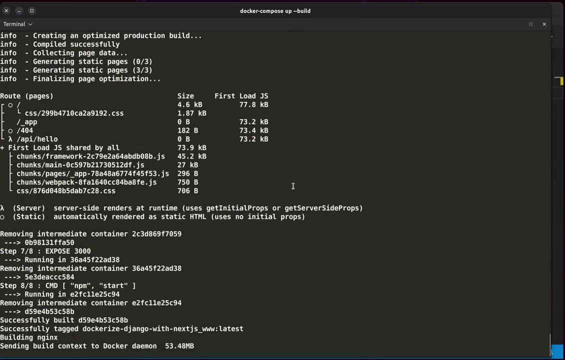 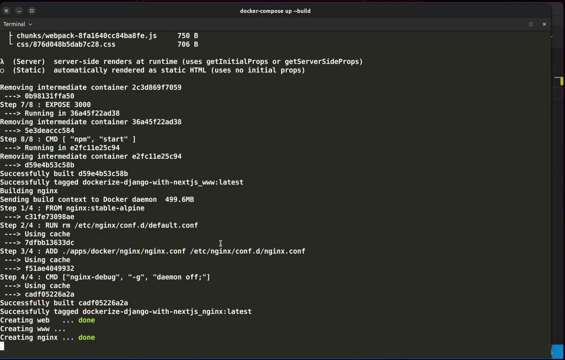 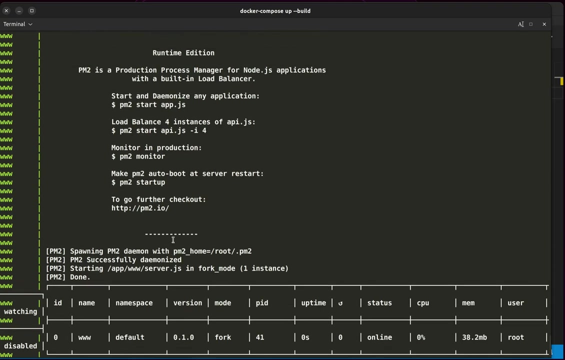 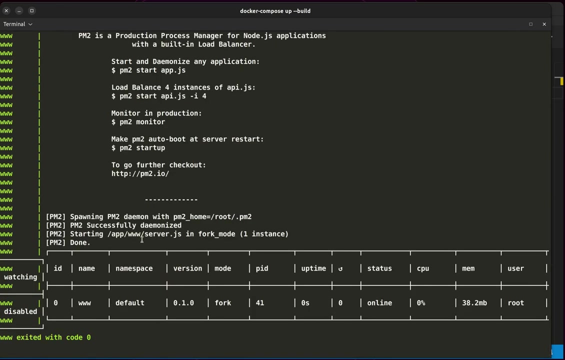 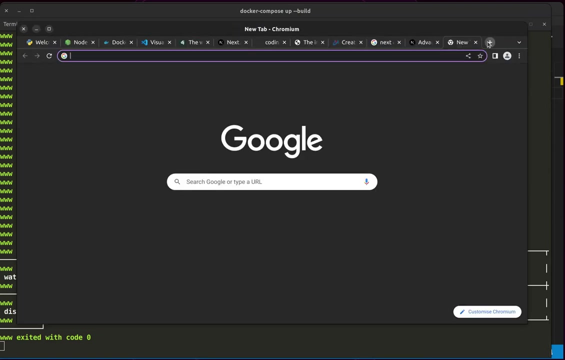 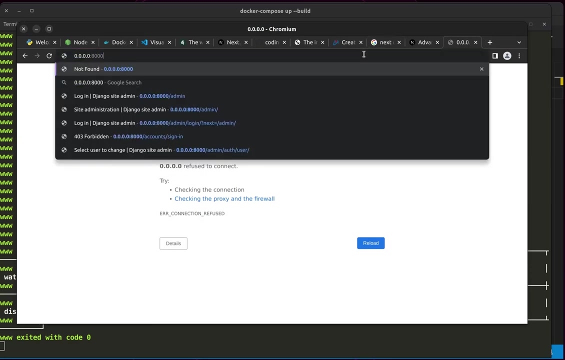 tmp dir. okay, so it's going to be a worker. tmp dir. okay, so it's going to be a worker. let's check for any errors on not Thank you. Okay, so my front end kind of failed, so let's go to. yeah, my front end is not running, but 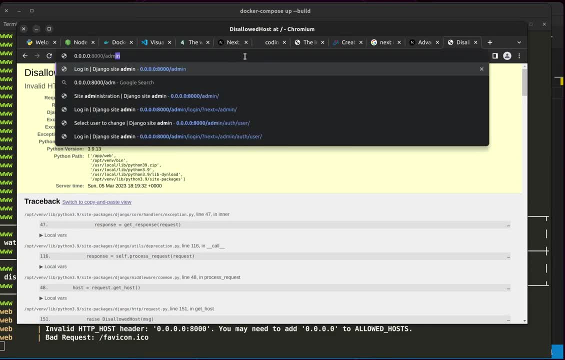 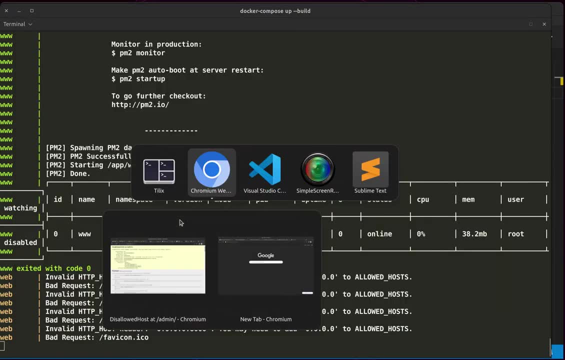 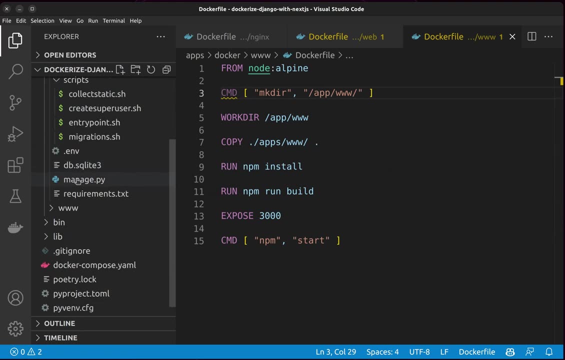 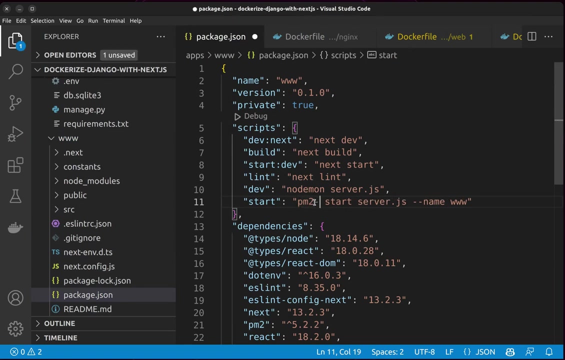 my? yeah, my back end is running. Yes, My back end is running, but my front end has failed. okay, so let's go to my. yeah, let's go to www, and then in packagejson it should be pm2 runtime. yeah, should be pm2, or else. 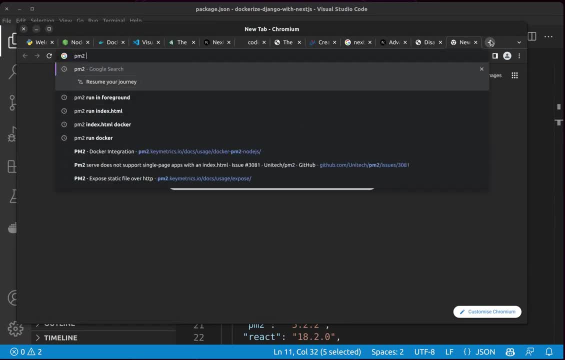 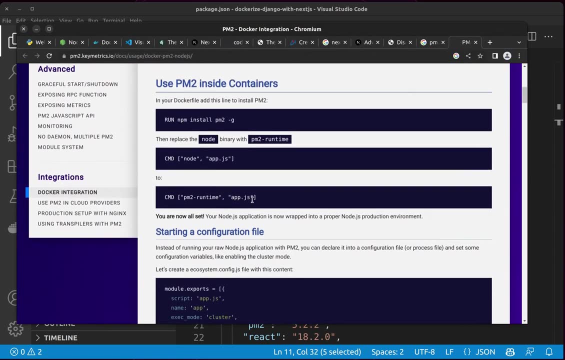 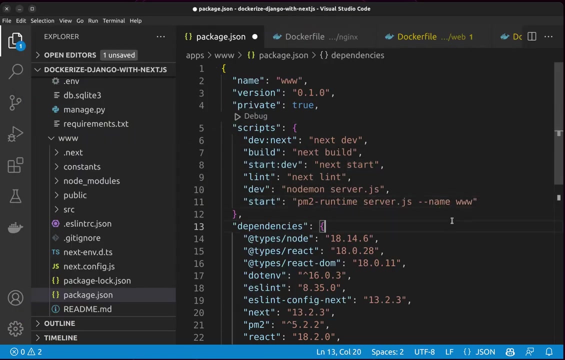 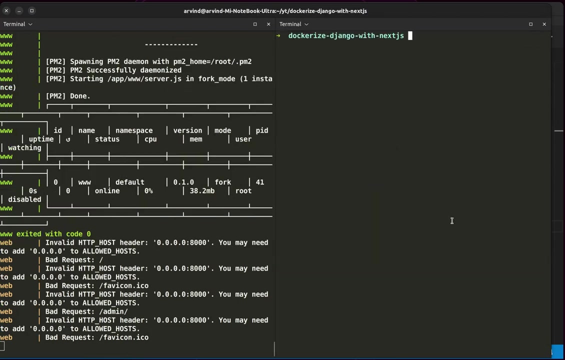 you can always google it. so pm2 runtime Docker, and then I see a docker integration and then it says pm2appjs, that's all. so it should be pm2 runtime serverjs, and then this should solve the problem. maybe. so yeah. 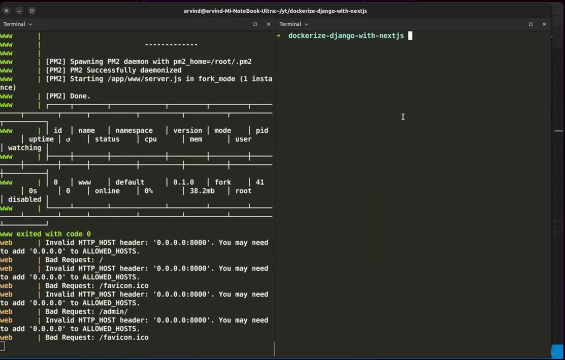 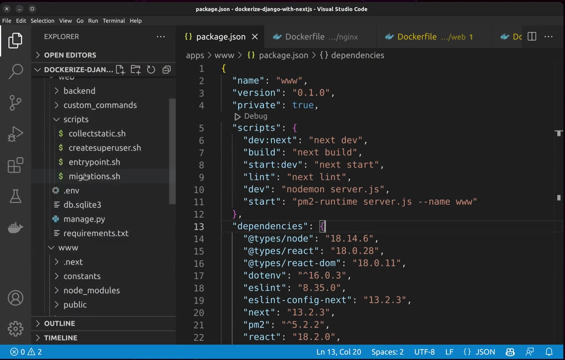 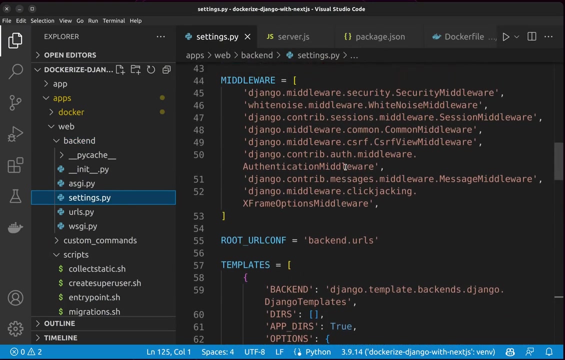 you can either press ctrl c, 2, 3 times or you can hit docker, compose down. Here we go Docker, compose down. Now the next step is: you want to do some tests? so what I'm going to do is I'm gonna go to my my python backend. 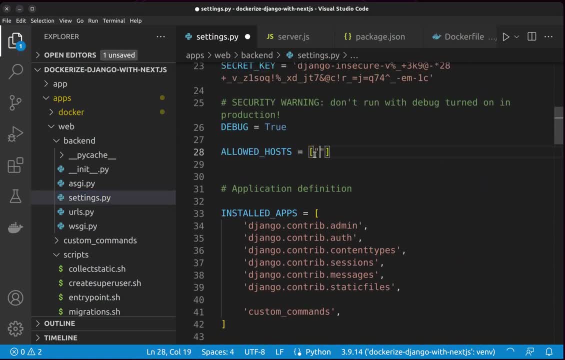 yeah, backend settingspy and I'm going to. yeah, allow hosts to star and now set my Django debug to false. Yeah, you can keep it as an environment variable and do, But as of now not available. 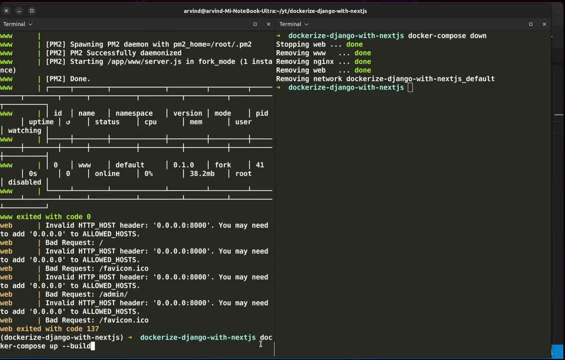 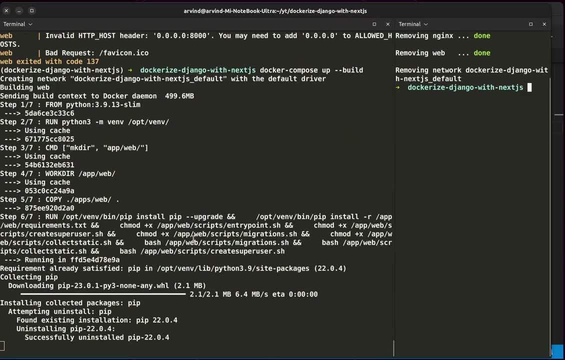 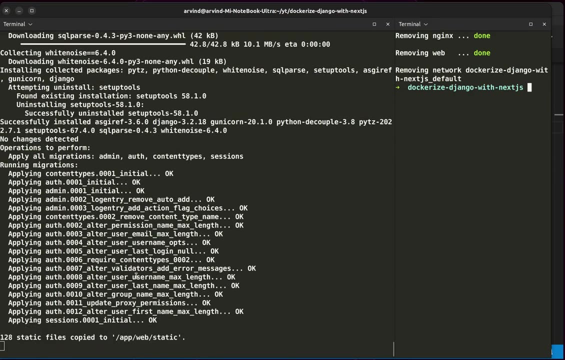 So you need to put the environment variable. So I'm gonna have to do this. I'm not going to do that, yeah, so let it build it. and yeah, I think everything is working perfectly, so at this time, everything should run okay. so once it's. 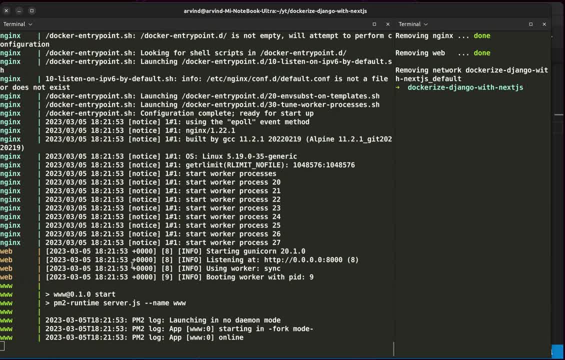 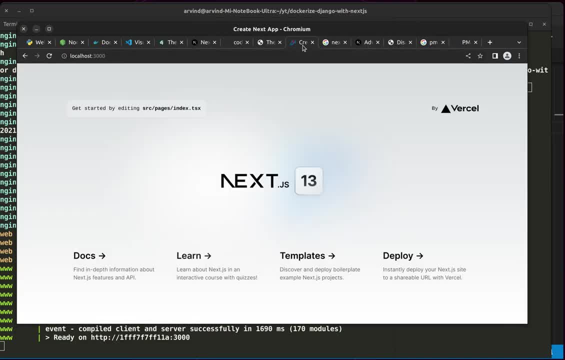 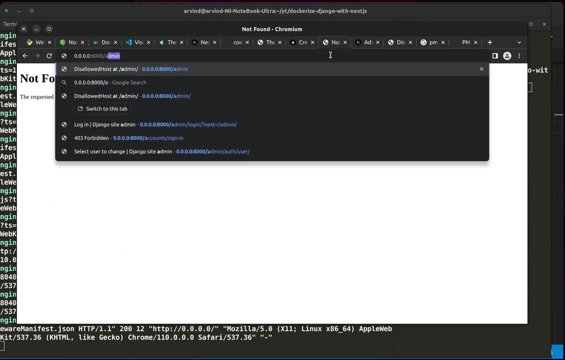 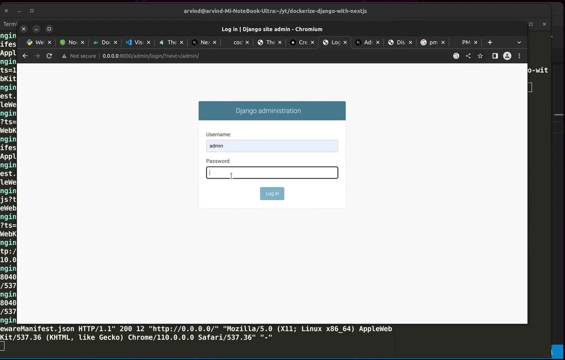 done. I'll get back to you, okay. so everything is kind of working perfectly, so this is the time to check what's happening, so I'll go to: yeah, my front-end is working now and now. yeah, admin, okay so, and now I created an admin with password one, two, three, four. 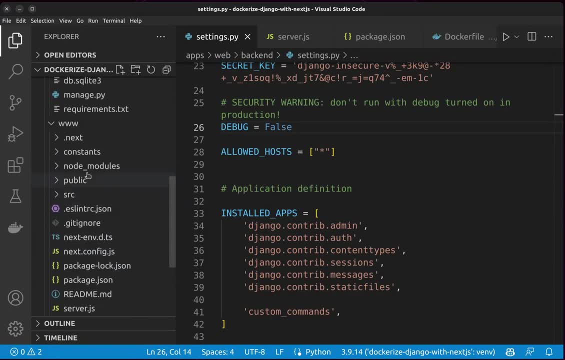 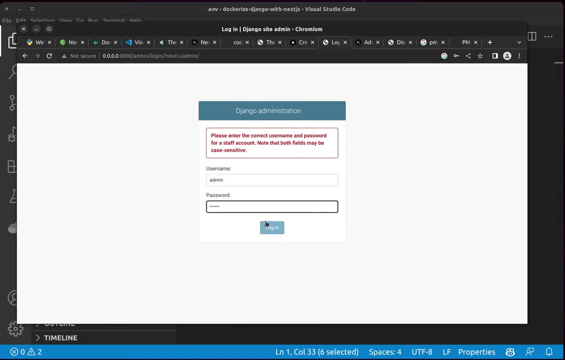 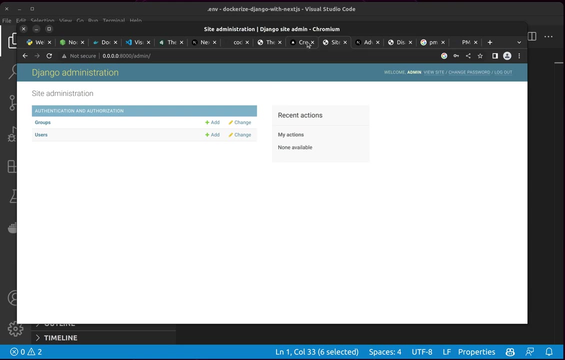 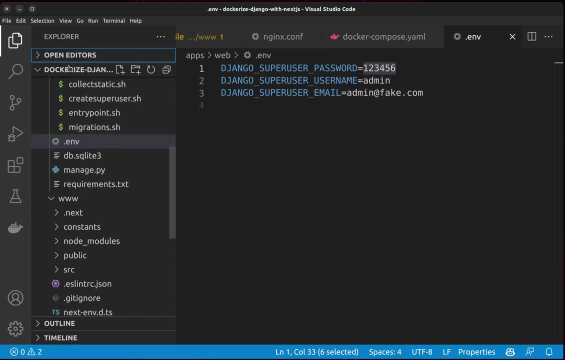 okay, I don't know what password I kept, so just okay. so it's one, two, three, four, five, six, admin, and now, yes, my super user is created, I can access my Django admin, and then my front-end is served using nginx. and so, yeah, this is what we have. 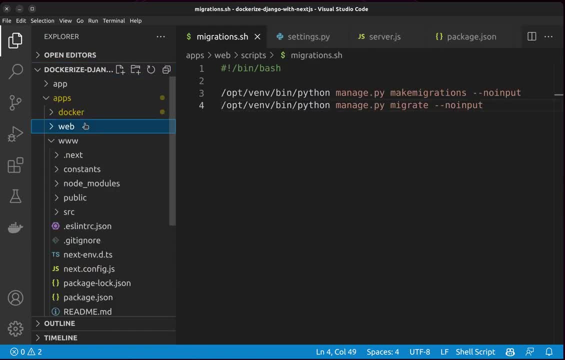 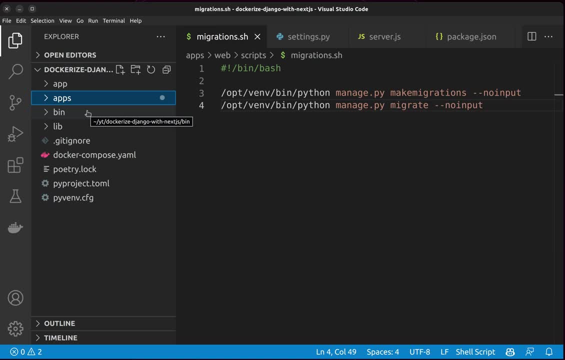 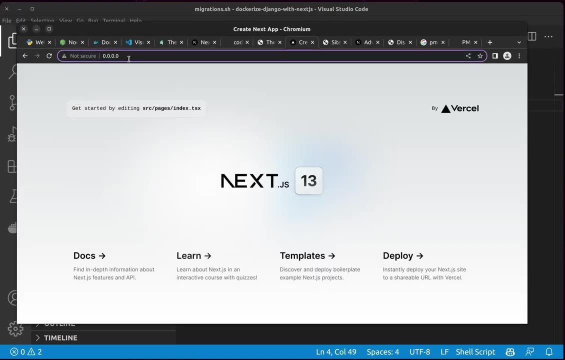 not done as configuring? yeah, configuring HTTPS. yeah, because as of not done as configuring, yeah, configuring HTTPS. yeah, because as of now it's, it's running in HTTP, so if you're going to production, you can use HTTPS. and then we didn't do like deploying it into an AWS or GCP and next. 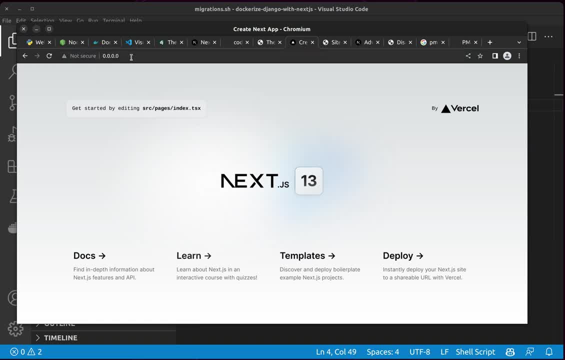 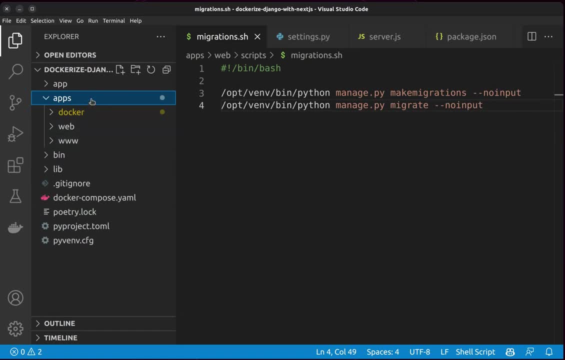 one is configuring domains, so only those three is left and those see if, if you are able to do till this much, are able to do till this much, then it's pretty much easier. all those, then it's pretty much easier. all those, then it's pretty much easier. all those, those are just small, small way across. 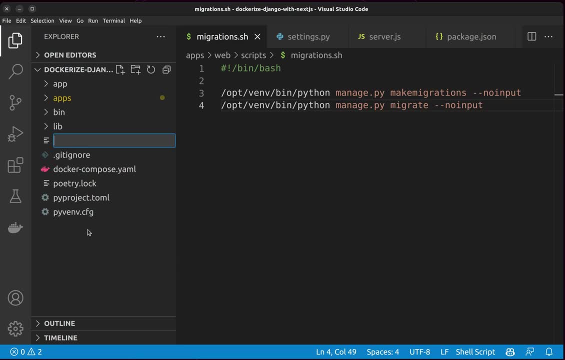 those are just small, small way across. those are just small, small way across. yeah, and now a pro tip. you can also. yeah and now a pro tip. you can also. yeah and now a pro tip. you can also create a dot docker- ignore docker- IGN for. create a dot docker- ignore docker- IGN for.